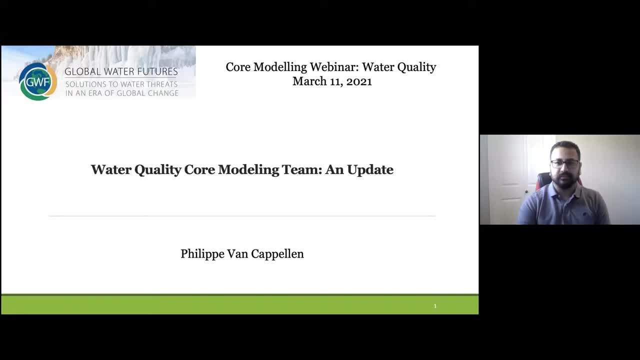 Philip, the floor is yours. Thank you, Parveen. So before we get started, I'd like to first acknowledge that I'm speaking to you from the traditional territory of the neutral Manishinabeg and Haudenosaunee people. 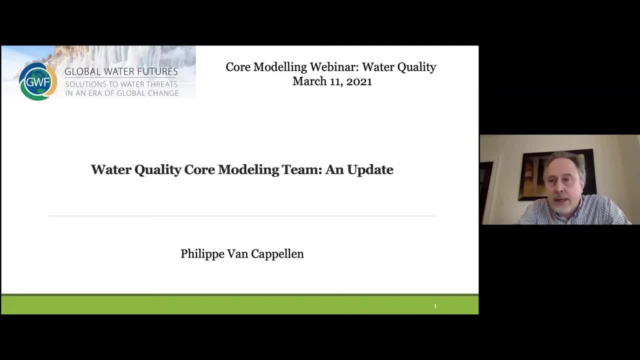 and I am talking to you from my home, which is situated on the Haldimand Track. That's the land that was promised to the Six Nations of the Grand River, So I'd like everybody to take a moment and acknowledge and appreciate the enduring role of Indigenous peoples as 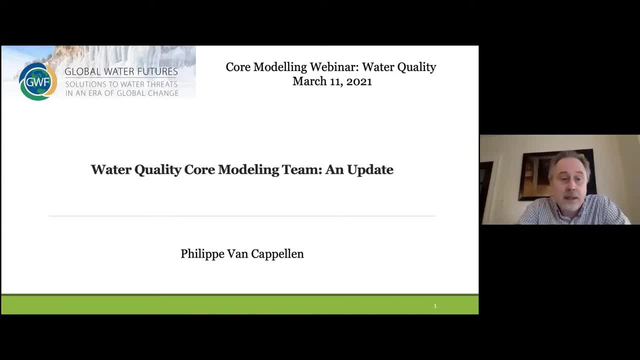 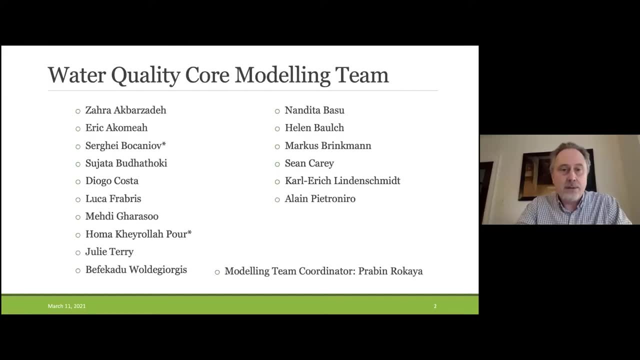 stewards of the river- Thank you very much, Parveen, Thank you very much, Thank you very- of our shared land and water and, on this occasion in particular, also as stewards of the quality of our water resources. so let me first start by introducing the water quality core modeling team. 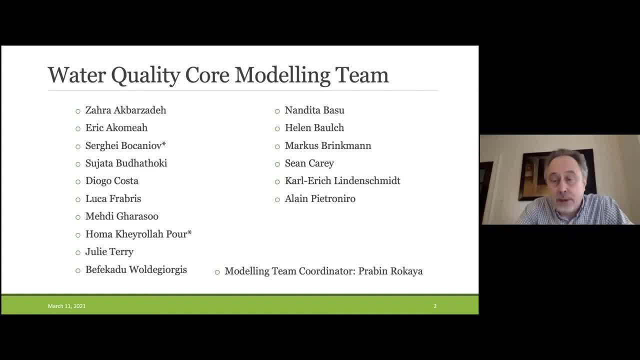 so on the left hand side, the list is the list of the current and two former uh postdoctoral fellows and associate researchers that formed the core modeling, the water quality core modeling team. so we have zara eric, sergey suyata, yogo luka, medhi homa, julie and bishikadu. 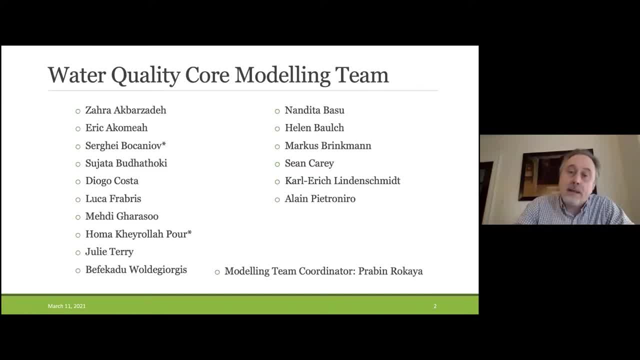 and the stars for sergey and homa indicate that they're no longer uh former. they're no longer formerly member of the water quality core modeling. they now have uh different appointments uh, but they're actually continuing the same work that they did when they were uh part of the water. 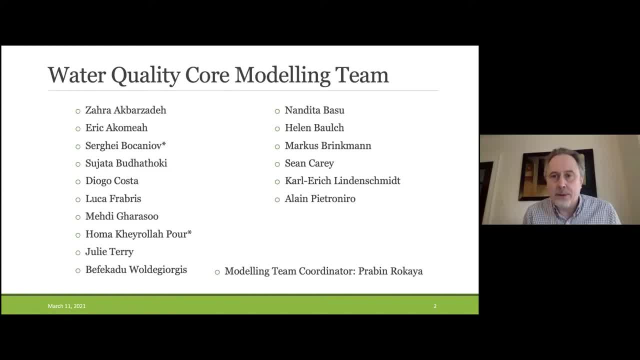 quality core modeling and i'll show some of their research results. also, on the right hand side you see some of the uh more senior people that are acting as supervisors or are closely involved with the activities of the water quality core modeling, and i also would like to acknowledge, of course, prabin, who has 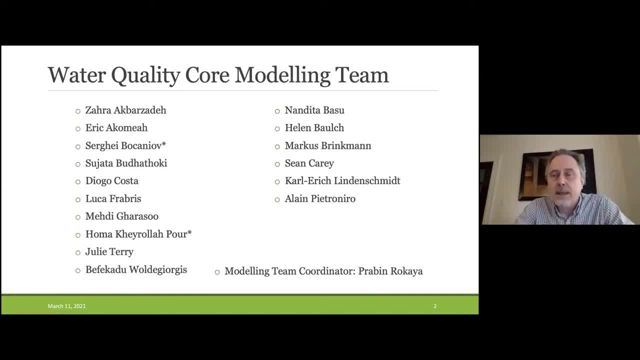 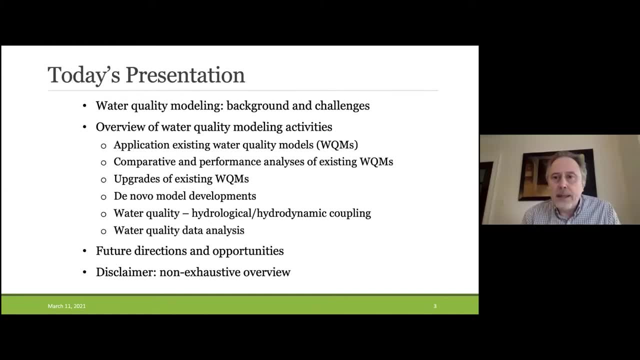 been helping with the logistics of coordinating the different meetings and keeping track of also the progress of the uh, of the team as a whole. so what i'd like to do today is to, um, to maybe start off with a little bit of a background uh on water quality modeling, so kind. 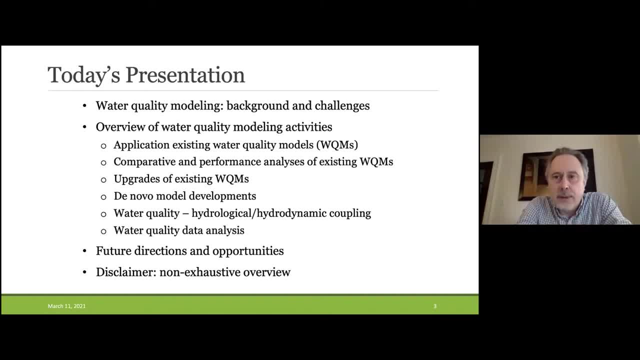 of what are the kind of the general challenges that we have when we want to model water quality of freshwater systems, and then i'll spend most of the time giving an overview of the water quality modeling activities within the team, so we'll see applications of existing water quality models. 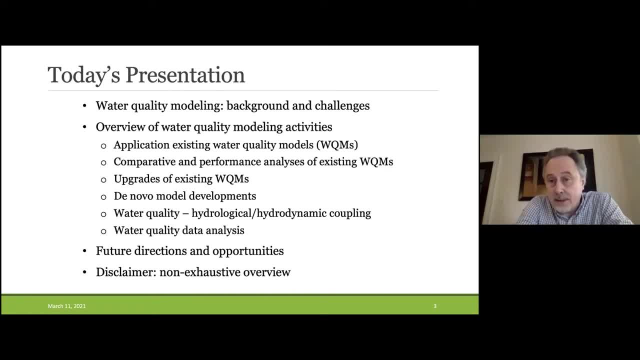 but also comparative and performing analysis of these existing models. that sometimes- and i'll show you at least one example where this actually leads to uh upgrading uh an existing water quality model, there will also be entirely new model developments. obviously, a big topic in in the team is: how do you essentially couple water quality calculations with hydrological and 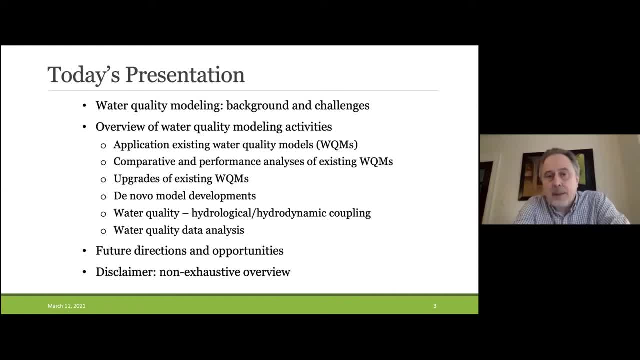 hydrodynamic simulations, and i'll speak a little bit about water quality data analysis, and i'll finish by giving at least a personal view of what some of the future directions and opportunities are. uh, within this, uh within this field, but also particularly uh as a. it relates to the core modeling team. uh, i want to also provide you with a disclaimer. uh, what? 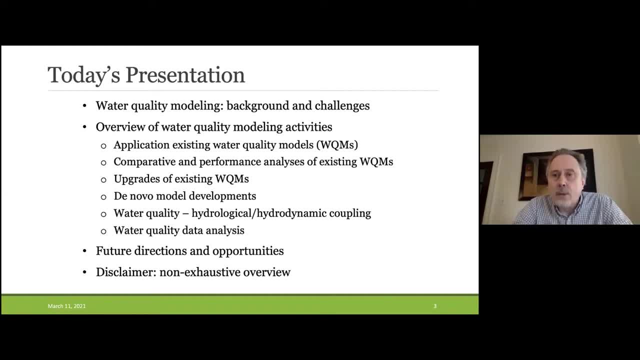 i will be presenting is not an exhaustive overview of all the water quality modeling work within uh- global water futures. there's other projects that are not directly supported by the, by this team, but that are doing, uh, some very exciting, some very new water quality modeling and even within 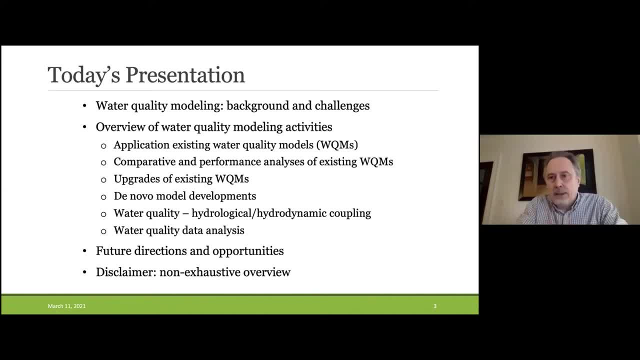 what is going on within the team. given the limited time, i will obviously skim over uh some of the the realizations or some of the activities, and so i apologize for that, but i hope at least that this overview will give you an idea of the capacity that's available in water quality. 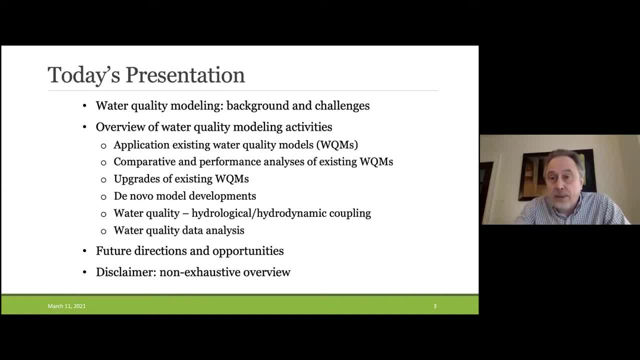 modeling within the team, and you should feel free, as a gwf researcher, to reach out to to our team for support in your- in your own research. i hope that at least this update will also allow us to stimulate that type of discussion, and so, when i present different projects, on each of the slides you will see the name of the. 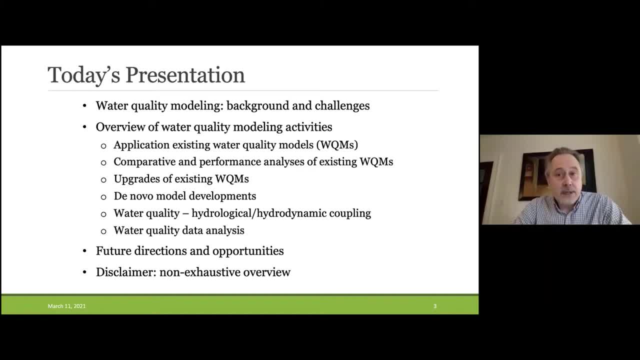 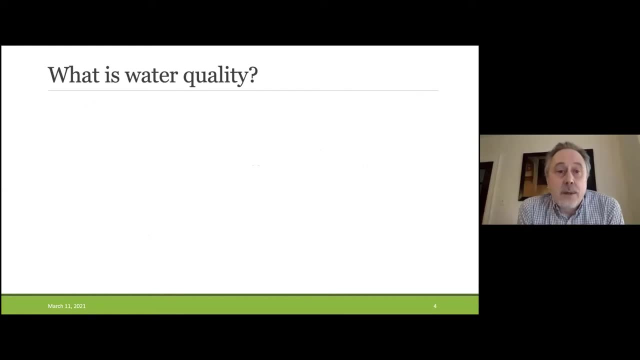 person who is doing that work, and so feel free to reach out to that person, or you can also reach out to me or to prabin to help you direct to that particular expertise that you might require new research. but let me first start by essentially asking the question: what is water quality and 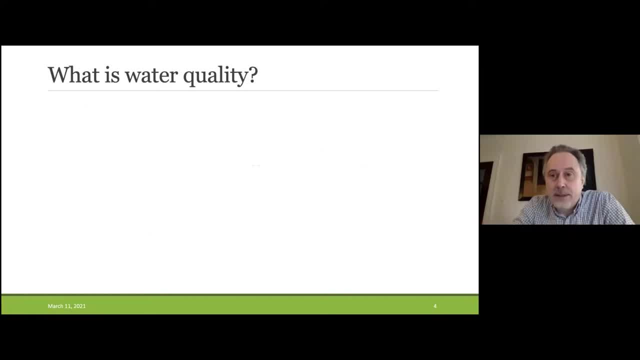 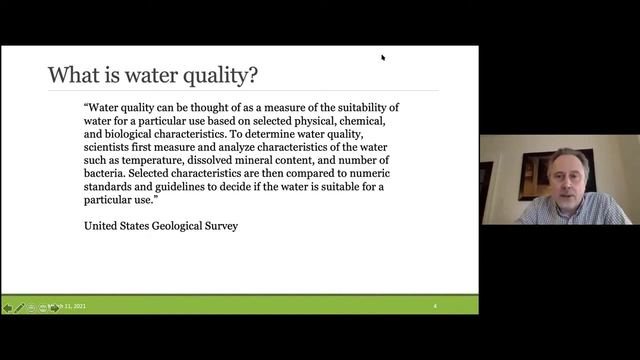 maybe i should have done this as a poll and ask all the participants here: what do you, how would you define water quality? and, of course, there is not a unique definition of water quality, and so here, for instance, is one that is from the uh, from the uh, united states geological survey, from usgs it. 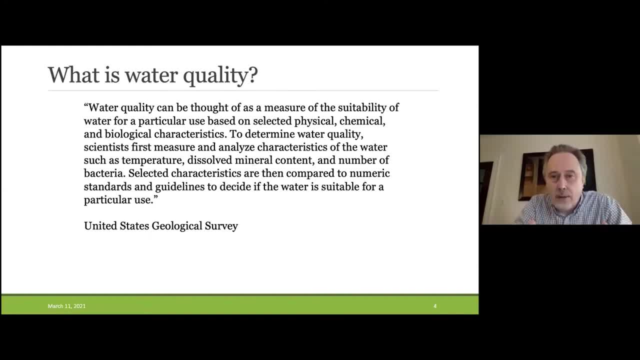 says, water quality can be thought of as a measure of the suitability of water for a particular use based on selected physical, chemical and biological characteristics. to determine water quality, scientists first measure and analyze characteristics of the water, such as temperature, dissolved mineral and number of bacteria. selected characteristics are then compared to numeric standards and 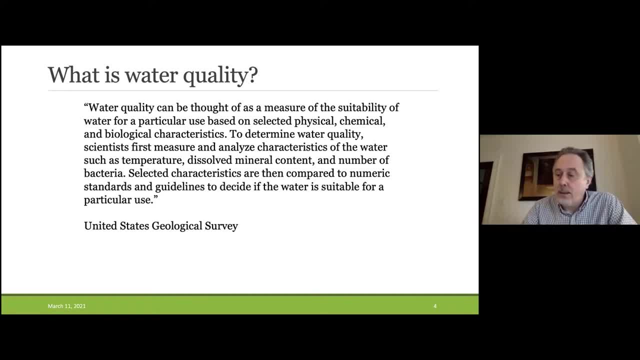 guidelines to decide if the water is suitable for a particular use. so you can see this is a very what i would call a utilitarian view of water quality. so it starts from the end use of the water and then defines what the appropriate water quality is. but you can still see that it's relatively to a 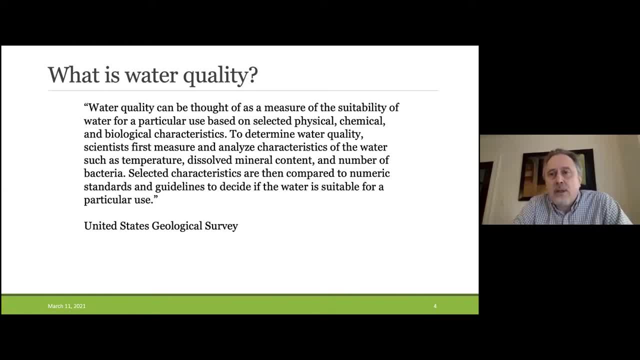 certain extent kind of vague, because it's it starts up and you can think of water quality as a measure of etc. so it's not as simple as saying, well, what is going to be the the water level in lake huron next year, given some hydrological predictions. so when you have to explain, or when i try to explain, water quality, 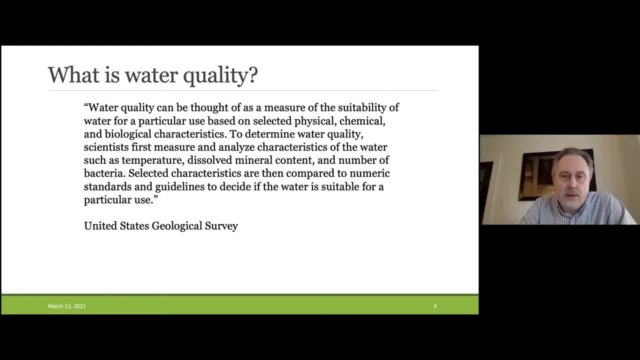 to maybe a more general public i use. what's often used nowadays is the trouble. moving forward here looks like my ah okay, so water quality is an attempt to keep the water swimmable, fishable and drinkable. so this is kind of more from the the human perspective i would say you can also. 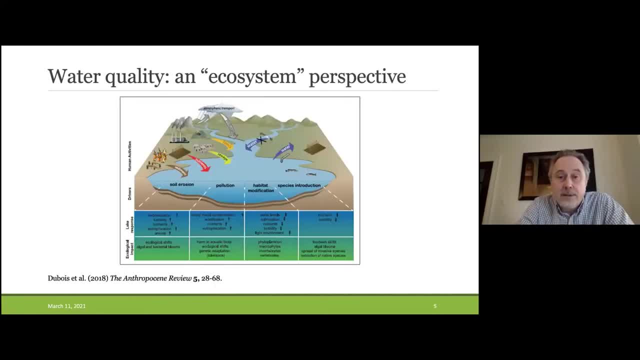 take a more ecological or ecosystem perspective. here, for instance, is a very nice diagram where you you look at the- if you can see my my point here- you look at the lake, you look at the various human activities in the watershed of the lake. uh, that leads to soil. 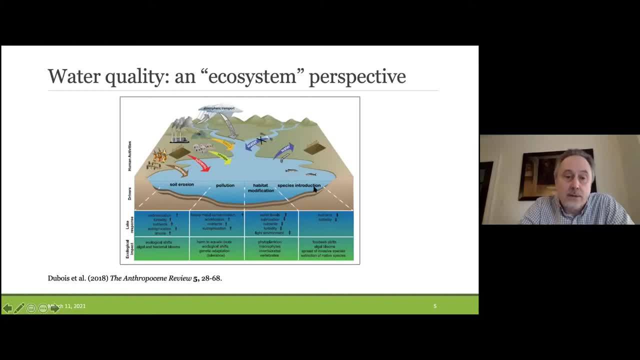 erosion, pollution, habitat modification, species introduction. then these drivers then have certain impacts or have responses of the lake, for instance, in terms of increasing turbidity or increasing nutrients, development of anoxia- which then lead to certain ecological impacts that might affect, for instance, the biodiversity- uh can cause all the blooms, etc. so what you see is that there's 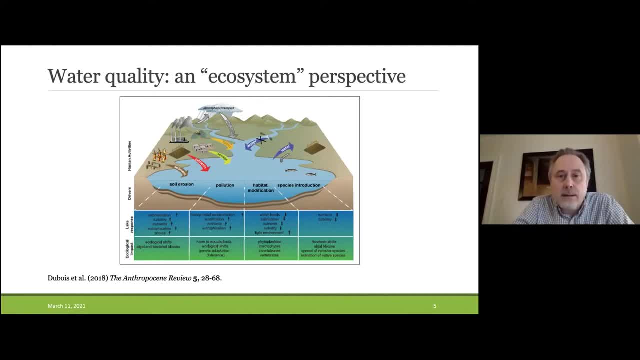 different perspectives on water quality, and so one way to then reconcile the human perspective or the societal perspective and ecosystem perspective is to concepts such as ecosystem services. so really start dealing dealing with water quality as a socio-ecological uh parameter. so then, how do we measure water? 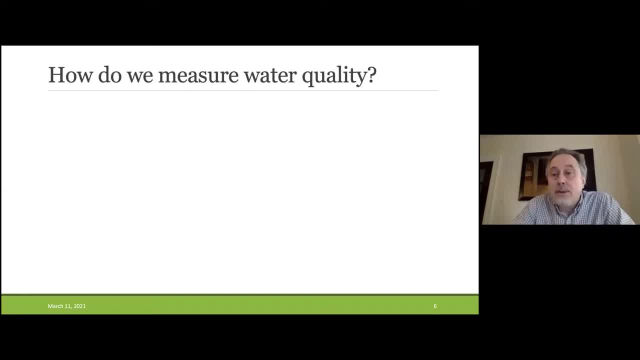 quality. again, it depends on who you are, what your interest is or for which agency you're working, or also what your, what your expertise is. and so you see the list of typical water quality measurements: temperature, salinity, turbidity, ph, major iron composition, things like hardness, biological oxygen demand. 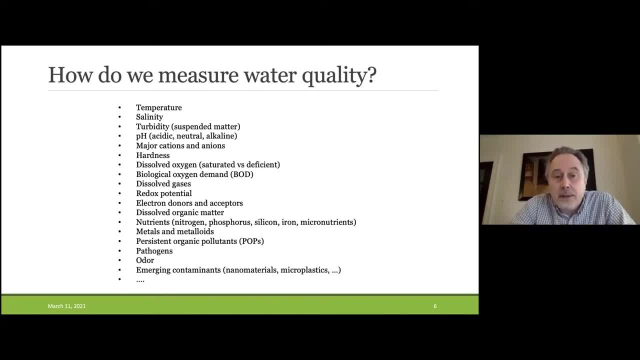 redox potential or defining redox conditions in terms of the availability of electron donors and acceptors, dissolved organic carbon, and the list goes on and on and on. and so that obviously also points to the problem of saying, well, we are water quality modelers, well, what kind of variables are? 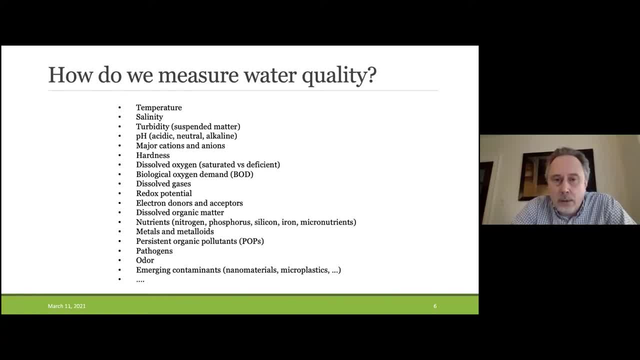 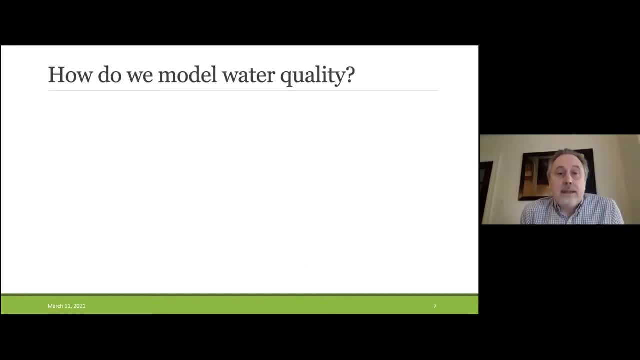 you considering, and obviously there's no water quality model in the world that will essentially simulate all these different, these different variables. now, at the very base, based on the theoretical basis of, i would say, essentially- most environmental models are so-called the conservation equations, so conservation of energy, of momentum and of mass. 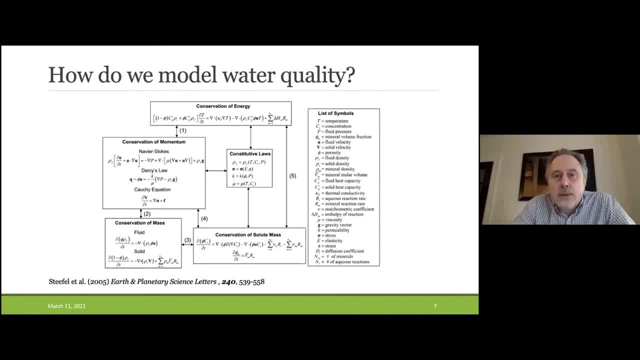 and when we're most of the project that you will see on that i'll present from the core team- deal with certain chemical characteristics, not always chemical characteristics, but also temperature: chemical characteristics of the, of the uh, of a water system, a hydro system, And so, for instance, if we talk about temperature, obviously we're talking about conservation of energy and all the processes that can produce or consume heat. 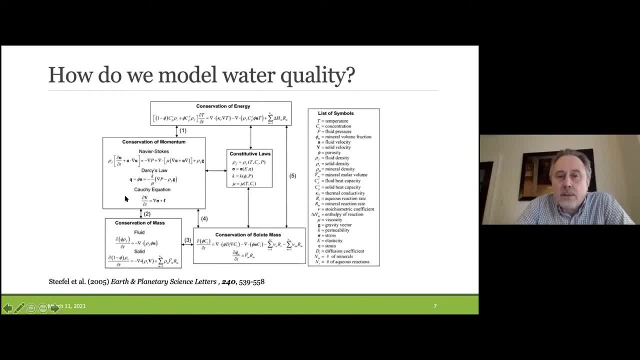 Obviously, we're dealing with hydrological systems, So we're involved. We are, of course, dependent on being able to say something about the flow of water through our system, whether it's a groundwater or surface water system, And so we have to consider conservation of momentum. 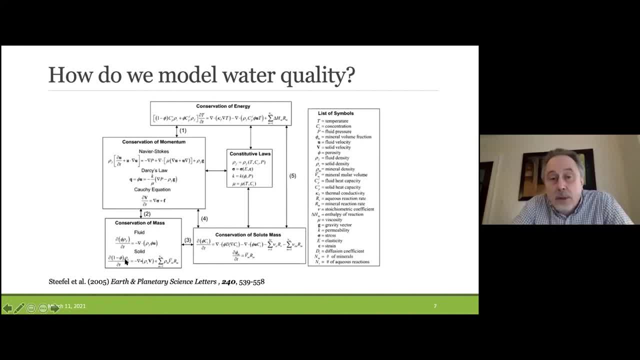 And then, if we're talking about a chemical constituent, then, or even a biological constituents, for instance bacterial numbers or pathogen numbers, we're dealing with the conservation of mass and in particular the equation, the conservation of solid mass. Here you see a bunch of terms here on the right hand side, that deal with the mixing and the transport of the constituent. 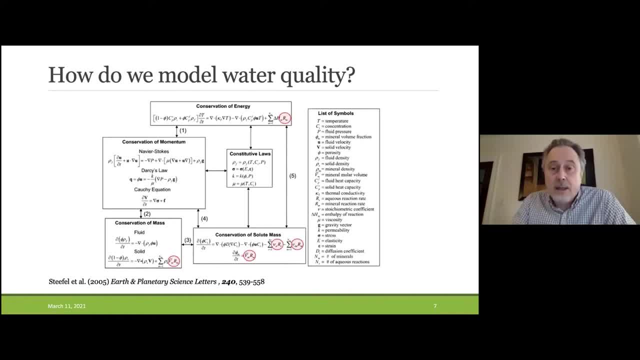 And then you have all these terms, these big R's, which actually reflect to the rates of processes That actually are affecting the constituent in the hydro system of interest. And so these big R's, these rates, are essentially one of the challenges in water quality modeling when we're dealing with reactive constituents. 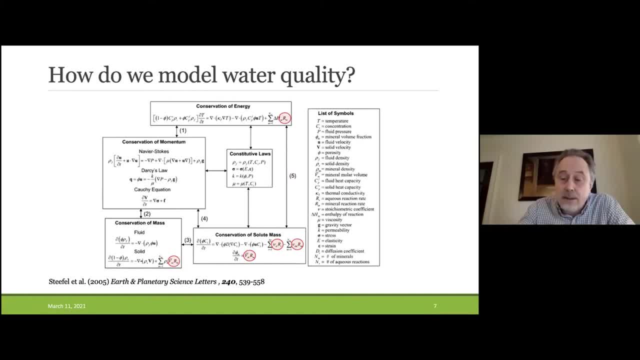 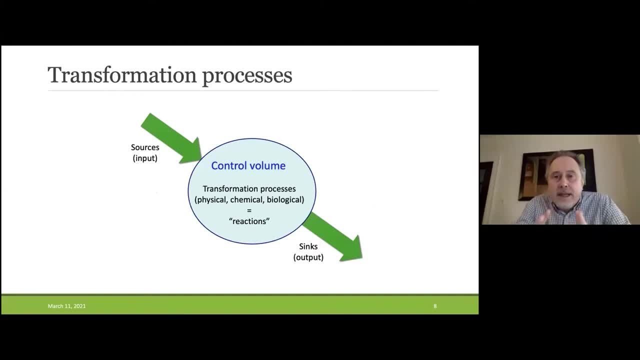 So constituents that actually can undergo transformations in the, in the system of interest. So, essentially, to go back to the modeling aspect, to be able to essentially account for the spatial and temporal, temporal distribution of a water quality parameter, whether it is temperature. 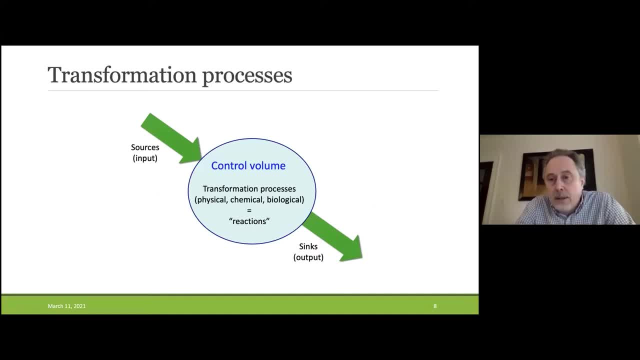 whether it is turbidity or whether it's a particular chemical constituent, say nitrogen or phosphorus. We need to obviously specify the sources to a particular system, account for the transformation processes in the system, And those could be physical, could be, for instance, a phase transition. 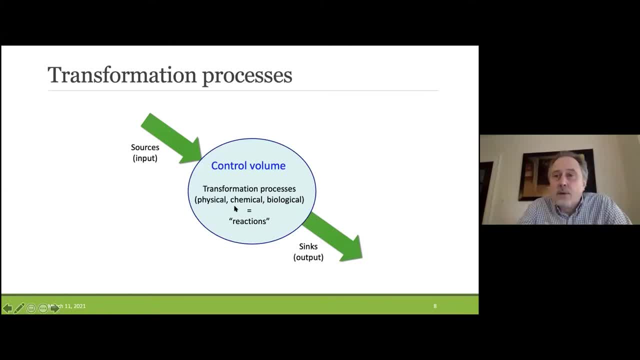 It could be chemical processes, say sorption, desorption processes or mineral formation. They could be biological processes- uptake of a nutrient, for instance biology- or mineralization processes, And then the sinks and the outputs could be towards the, for instance. 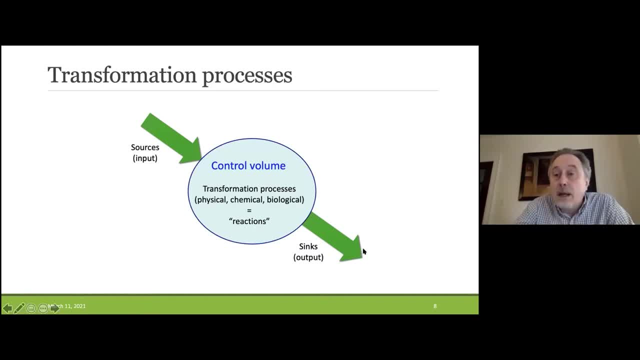 if we're looking at a river, the sink could be the outflow to a lake, But, for instance, nitrogen also be denitrification and the release of gaseous nitrogen to the atmosphere. So, in terms of looking at these transformation processes, 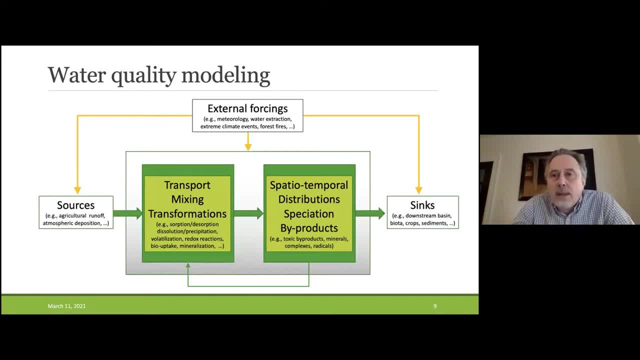 this is kind of the general scheme, then, for a water quality Modeling, where you account, of course, for the sources of whatever variable you're interested in it within the system, which is the big box here. you have to then account for, or you have to have a mathematical representation of the transport and mixing processes. 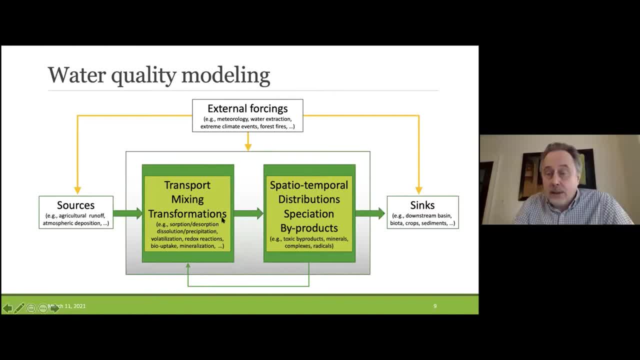 and then account for all the transformations if you're dealing with a reactive constituent, and reactive taken broadly, including also biological constituents of the system, And so I think Marked here a couple of these transformation processes, If you're able to come up with mathematical representations for endotransport. 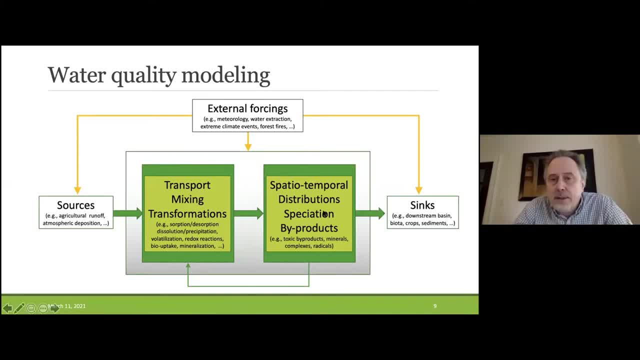 endotransformations. you should be able to then predict or simulate the spatial and temporal distributions, but also, particularly for reactive species. also account for the different forms under which, say, for instance, nitrogen occurs in a lake or in a river system. 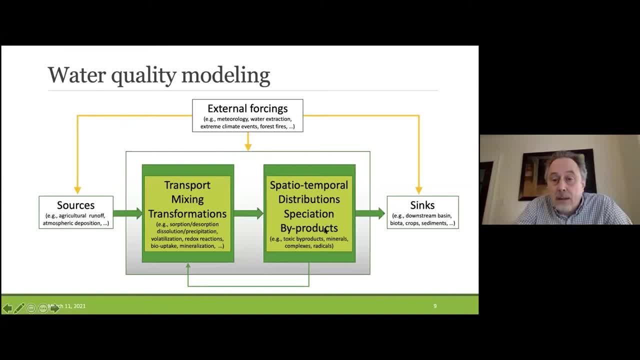 A lot of times, when we have these reactive constituents- and again let's think about nitrogen- you can actually produce byproducts. So, for instance, in the process of denitrification, nitrate ultimately is transformed into gas that then can be gas to the, to the atmosphere. 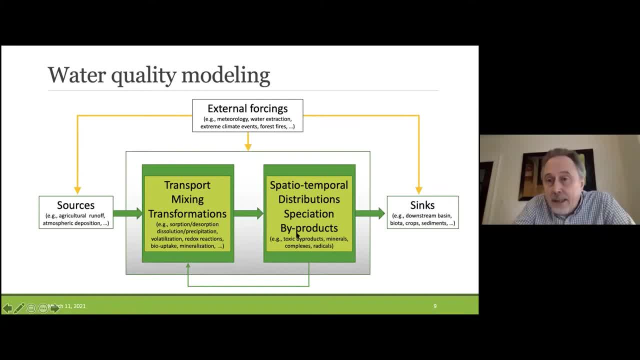 But you also produce byproducts, such for instance as nitrite and nitrous oxide, And these byproducts can also have an impact on water quality, And therefore you then also have to account for their transport and transformation processes, And then ultimately you have your sinks. 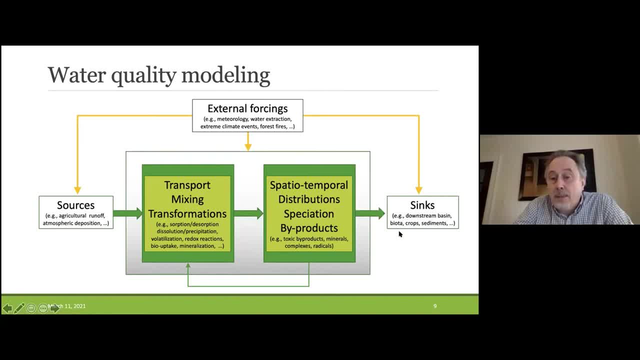 This could be a downstream basin, could be uptake by Bovota. If you're dealing with an agricultural system, it could be uptake of carbon and nutrients by crops. It could be essentially burial in sediments And, of course, both well, in fact, in your sources and your system and your sinks are then also subject to external forcings. 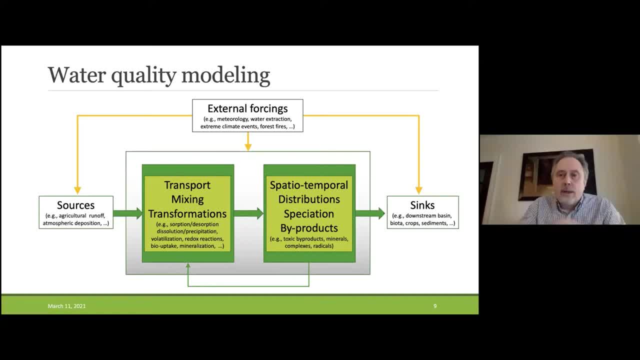 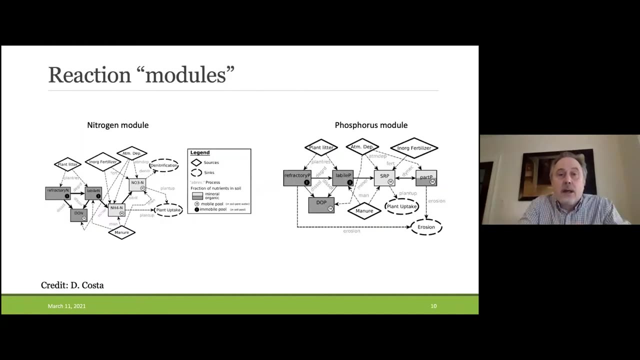 So this gives you kind of the overall scheme that we're working in, And of course, not a single person within the core modeling team does that. It does everything, But it kind of fits within this general framework. So when we talk about reactions, this is kind of a good way to represent them. 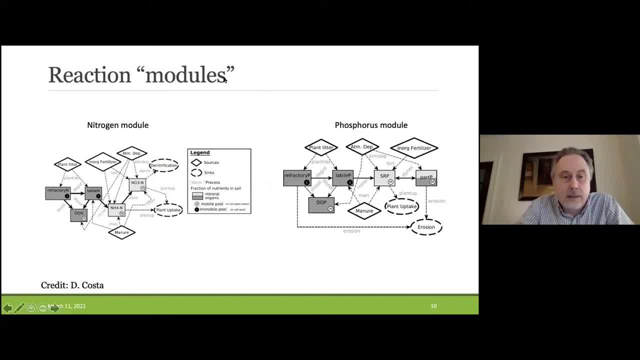 And it's from Diego. For instance, he's developed a nitrogen module and a phosphor module to represent processes in soils, in catchments, And it nicely shows with different symbols the sources. So for instance, if you look at the nitrogen module, you have fertilizer. 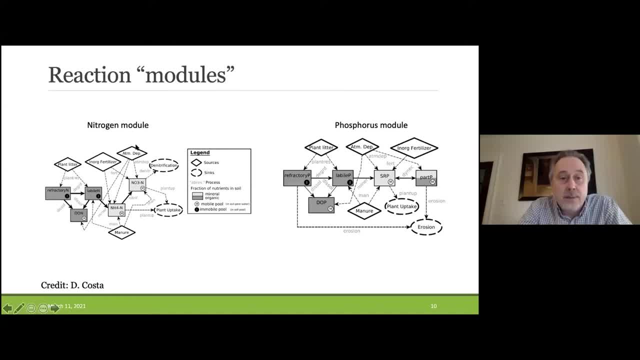 Fertilized application plant, later deposition And the rectangles represent a different pool, the different species, if you want, of nitrogen in the system, And then you also have your sinks, Then here you have your nitrogen module and here you have your phosphorus module. 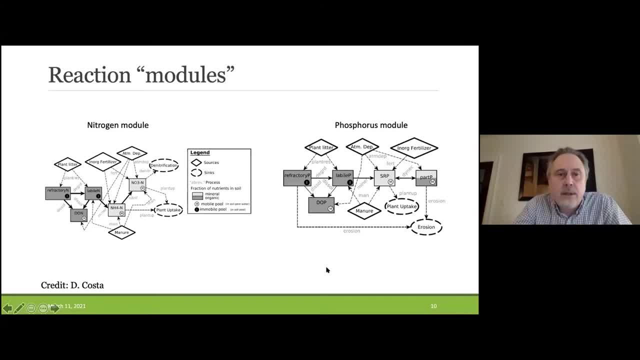 So if you look at that, you might say, well, I'm really only interested in nitrogen, so I'll just use the nitrogen module. Or I'm only interested in the phosphorus module, so I'll just use the phosphorus module. 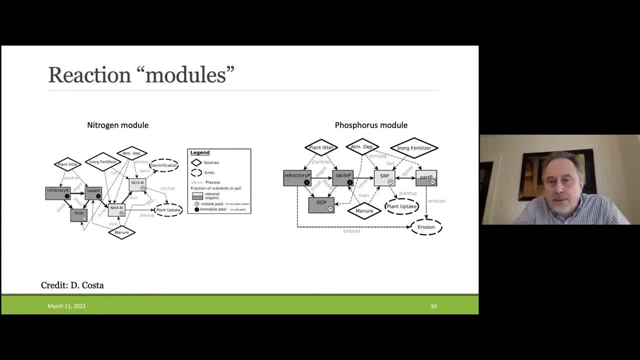 But of course there are couplings between nitrogen and phosphorus, For instance. a lot of experimental and field observation have shown that, for instance, in lakes, if you're looking at, for instance, phosphorus mobility, it actually depends on the availability of nitrate. 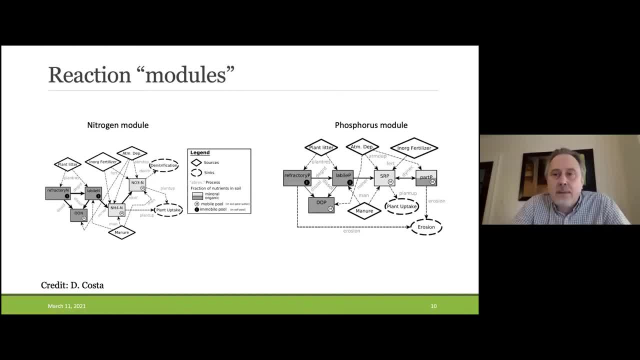 Low nitrate concentrations tend to enhance the mobility of phosphorus or the recycling of phosphorus through the lake system, And if the nitrate is too high you can actually have the opposite effect. So you have also these couplings between your different modules. 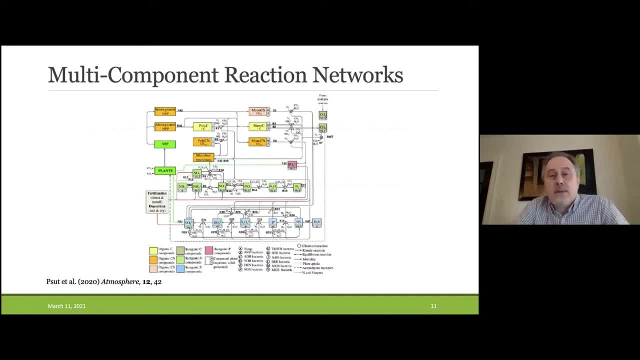 And so I'd like to show this. So I'd like to show this one because I can't even read what's on there. But essentially it's a soil biogeochemical module that essentially deals with nitrogen, with carbon and with sulfur. 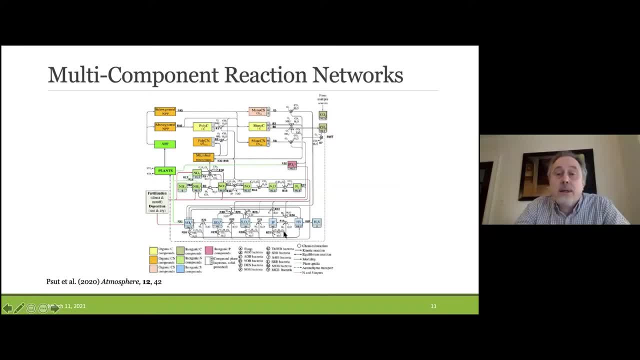 And you see all these lines going between all these different boxes which show these couplings between the elemental cycles of sulfur, nitrogen and carbon in a soil system, And obviously, if you develop one of these very complex, highly coupled reaction networks, 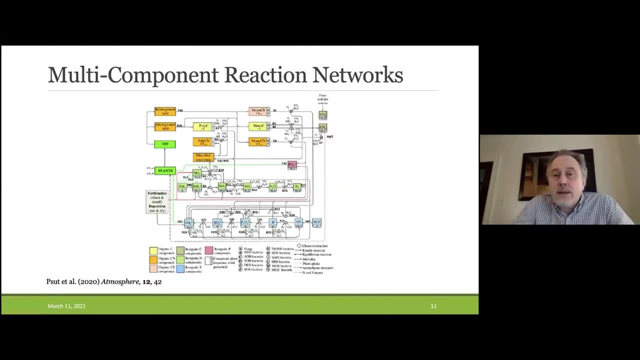 you probably can claim that you are more realistically representing what is really happening in natural soil, because we know from experience and from a lot of data that, indeed, what happens to the carbon is directly linked to what happens to the nitrogen, which is directly linked to what happens here, to the sulfur. 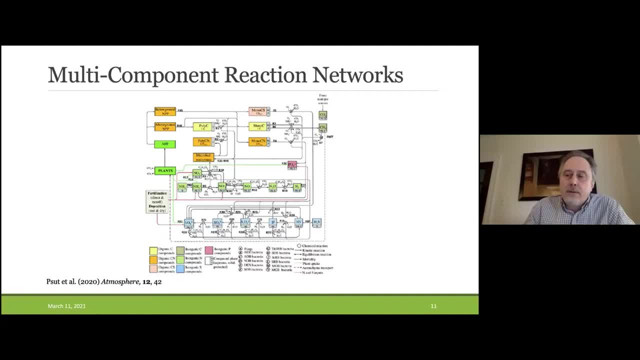 So you have a more realistic representation of your system. But, of course, to run one of these models you have to specify a lot, a lot, a lot of different parameters, And most of these parameters are empirical. There's no real theory. 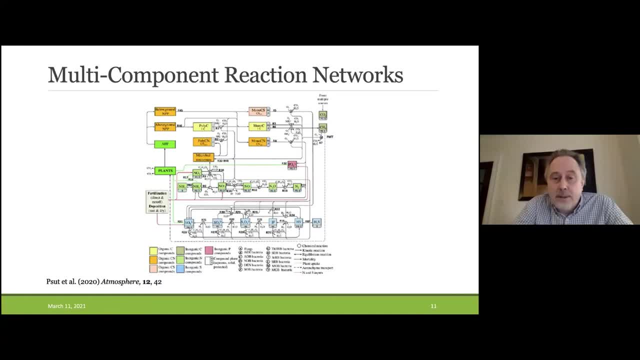 There's no real theoretical foundation to predict these parameters. So by making your model more accurate in terms of its model structure, by saying, well, my model is more realistic, more closely resembling the real world, you of course are increasing the uncertainty associated with the assignment of all these parameters. 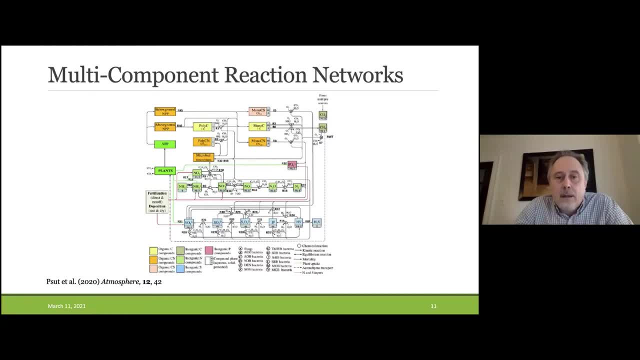 And that's really the struggle we often have in water quality modeling- is to balance the degree of accuracy, the degree of realism that we want to build into our models versus, of course, the uncertainty that's associated with the representation of all these different processes and the parameterization of all these processes. 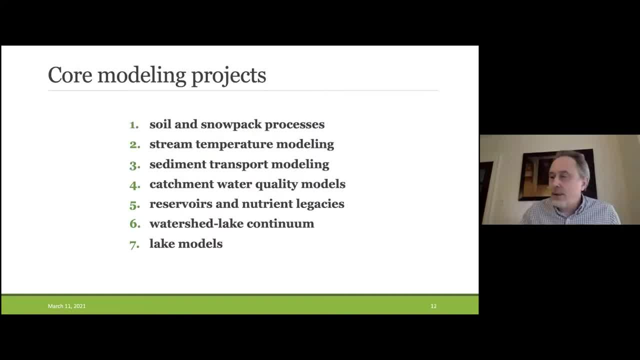 All right, So let's now look at some of the ongoing projects or finished projects within the core modeling group. We'll talk about soil and snowpack processes, stream temperature modeling, sediment transport modeling, catchment water quality models, reservoirs and nutrient legacies. 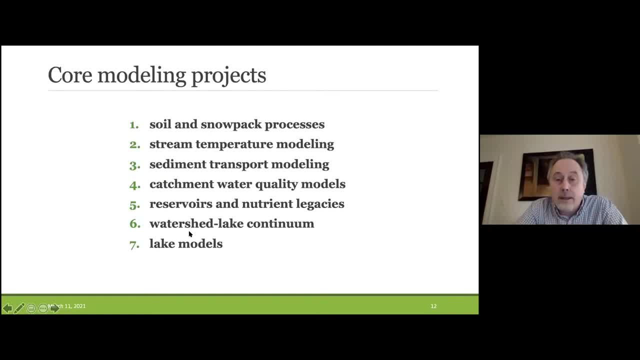 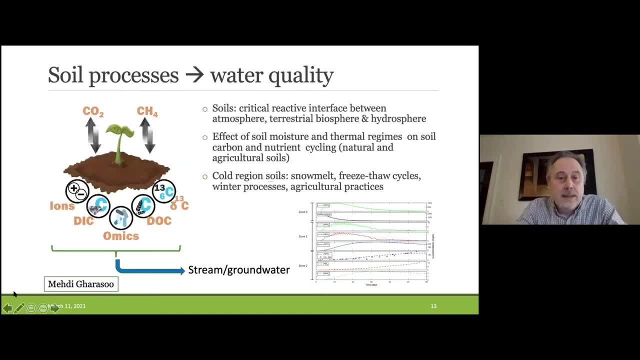 Talk about the watershed, lake linkages and then finish with some examples of lake modeling work. So, as I said, in the upcoming slides, Dan here will always mark the name of the person that is conducting this or carrying out the project. So here we have work from Mehdi. 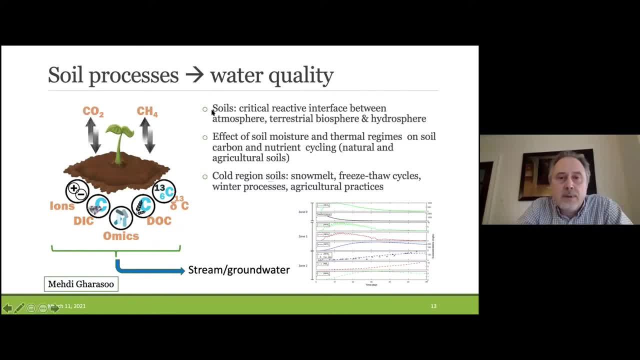 So he works on soils really from the perspective that soils are the critical reactions to the soil, The critical reactive interface between the atmosphere, the terrestrial biosphere and hydrosphere, and particularly has been working on the effect of soil moisture and thermal regimes on soil carbon and nutrient cycling. 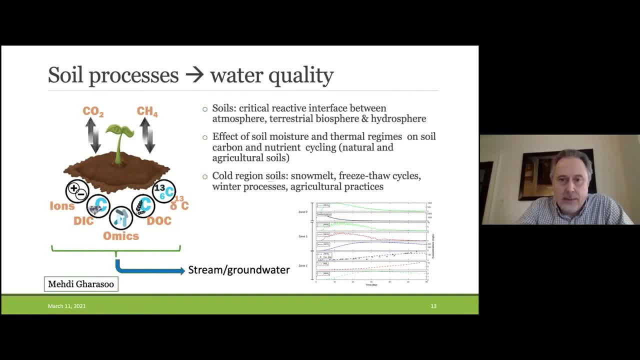 both in natural and agricultural soil, But really, ultimately, from the viewpoint of how is this also going to influence, then, the stream and groundwater water quality and the specific interests, of course, for cold region soils, And so to also take into account processes such as snowmelt. 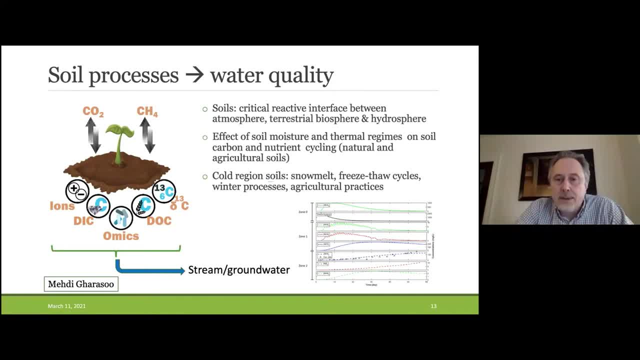 freestyle cycles, other winter processes and also agricultural practices. And just as an example here, this is the results of a reactive transport modeling project, where Mehdi developed a model to account for the leaching of nitrogen from fertilizer that's applied at the end of the fall by farmers so that, essentially, by the time the spring starts, 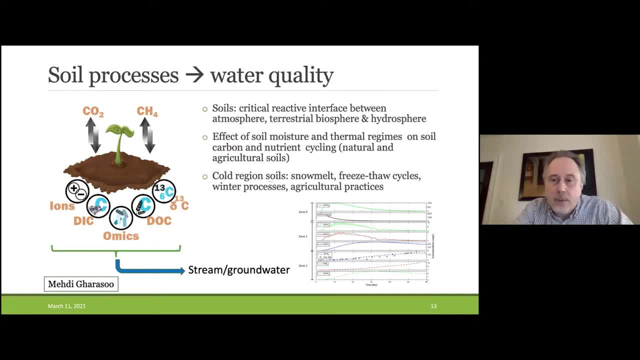 the nutrients would be available for the crop uptake, And so this was done. So this was done under simulated freestyle cycles and freezing of soils also during the winter period, So over a fairly long time period. if you look here at time, it's essentially two months. 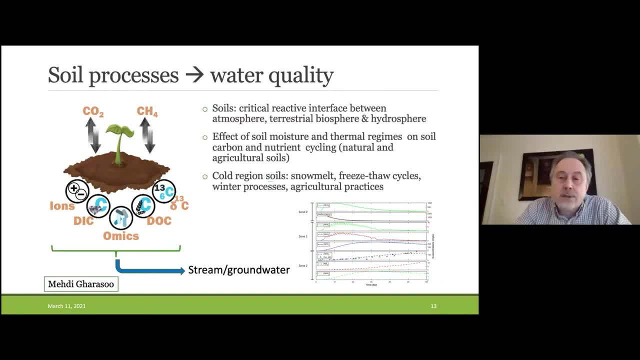 And what it essentially shows here is that, even when soils are frozen and when we have freestyle cycles, some of the nitrogen from the fertilizer is actually leaching downwards into the groundwater, And so that, of course, represents an economic cost for the farmer. 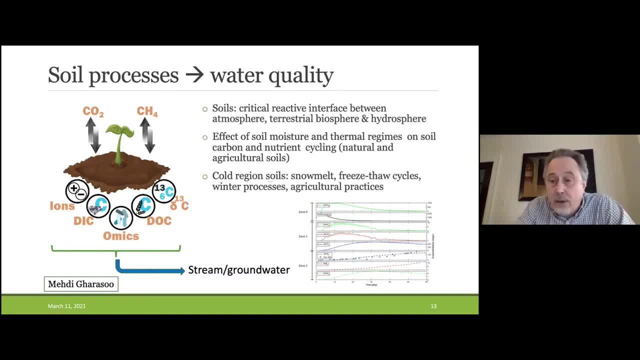 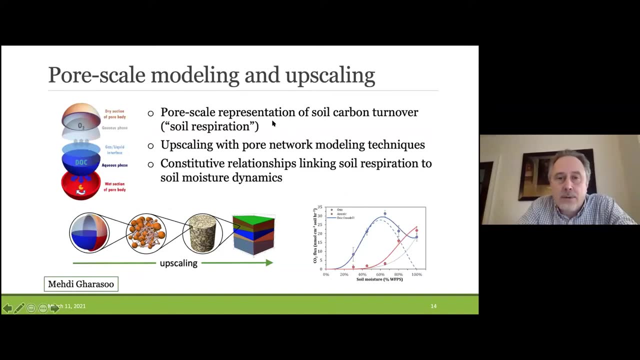 because essentially that's nitrogen that is not going to be there for the crops in the spring, But of course it also can have environmental impacts in the downstream rivers and lakes because of eutrophication. So he's also been working at pore scale. representation of soil carbon. 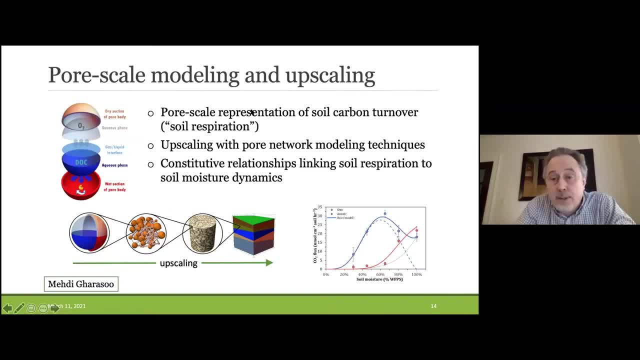 because that's the job of most of the processes affecting carbon nutrients and other constituents, such as metals, in soils, And then use upscaling techniques to go from the pore scale to the macroscopic scale, develop conditions, constitutive relationships that link soil respiration to soil moisture dynamics. 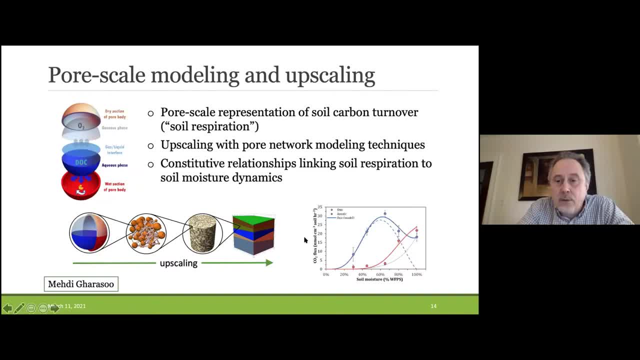 And you see here an example here of CO2 fluxes out of soils as a function of soil moisture. both experimental data and then modeling results. And of course the soil moisture dynamics are driven by meteorological forcings, but also by things like groundwater fluctuations due to groundwater extraction or farming practices such as tile drainage etc. 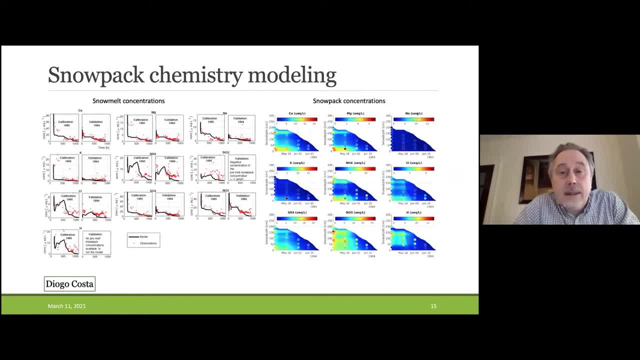 Here's some work from Yogo where he looks at the simulating snowpack chemistry. So the idea is that at the end of the winter, when you have a snowmelt, what is the chemistry associated with that snowmelt? And so, if you go to the right hand side, 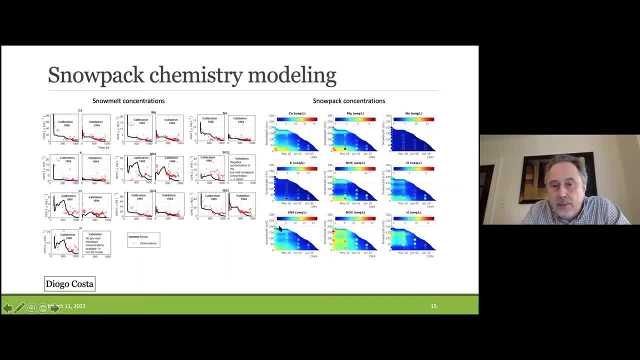 you have these graphs here And, as a function of time, the envelope here is the snowpack thickness. So you see, essentially what you're seeing here is a snowmelt event with also plotted on their chemical concentrations, You have cations such as calcium, magnesium, sodium. 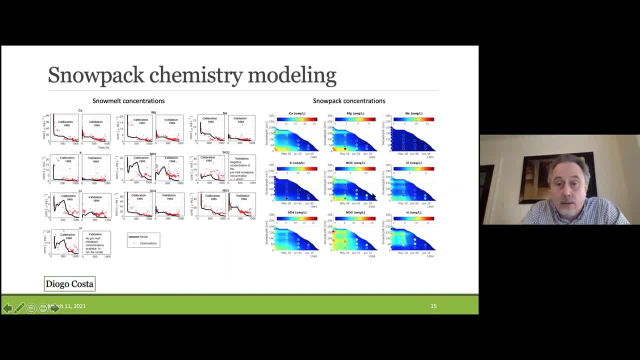 Sodium, potassium, ammonium chloride, sulfate nitrate and protons. And what you see is that in some cases we have significant concentrations, for instance nitrate, because of atmospheric deposition To the left hand side. there you see observations and model calculations of the evolution of the snowmelt chemistry. 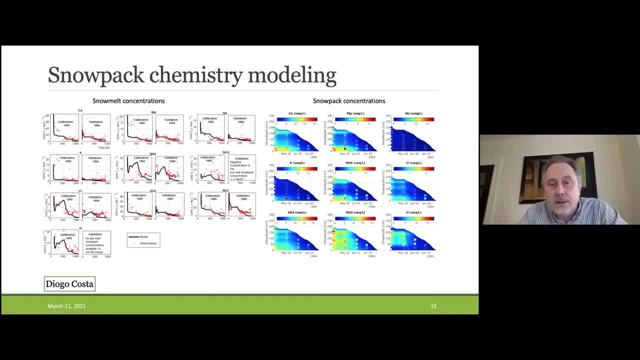 And you can see that there's large variations between the early snowmelt versus the late snowmelt, with typically the early snowmelt being much more concentrated. So we see this whole variation of the chemistry of the snowmelt that then ultimately enters into the nearby stream system. 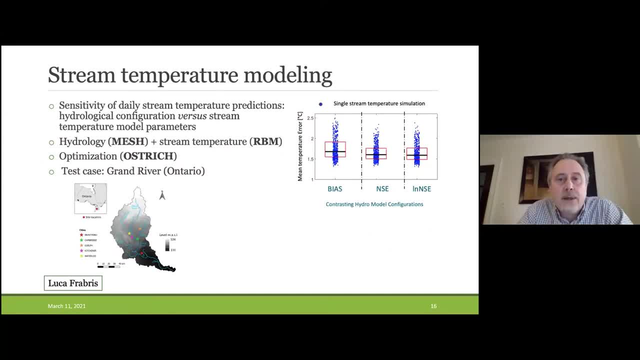 Stream temperature modeling. This is work by Luca, So he was interested in figuring out the sensitivity of daily stream temperatures, hydrological configuration versus stream temperature model. So the mesh surface hydrology model of Environment, Canada, to the stream temperature model known as RBM. 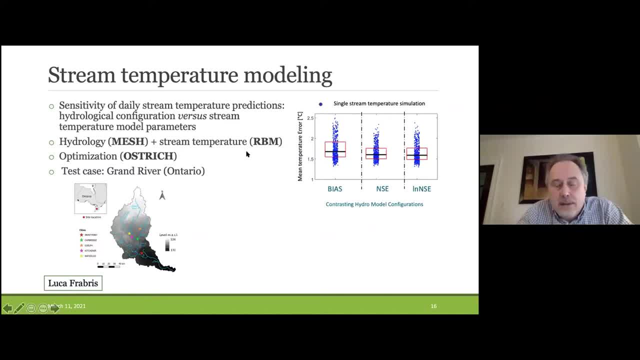 And so this is a stream This predicts, or is based on essentially empirical relationship between headwater temperatures and air temperature. And then he did his analysis using optimization routine known as Ostrich, And his test case is the Grand River watershed in Ontario. 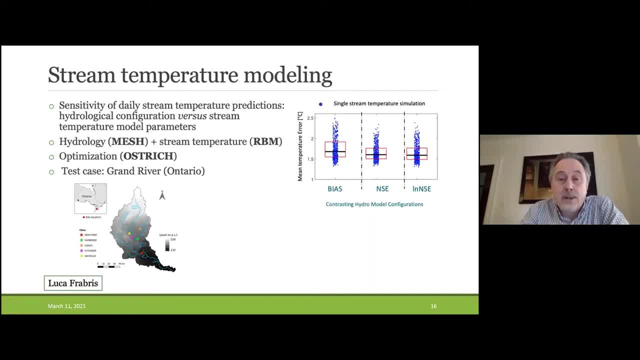 And so what he found in this? that, essentially, the more sensitive, there's higher sensitivity of his predictions on the stream temperature parameters that are imposed rather than on the hydrology. So, in other words, temperature model performance is affected more by the temperature parameters. 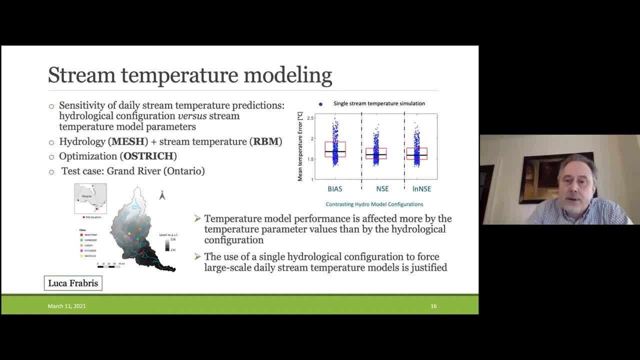 that are supplied to RBM than by the hydrological configuration. The different hydrological configurations he used also have different contributions of surface versus groundwater to the river system, And so that also means that the use of a single hydrological configuration to force large scale daily stream temperature models is justified. 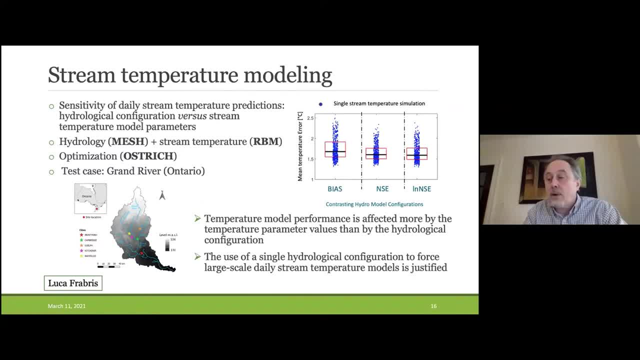 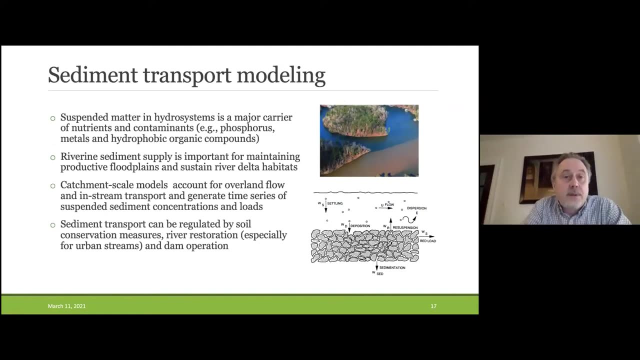 So that of course also opens the way to forecast of stream water temperature in the mesh model And sediment transport modeling. obviously we're very interested in sediment transport because suspended matter in hydro system is a major carrier of nutrients such as phosphorus. 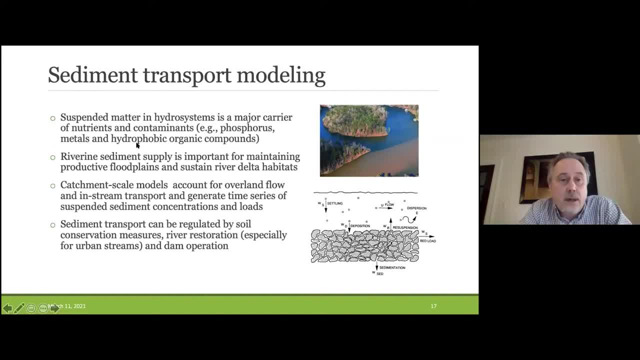 but also contaminants, whether it's metals or hydrophobic organic compounds. If we have a riverine, sediment supply is important for maintaining productive floodplains and sustained river delta habitats, And I'll come back to that in the next few slides. 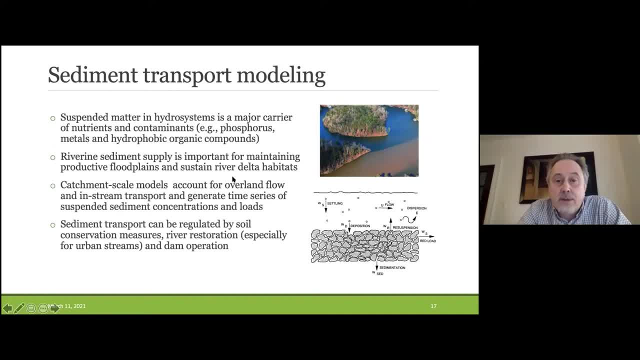 And then a good catchment scale sediment transport model should account for the overland flow which supplies the sediment to the river system, and then the in-stream transport and processes, and then generate time series of suspended sediment concentrations and loads, And then this type of modeling capacity is important also. 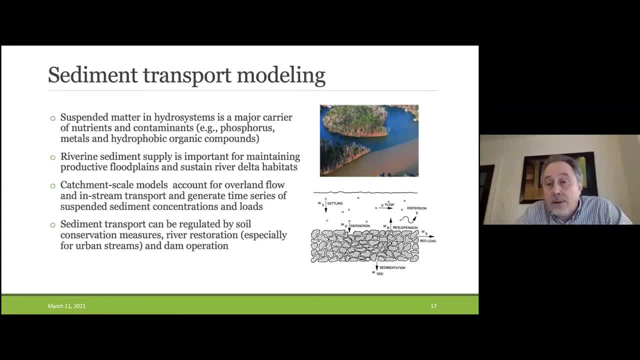 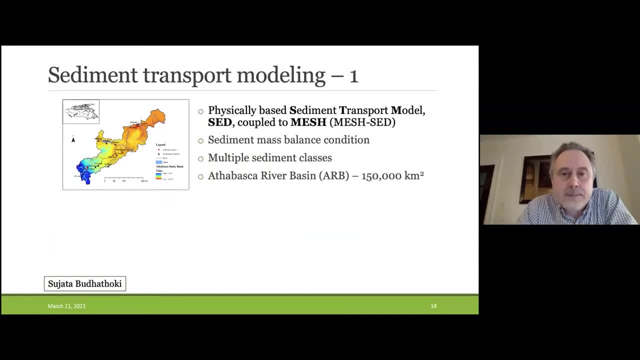 if we want to inform soil conservation measures, river restoration strategies or even dam operations, which all are very much influenced or influence sediment transport. So the first project here is from Suyata, So she works on the Atabasca River Basin. 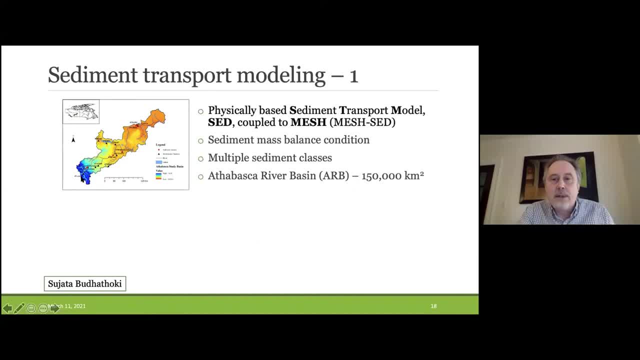 so a huge river basin, And she has been using MESH again, the so the Grand Canada modeling platform for surface hydrology, And she has coupled this to the sediment transport model, SED, And so that then results in the MESH SED. 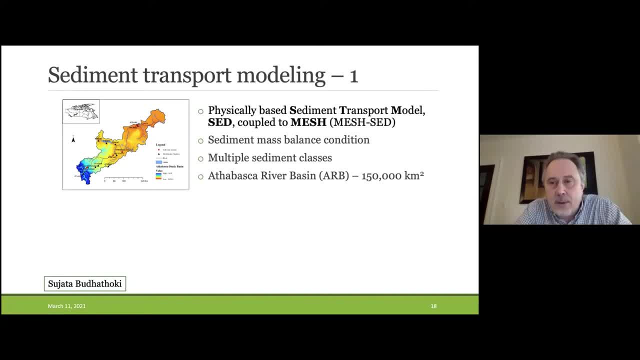 So the equations in the sediment transport model are the classic equations that deal with sediment transport, deposition, use, tension, etc. And if you remember what I said about the conservation equations, well, it appears here to the sediment mass balance condition. The model has the capability to account for multiple sediment classes. 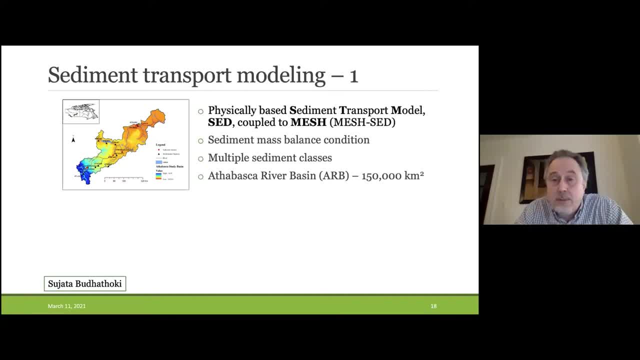 which is important for future applications on contaminant transport, because different sediment classes have different affinities for different contaminants, And so here are some of her results. So on the left hand side you see the calibration using data from 2003 to 2009,. 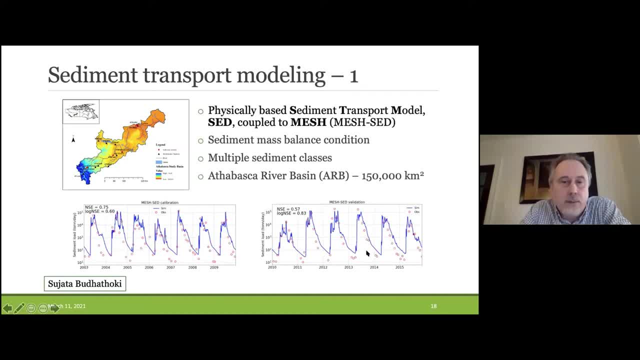 and then the validation from 2010 to 2015.. And so the blue lines, of course, are the model, The red dots are the data, And so you see this very strong seasonal dependence of sediment transport through the river system, here, with the high 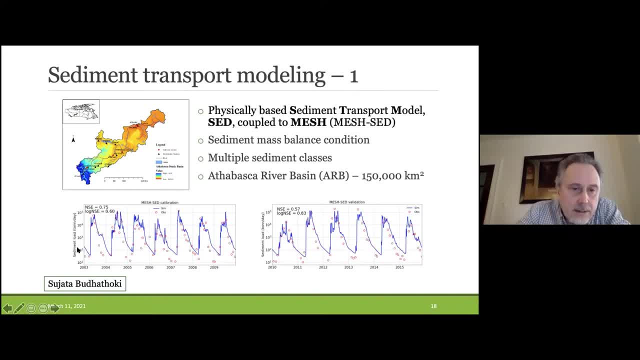 by the way, the vertical axis here. If you look at the scale, it's a logarithmic scale, So you see order of magnitudes higher sediment concentrations or loads. In fact, these are loads here during the summer, when we have high flow rates. 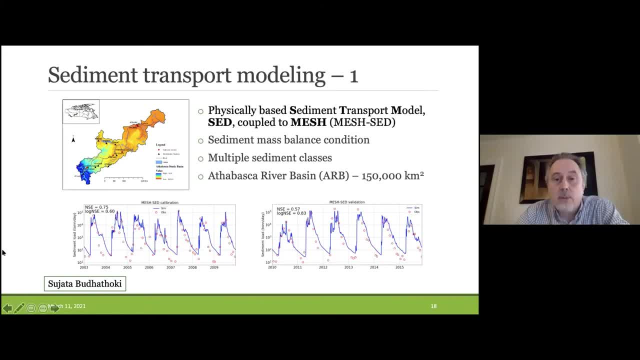 and then very low during the winter, when parts of the river are ice covered and the flow rates are much, much, much lower. And of course, the sediment transport or the turbidity, seasonal fluctuations in the whole river system are important for the river system itself. 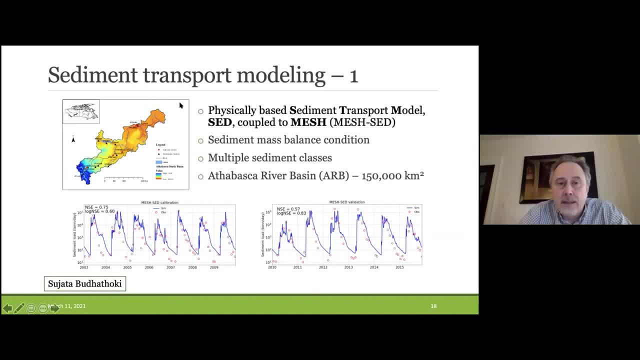 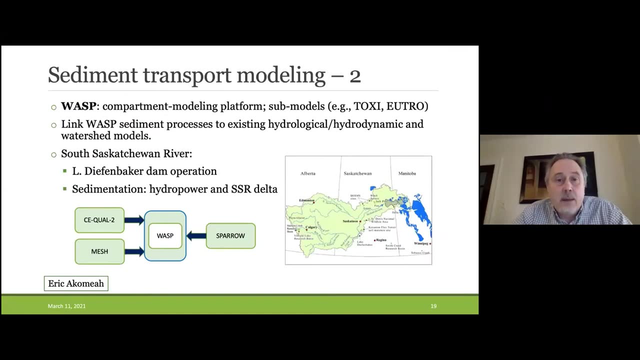 but also very important for the Athabasca Delta And, as you know, probably know, the Athabasca Delta is a biodiversity hotspots and it's also very important for the livelihood of the indigenous people living in the Delta region. So another sediment transport modeling project is by Eric. 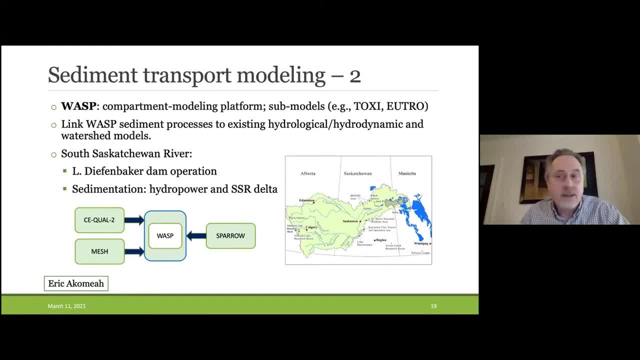 And so he's using the WASP model, which is an EPA model, the water quality analysis model, the water quality analysis simulation program. It's a program that I think was developed early in the early 80s and then since then has had very, very many different versions. 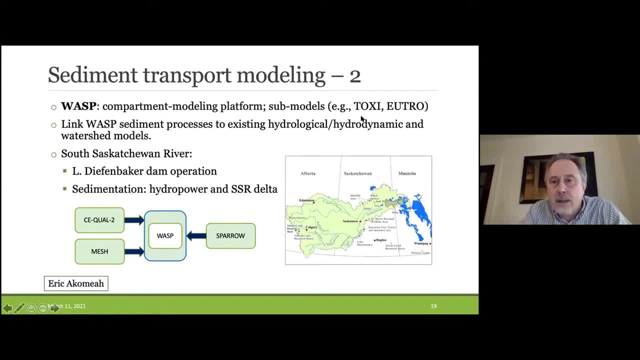 And, in particular, they've kept adding submodels to it. For instance, some that Eric is particularly interested in are the TOXI and the UTROS submodels: TOXI for toxicant transport, FADEN transport and UTROS for eutrophication. 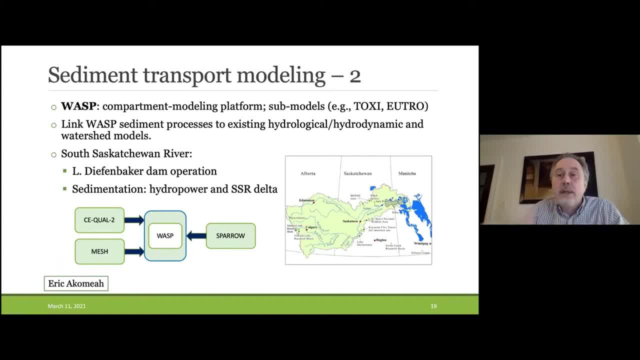 And also they've also increased the capability to link WASP to other models, to other modeling codes. In particular, what is done in Eric's project is to link WASP to SPARO, so a catchment model to MESH again. 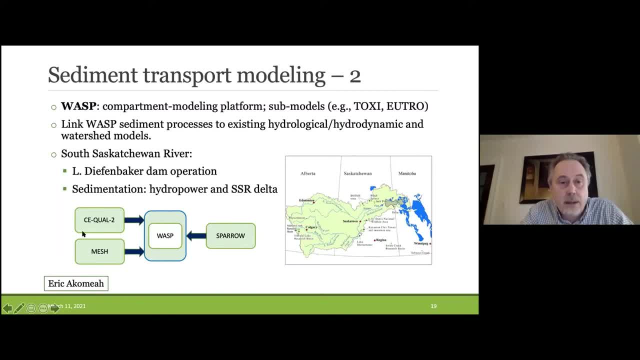 but also particularly for the work that will take place in Lake Diefenbaker, to the CQUAL2 model, which is a two-dimensional hydrodynamic water quality model, And so his focus is on Lake Diefenbaker. how Lake Diefenbaker dam operations. 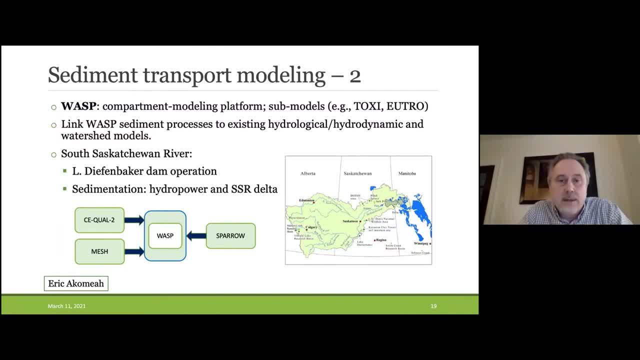 are changing the sediment transport along the South Saskatchewan River, and also of interest in this project is obviously the sediment delivery to the delta of the South Saskatchewan River which, as you can see on this map, is also important because it is the gateway to Lake Winnipeg. 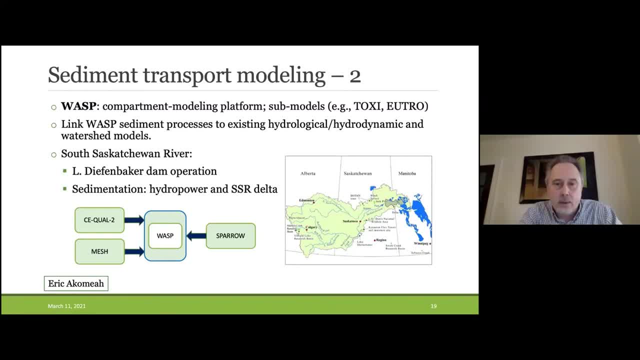 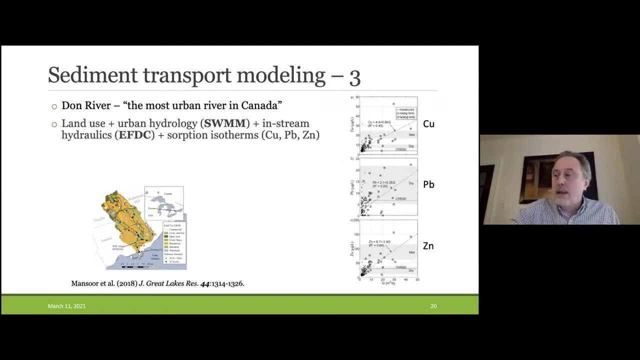 And so at some point it would of course link this work and the sediment delivery through the South Saskatchewan River and the associated nutrients and contaminants to water quality simulations in Lake Winnipeg. A third project, which was finished actually fairly early on when the core modeling group was started. 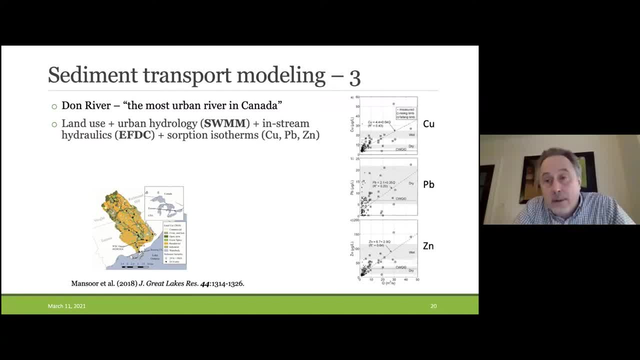 In fact we weren't able then. we were still looking for core modelers, so we used some of the financial means to hire some smart students that could help us with the coding. And this is on a much, much smaller catchment. 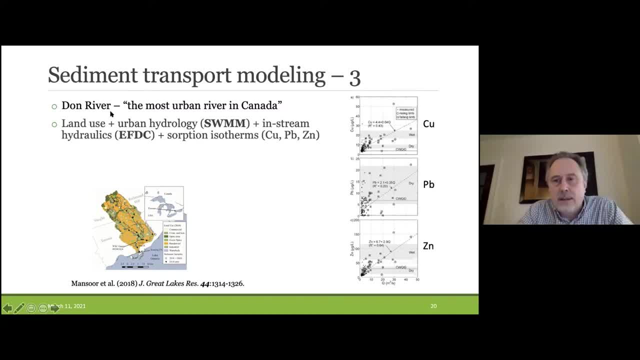 the Don River catchment. It's about the catchment. I think is about close to just under 400 square kilometer. But the notoriety of the Don River is that it's the most urban urban river in Canada, So its entire watershed. 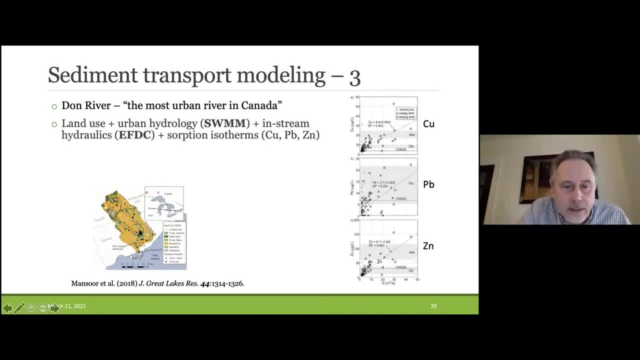 is within the Toronto metropolitan area And if you look at the map you have some little green spots. That's kind of open areas and green areas, but the kind of light brown to orangey color is essentially all residential areas. So it's a classic example. 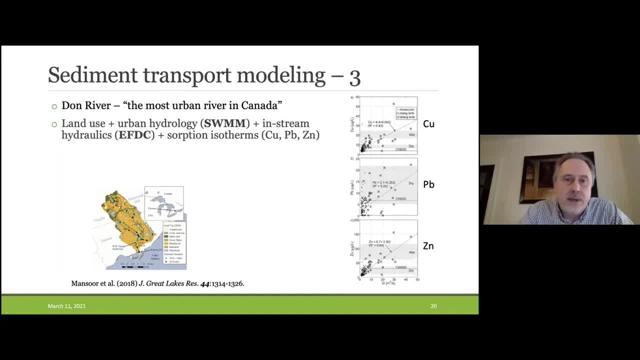 of the urban stream syndrome. Parts of it have been straightened. There's a lot of infrastructure, There's weirs, There's bridges crossing the Don River, And so it's been essentially a problem child for the TRCA, the Toronto and the TRCA. 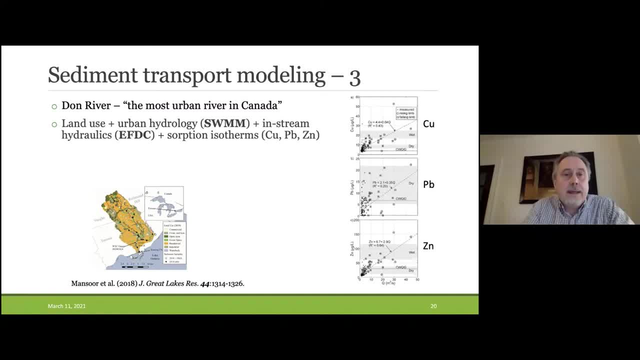 the Toronto and Region Conservation Authority, And so what we've done, then, is to couple land use information to an urban hydrology model, the SWMM model, the stormwater management model, which is very important in this case, because about 95% of all the stormwater 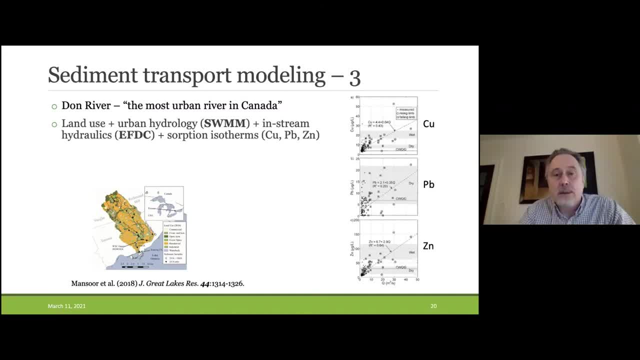 in the catchment is actually straight into the stream, And then couple that to the in-stream hydraulics model, the environmental fluid dynamics code Also. so those are two EPA models. and then sorption isotherms for copper, lead and zinc. 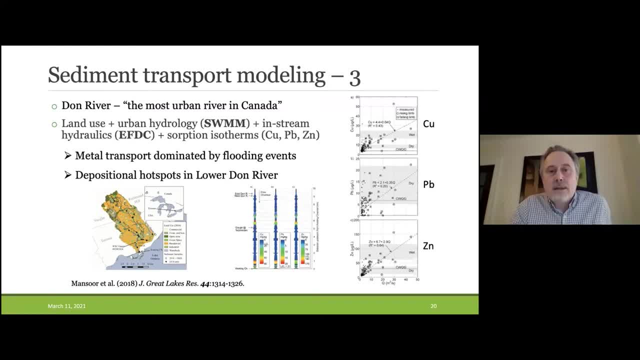 And so some of the findings. not surprisingly, metal transport is dominated by flooding events, And so you can see this in these CQ relationships. So it's concentration versus discharge. We have these positive relationships. So at high discharge we have high concentration. 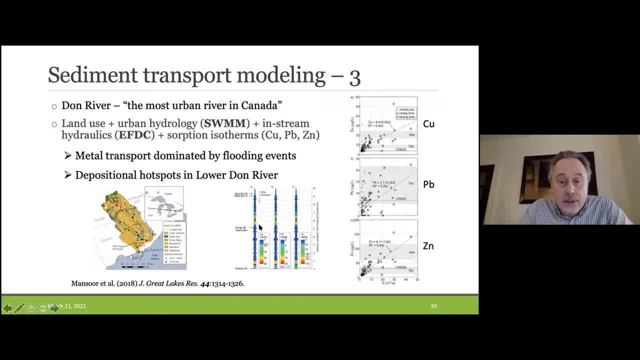 high leakage. We have loads of metal, which also means that most of the metals- a lot of these metals- are legacy metals- have not been essentially transported to the lower part of the Don River, And this is a representation of the lower part of the Don River. 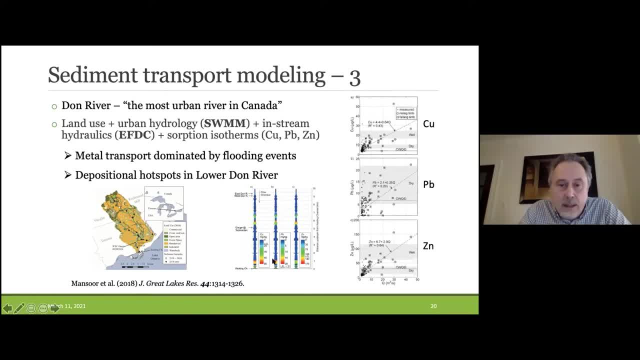 And we have copper, lead and zinc, And you can see, we have these hotspots where the metals are accumulated, And this information is, of course, important because it tells us that's where cleanup of the river system should take place, rather than waiting until it ends up. 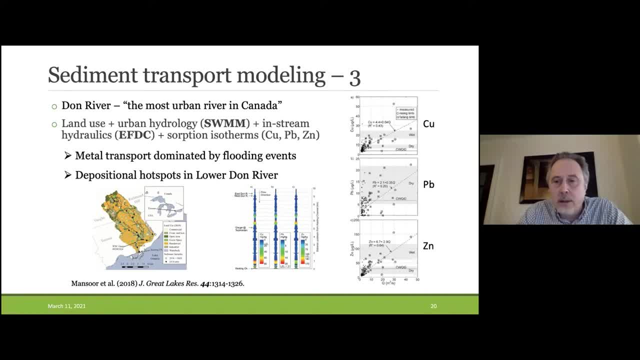 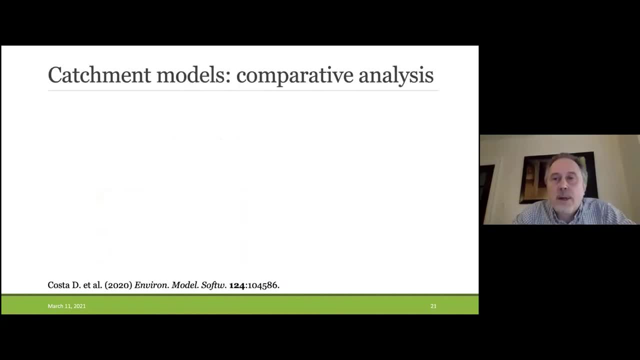 in the Toronto Harbor, where dredging is much more complicated and costly. All right, So now I've already shown you several projects where existing models are used or existing models are coupled. So of course it means that there is a lot of catchment scale models. 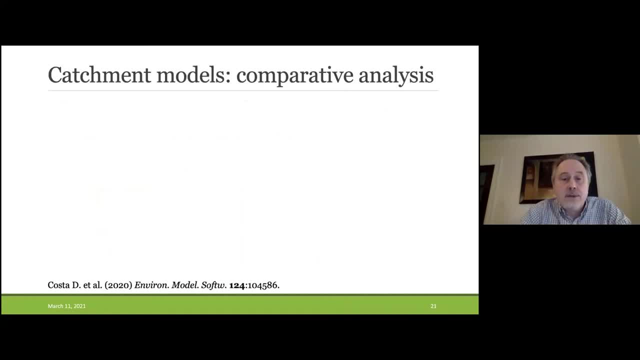 with water quality capabilities out there, And so an interesting study that was done about a year ago. also early on was to say, okay, let's look at all the available models and let's compare the capabilities. what functionalities are represented in some of the models and not the other models? 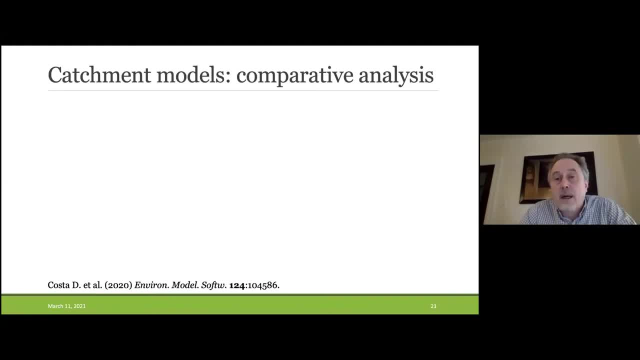 And, of course, with an interest particularly of how well are they in representing or accounting for the processes that are particularly important in cold regions. So here, for instance, here are the different models that have been compared by YugoHype, the HSPF. 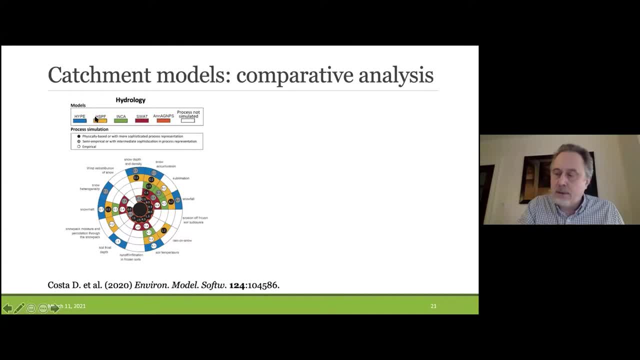 so that's the HPS, and for the hydrological simulation program in Fortran, then the integrated catchment model, the INCA model, the SWAT model, the soil and water assessment tool, and then the ANA. GNPS is a model that's specifically designed for agricultural watersheds. 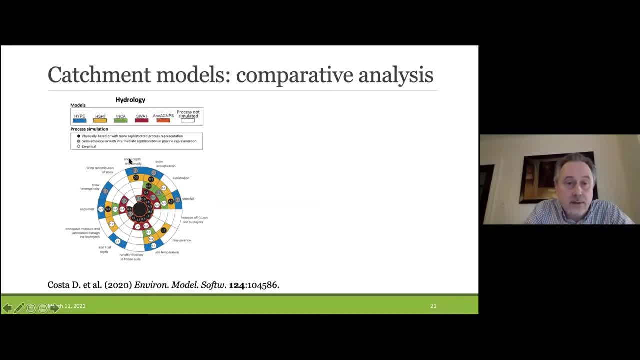 And so what you see in this figure here, this is for the hydrology. So you look at, you go around the circle here and you have all these different processes that are obviously very important in cold regions: hydrology, for instance, snow accumulation. 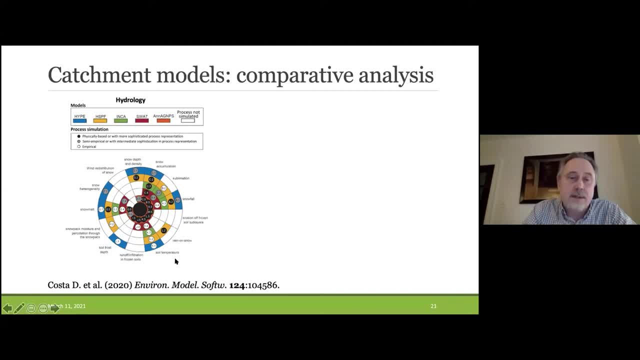 sublimation, snowfall, erosion of frozen soil, sublays, rain on snow, et cetera, et cetera. So all this indicate whether the corresponding model actually has these processes, these factors represented in their code, And you can see that there's even certain processes. 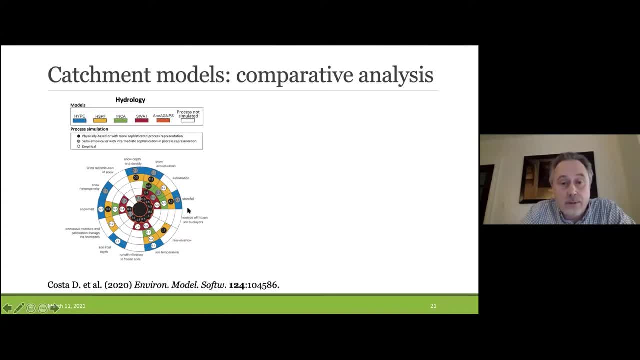 like wind, redistribution of snow or the erosion of frozen soil sublays, that are not represented in any of these models And in some cases, just one or two models represent a particular process And in some case, like soil temperature, it's represented in all these different models. 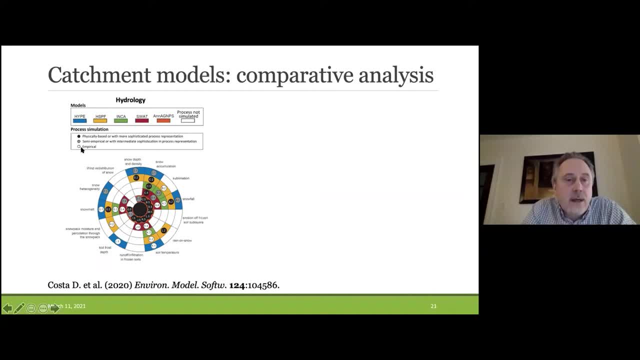 What the analysis also does is to identify whether the processes are represented by physically based or more sophisticated process representation, or whether they're empirical or somewhere in between, And so the analysis is also applied to, for instance, in this case, nitrogen species and nitrogen cycling. 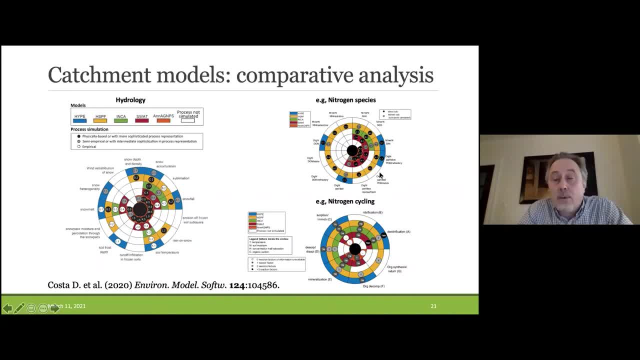 Again looking at the different models, for do they represent these different nitrogen species And do they represent the processes that control the cycling of, in this case, nitrogen? And you can see that only one model, the HSPF, is actually representing all these different nitrogen species. 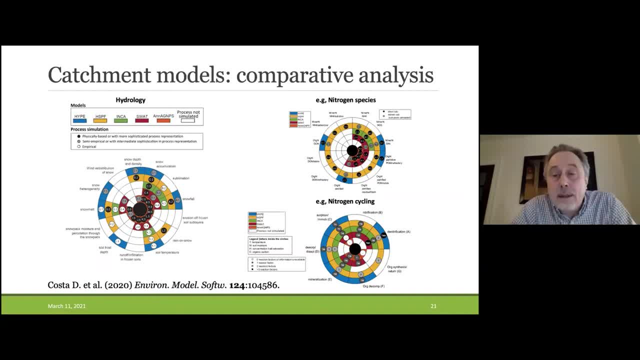 and the different processes. So this of course helps you guide, choosing a model for a particular application you're interested in, But it also offers, of course, opportunities to say, hey, there's a certain I really like, a particular model. 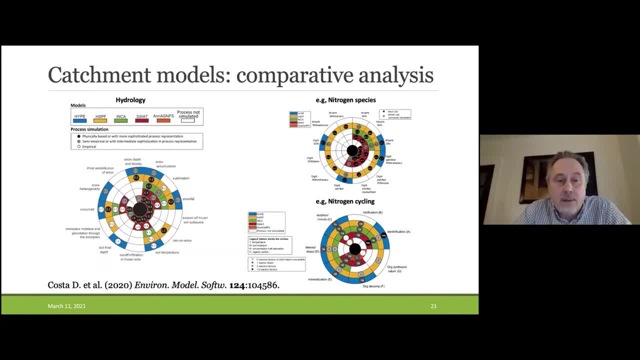 I say really like the Inca model, but I also really need to have a better representation of runoff infiltration in frozen soil. So it offers opportunities to us discovering where we can basically add in or upgrade these models, because most of these models consist. 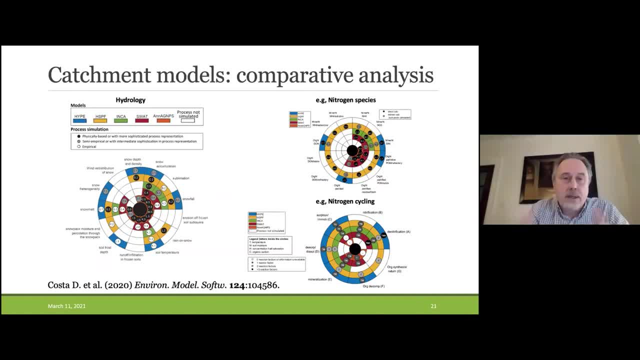 are. several have been worked on for several for a long time. Some of those go back to the 1960s of these models, when they were first developed, And so over the years functionalities are can be added to them. So just to look at one example of an upgrading: 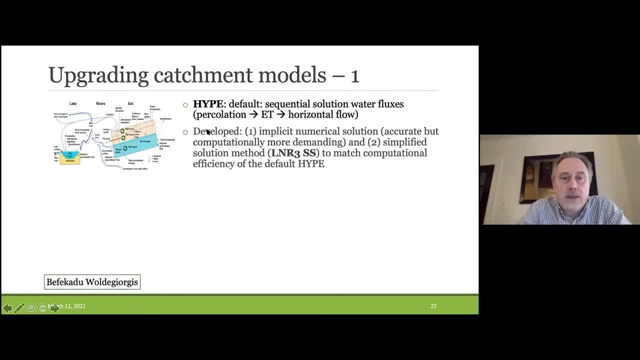 of a catchment model by Befe Kadu, So he worked on on HYPE, So it's a semi-distributed hydrology biogeochemistry model. It has a very extensive representation, for instance, of carbon nitrogen and phosphorus. 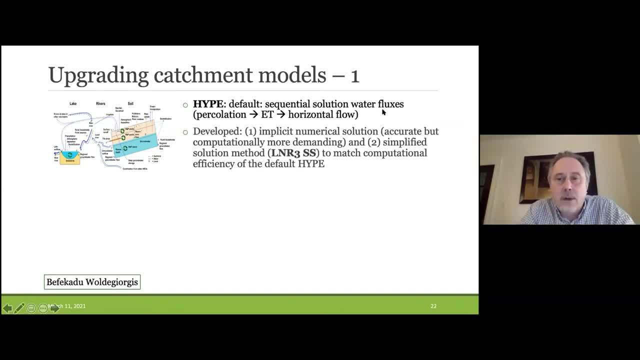 But he specifically looked at at how HYPE is solving the, the water fluxes, And in the default HYPE model it's done sequentially. So essentially first percolation is calculated, then evapotranspiration is calculated, then horizontal flow is calculated. 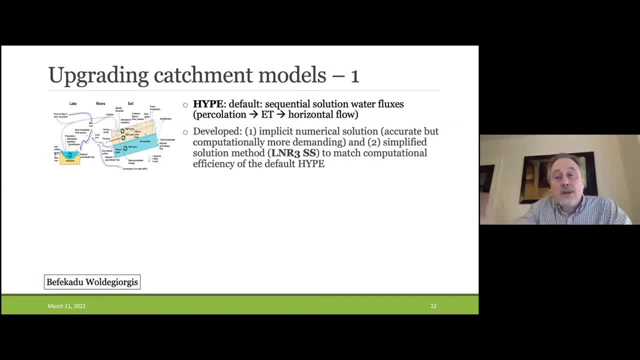 And what he was able to show is that this, this sequential approach, which is computationally efficient, may actually yield unrealistic water flux, In particular, under certain conditions. it predicts that there's no horizontal flow. Well, we know that there should be horizontal flow. 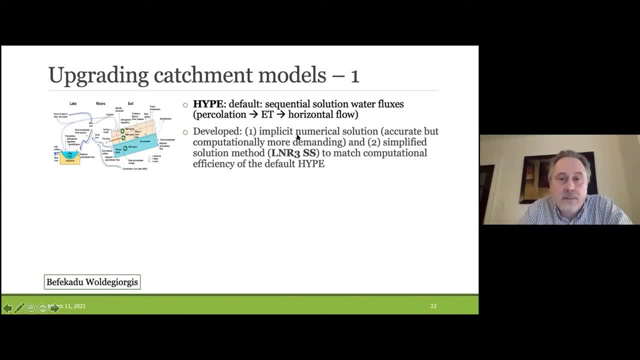 So to address that, he developed a fully implicit numerical solution, So solving all the equations for these different water fluxes at the same time, which of course gives you the more accurate solution. I particularly did that by looking at whether the horizontal flow was predicted under given conditions. 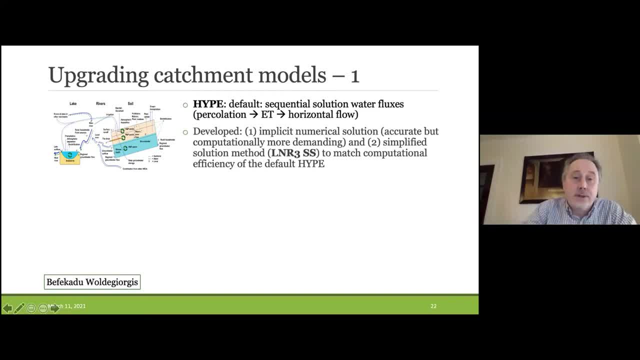 but it's computationally much more demanding, And particularly if you want to do a lot of runs and if you want to run this at a large catchment scale and you want to look at the carbon nitrogen and phosphorus at the same time. 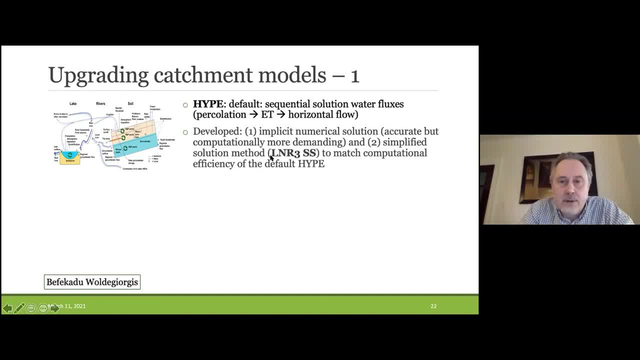 So then he produced a simplified solution, the LNR3SS solution, And the goal was to essentially have to match the computation efficiency of the sequential solution that's in HYPE, but also to, of course, match the the accuracy of the implicit numerical solution. 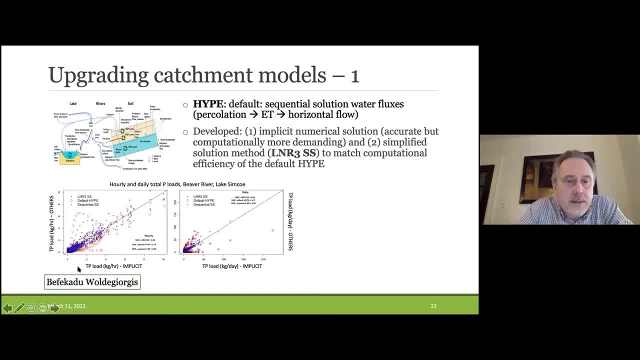 And so here are some results where he compared, for instance, the TP load calculated by the implicit method. So that can take, can consider the, this the vertical axis here, as the true solution And then compare this to the, his simplified solution. 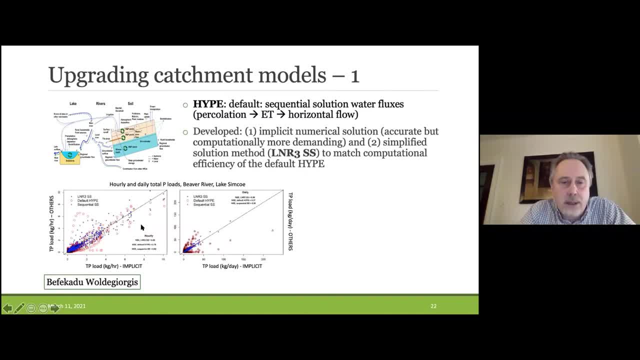 but also the default HYPE solution is also another solution here. But if you just look at the blue and the red symbols, you can see for the. these are the hourly loads and the the daily loads. you could say well, 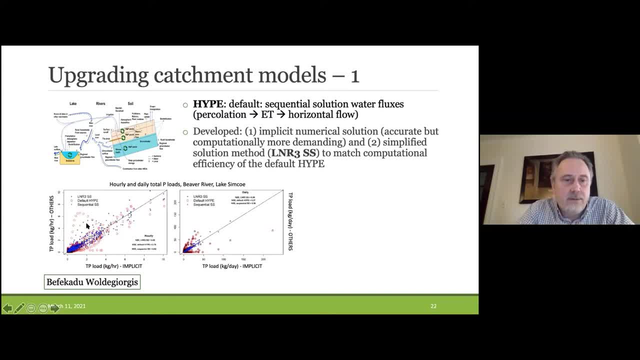 you have some kind of weird stuff happening here, with very high loads predicted by the default HYPE method. But overall it works kind of okay for the default method and you can get a better match of the one-to-one curve for the for the simplified solution he developed. 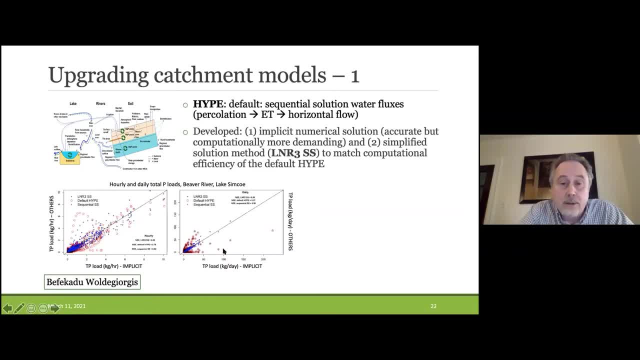 But it becomes. particularly if you look at the daily loads, you can see that there's particularly the high loads are significantly underrepresented by the by the default HYPE load. So his conclusion is that that obviously more realistic flow paths simulations will yield you a more accurate contaminant load estimates. 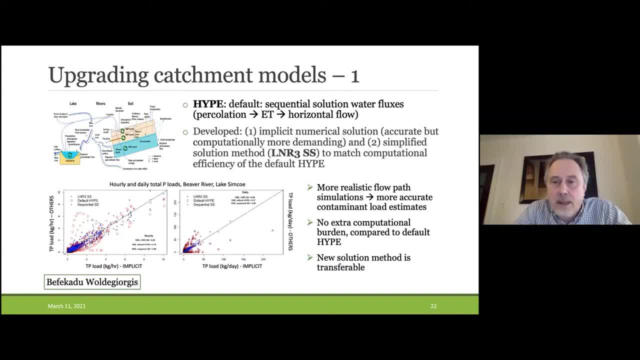 because the load estimates are directly dependent on your, your flow paths and the the flow or the flow of water according along these different flow paths. It has no extra computational burden compared to default HYPE. And also this, this solution approach that he presents is also transferable to other 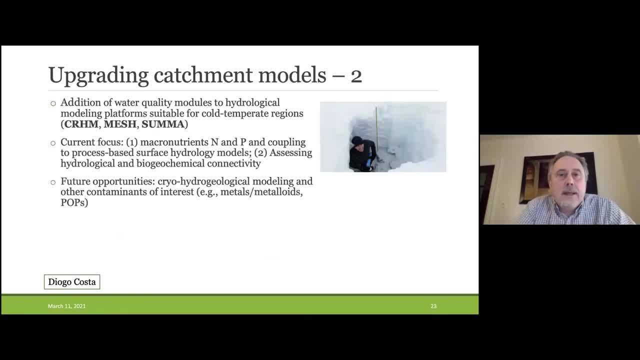 to other hydrological models. Okay, Another example is from Diogo, where he's essentially adding water quality modules to modeling platforms that are specifically that are very suitable for cold temperature regions, in particular the cold regions hydrological model, the CHR-HM and the mesh model. 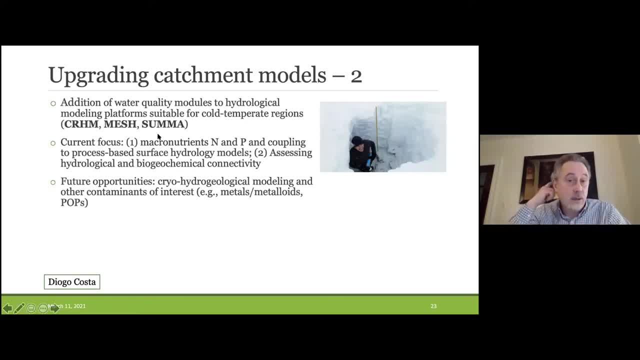 And then also now working under the SUMA. this, this new approach, modeling approach that's also been strongly pushed by the, by Martin Clark, So for the moment he's he has focused mostly on the macronutrients- nitrogen and phosphorus, and the coupling to these process-based service. 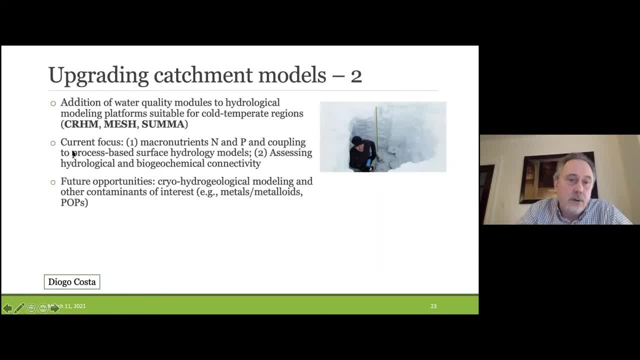 hydrology model And it's also been assessing then, or using this to assess, the hydrological connectivity and see how that then translates into the biogeochemical connectivity. So here, for instance, some results from the South Tobacco Creek in Manitoba: 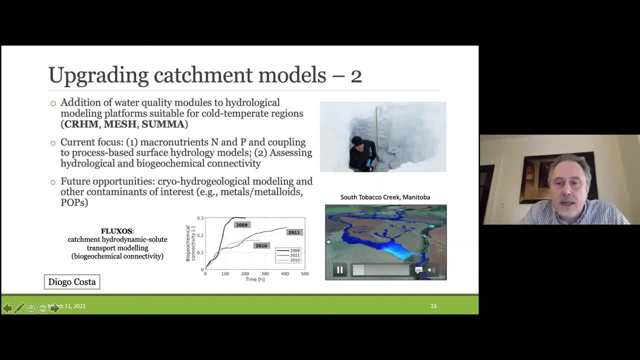 And, yeah, it works here. You can see that it's a very flashy hydrological system. Sometimes there's certain creeks that are active activated, sometimes they're not activated. So essentially it's a very variable hydrological system, And so what he's been looking at is also, then, how this hydrological 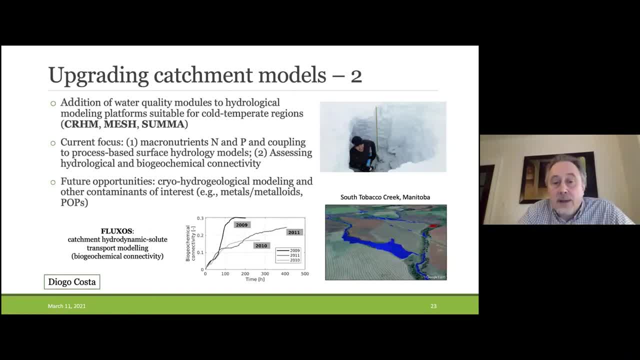 variability translates in the variability in the biogeochemical connectivity, And here you see this: biogeochemical connectivity trajectories for three different years, And you see that these three different years yield very different trajectories, And so capturing this is, of course, a major advance in our understanding. 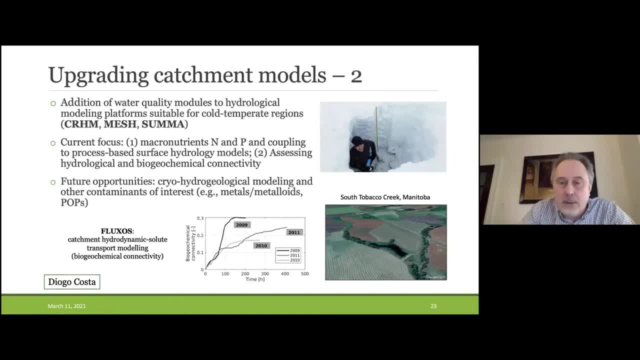 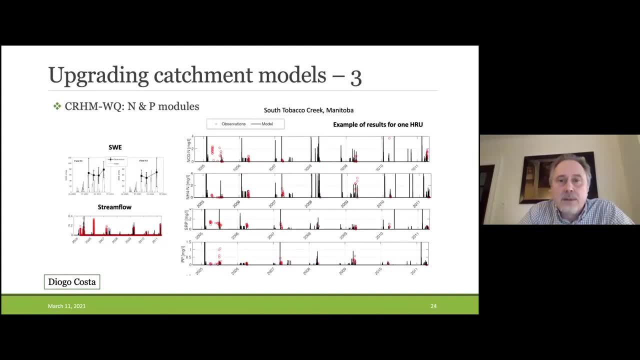 how the system work as biogeochemical flow and transport, transport and reaction systems. Here are some other results from the South Tobacco Creek using the cold regions hydrological model WQ for water quality, which now includes nitrogen and phosphorus modules. 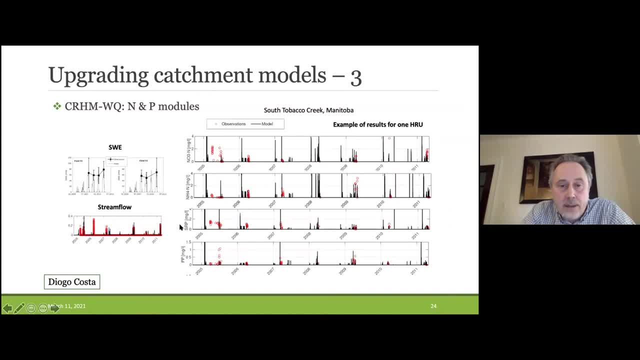 You see here time series for nitrate, ammonia, soluble reactive phosphorus and particulate phosphorus, And if you look, I mean you can see that it's a very flashy system, Obviously. so you have these events and for these events, 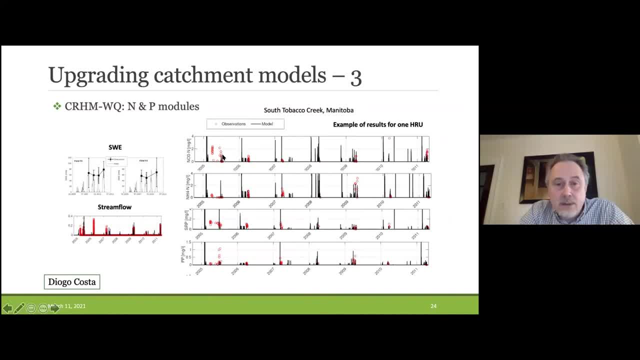 you can see that in some cases- well, there's still some issues here in this- maybe this first event for nitrate and SRP, But what I find interesting is that you can see that it captures the model, captures these events where you have N high, nitrate and high. 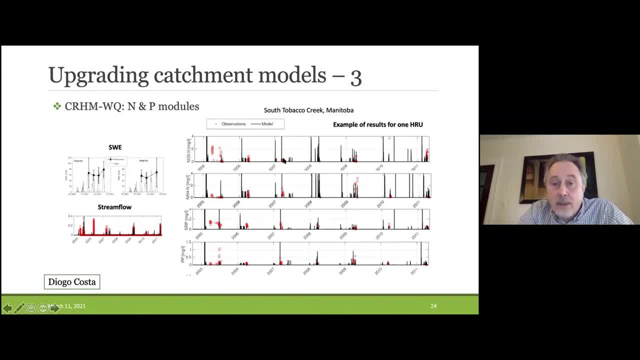 ammonia, but also events where you have high ammonia, very little nitrate, and then events like this one where you have high nitrate and low ammonia. So you can see that that kind of that biogeochemical- or at least this is probably reflects. 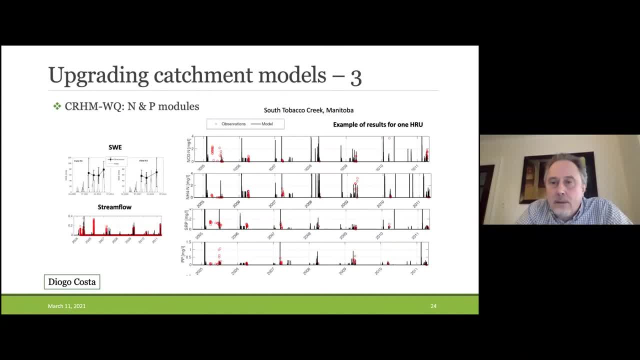 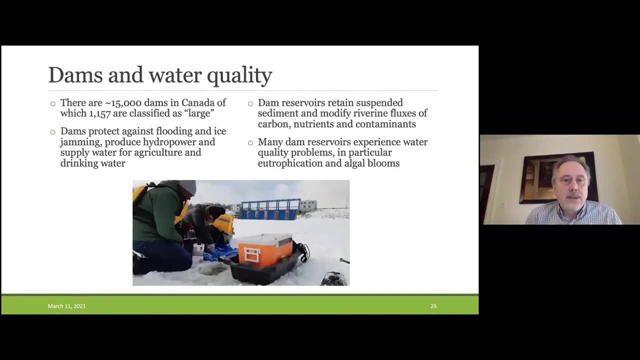 I think- and that's something that Yogo can talk more more, more knowledgeably about- but this probably means that there's different sources that are activated during these different events. different land-based sources of nitrogen- Okay, Then dams and water quality. 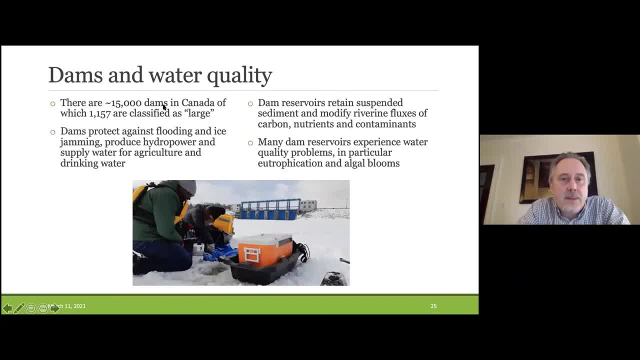 just as background information, about 15,000 dams in Canada and about over thousand are classified as as large or higher than 15 meters. Obviously, these dams have a lot of beneficial functions: They protect against flooding, ice jamming, they produce hydro power and supply water for agriculture and drinking. 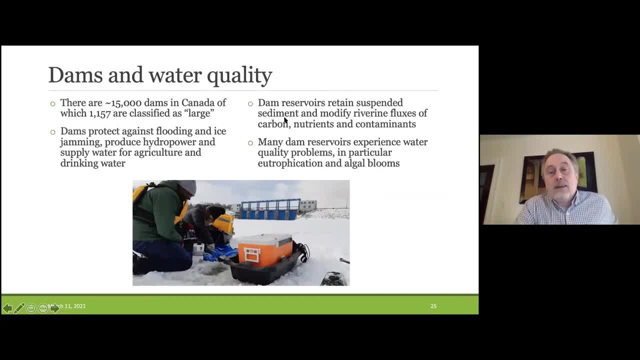 water Dams also retain suspended sediment- And we've talked already about sediment transport modeling activities- and they also modify the riverine fluxes of carbon, nutrients and contaminants. And also many dam reservoirs do experience water quality problems in their reservoirs. 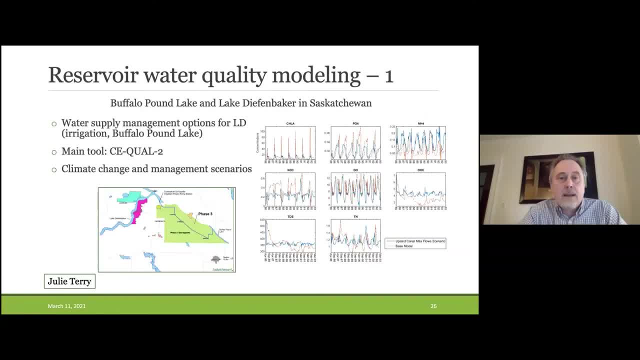 in particular eutrophication and all the groups. So one project on reservoir water quality modeling is by Julie and she works on Buffalo Lake and Lake Diefenbaker in Saskatchewan And her work is closely tied to water supply management options that are 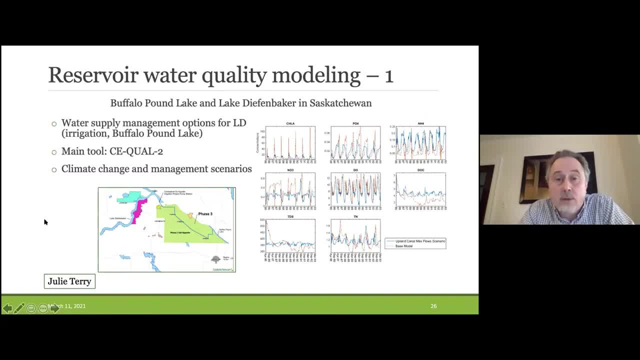 being considered for Lake Diefenbaker, particularly to augment the water availability for irrigation, but also the water that can then transfer, being transferred from the Diefenbaker. here's Lake Diefenbaker to Buffalo, Pound down here. 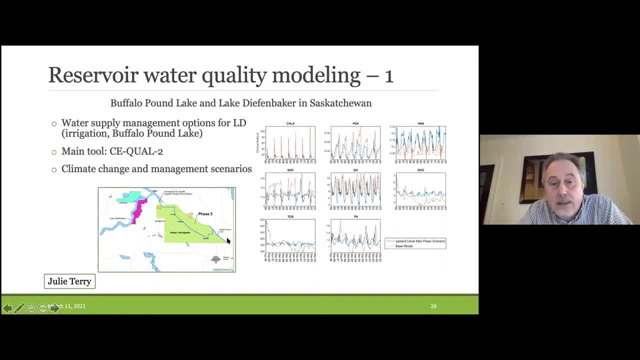 this very long kind of reservoir, that is the, that also supply drinking water, But also supply drinking water to the city of Regina. So the tool she's used is sequel to it, So it's a two dimensional. two stands for two dimensional hydrodynamics. 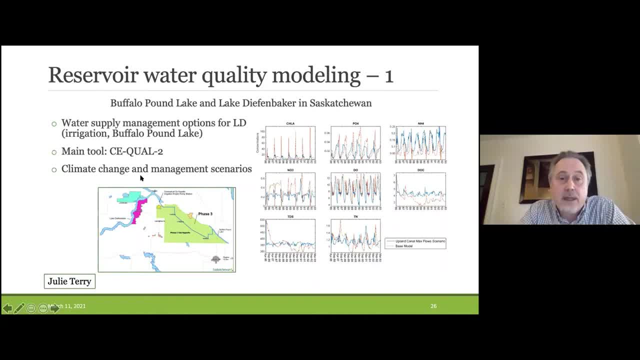 water quality model And she's exploring different climate change and management scenarios in these two environments and Lake Diefenbaker, but mostly for the moment in Buffalo Pound Lake, You see, for instance, example where a baseline model sort of kind of 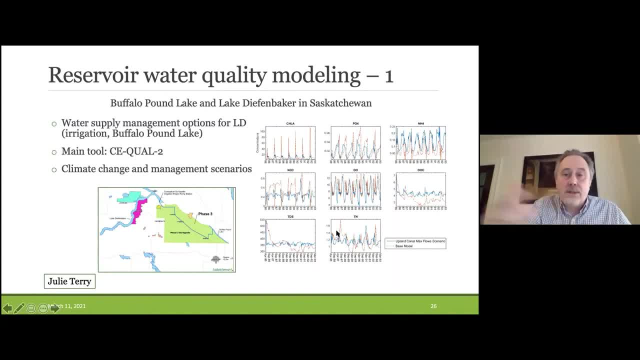 you could think the current situation is compared to one of these water management scenarios and looking at parameters such as chlorophyll, phosphate, ammonia, dissolved organic carbon, dissolved oxygen nitrate, total dissolved solids and TNN, If you just look at the various curves, 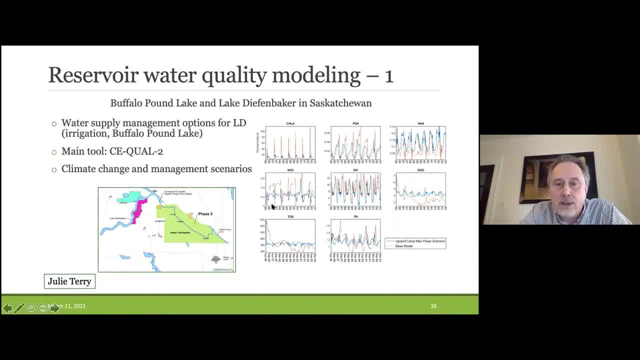 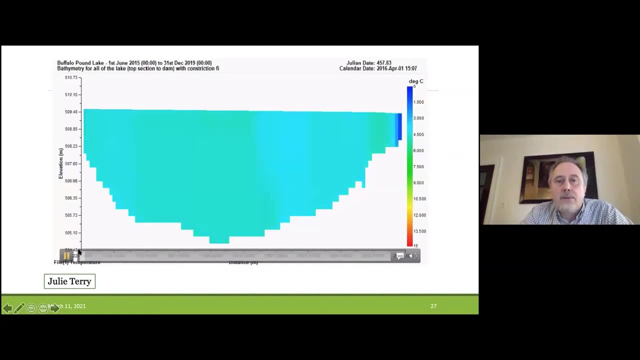 particularly for nitrate. here you see that the large fluctuations in the base scenario are much more attenuated in the proposed, one of the proposed management scenarios. So here is a scenario simulation- I'll start it up right away here- For one of the basins of Buffalo Pound Lake. 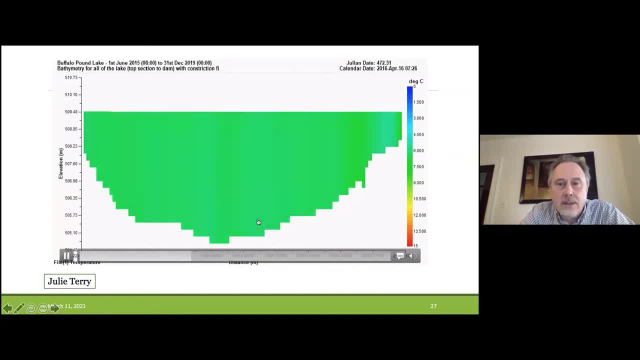 you can see, it's a very shallow lake. So you see that. so it's temperature, the temperature distributions. you see that we have very little vertical stratification in the Pound Lake And what you see is this, these, these events, or these. 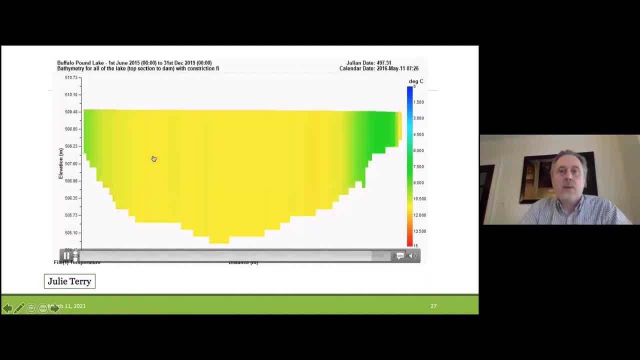 these wind driven stages that basically bounce back and forth from one end of the basin to the other one, keeping it well mixed. So that means that we don't have to worry about, we don't have to worry too much about stratification, thermal stratification in this basin. 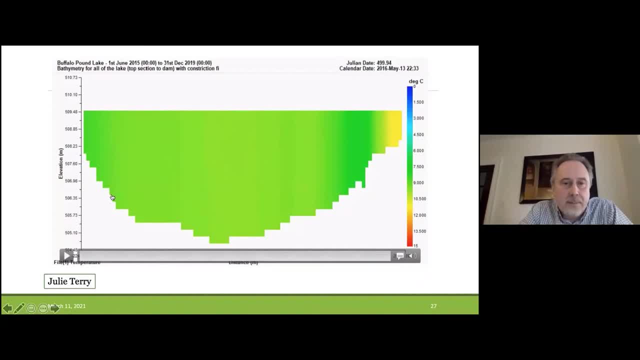 And thermal stratification is often associated with with oxygen depletion in in the lower part of a lake or reservoir And that has a big effect on the internal loading of phosphorus. And yeah, And so that's actually the the. 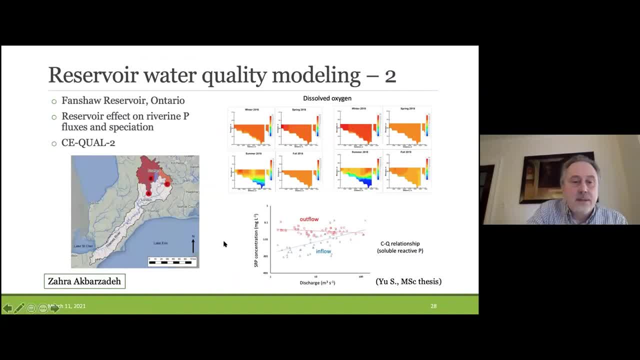 the topic of this second project. It's actually a master's thesis where Zara was providing support. So now we're talking about the, the potential reservoir in Ontario. it's located on the Thames River. Remember that, because I'll continue with the Thames River and Lake St. 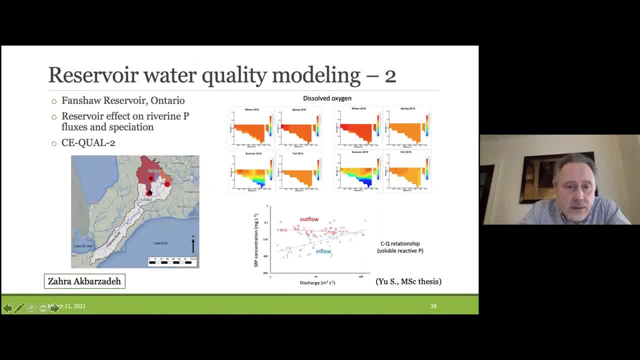 Clair here in a minute And it was specifically to look to eventualize the little Reservoir A here And it was to look at the reservoir effect on riverine phosphorus fluxes and speciation using the same modeling platform, SQL2.. 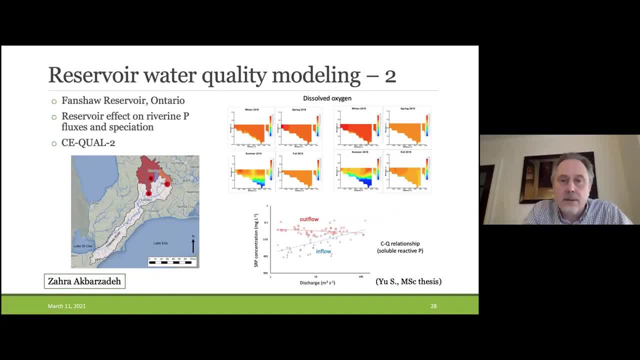 So here we used extensive data sets that were collected by another of our students over 2018 to 2019.. We use the 2018 data to calibrate the model and then 2019 to validate it, And what I want to point out is that during the summer months, 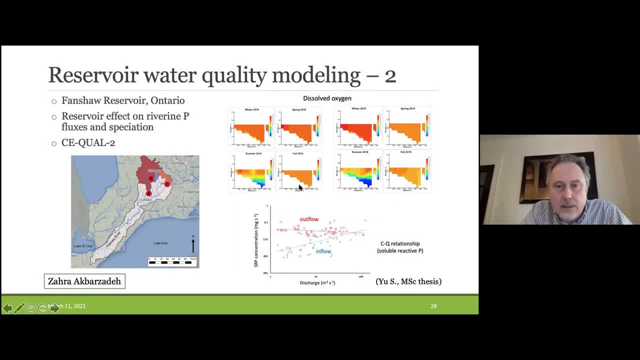 both in both years- in 2018, but even more extensively in 2019,- we had stratification of the deeper part of the reservoir, So that's the part close to the dam, And so depletion of oxygen, which activates internal phosphorus loading. 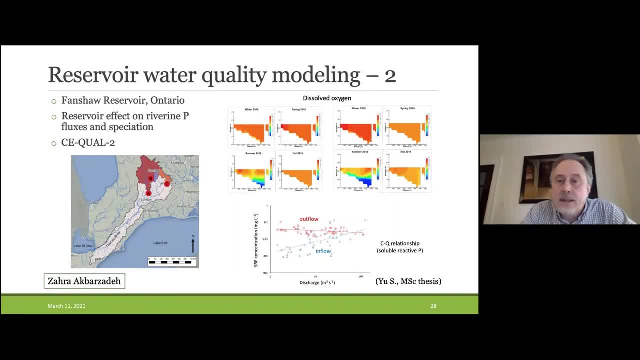 So during the summer the reservoir actually acts as a net source of phosphorus to the downstream river. So that's the same river reach, So the the Thames River, while overall, integrated of the entire year, the reservoir actually retains as net retention of phosphorus. 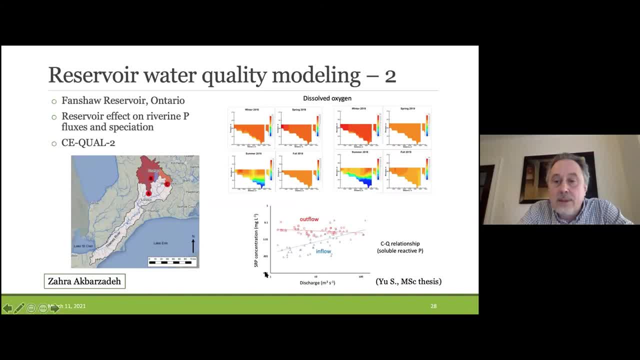 And if you look at the lower graph here what it shows. So here again it's one of these CQ relationships, So the concentration versus discharge relationship. this is often used as a signature of the river and is usually interpreted in terms of the 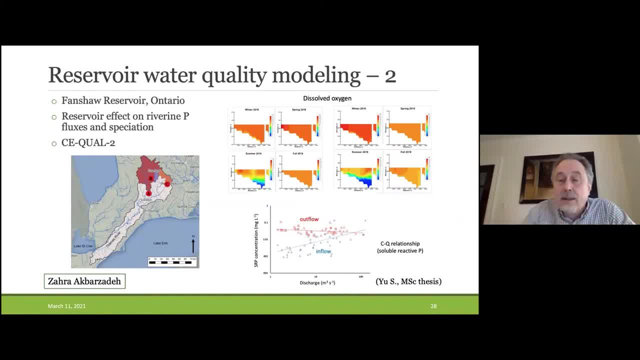 the sources of whatever constituent you're interested in, And then the transport pathways from those sources to the river. Now, if you look at the inflow- so this is the river coming in upstream of the reservoir- you have this positive correlation between the concentration of. 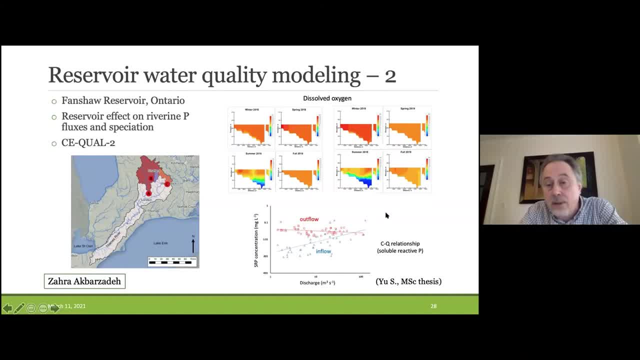 soluble, reactive phosphorus and discharge. So this would be called an enrichment trend. But if you do the same with the measurements in the outflow- in fact these are all model, model derived concentrations- You see that the the relationship has completely changed. 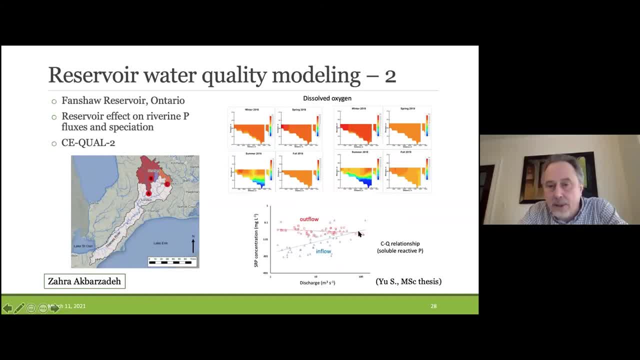 And in fact it's more of a chemo static relationship. So, but rather than saying something or indicating a change in sources of flow paths, essentially this change in the CQ relationship is a signature of the processing of phosphorus in the reservoir. 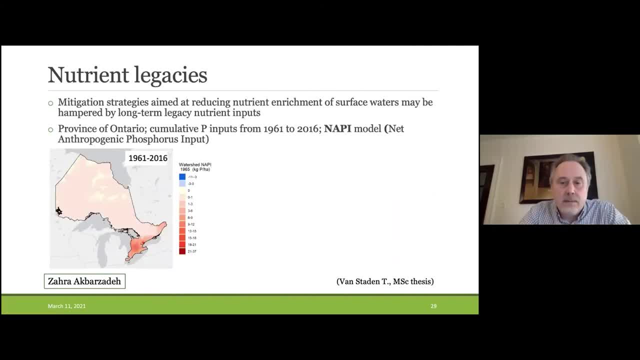 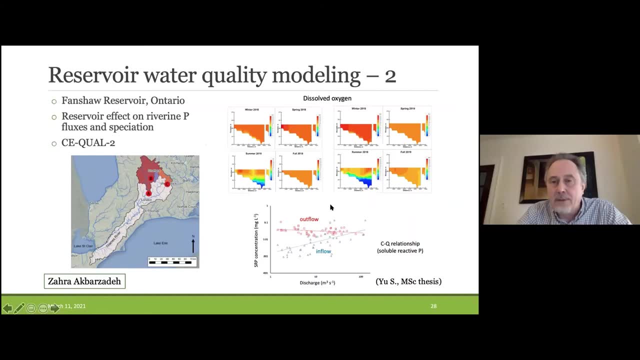 All right, So that's actually brings me If I go back for a second. So, as I said, the reservoir here, on an annual basis is will retain phosphorus, So phosphorus is accumulating in the reservoir. So this is an example of a legacy that is building up in. 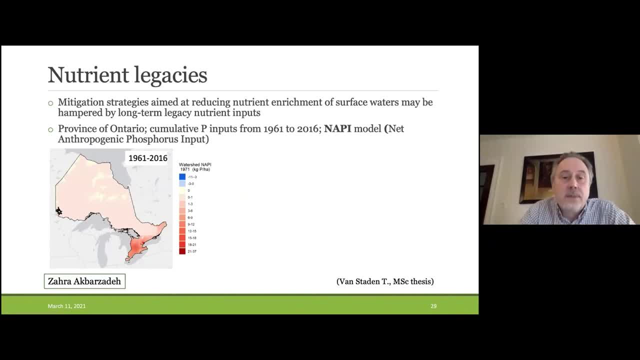 in this case the stream, but nutrient legacies also build up in in the landscape, or in the, in the- yeah, in the landscape, And so one of the issues that is being addressed, particularly in the in the research group of Nandita, is how mitigation strategies aimed at 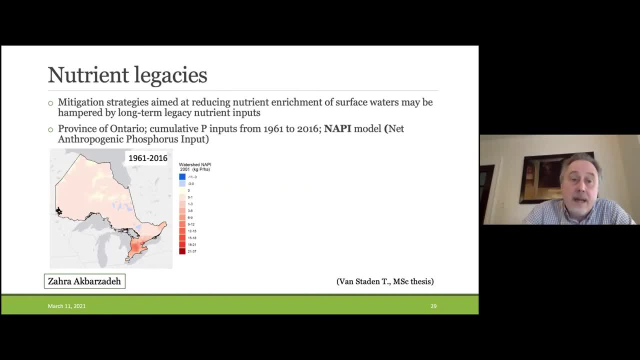 reducing nutrient emission, surface waters might be hampered by long-term legacy nutrient inputs. So these legacy nutrient inputs are essentially what is remaining in the landscape over historical time and is slowly released Then back to the, to the groundwater or ultimately to to the river system. 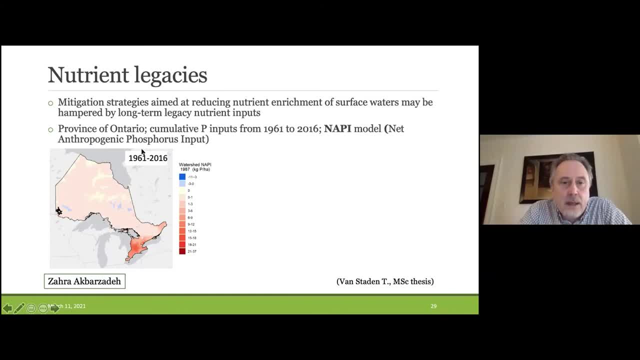 And so in this project, also supported by by Zara, was an assessment for for the entire province of Ontario, of the cumulative phosphorus inputs from 1961 to 2016.. And if you look here, at the graph here, and you see this little counter here, 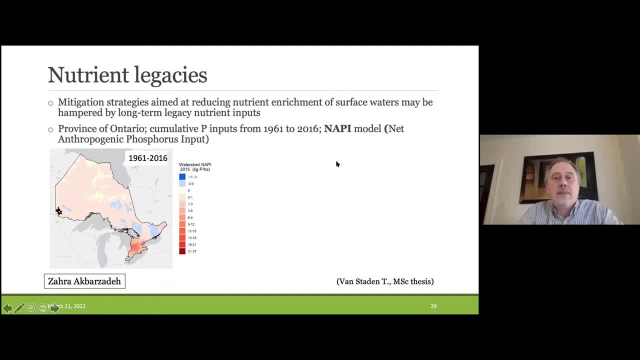 So so what you're seeing here is, year by year, the what's called a net anthropogenic phosphorus inputs over distributed over the entire province of Ontario, And, of course, one of the things you see is we have this hotspot of nutrient. 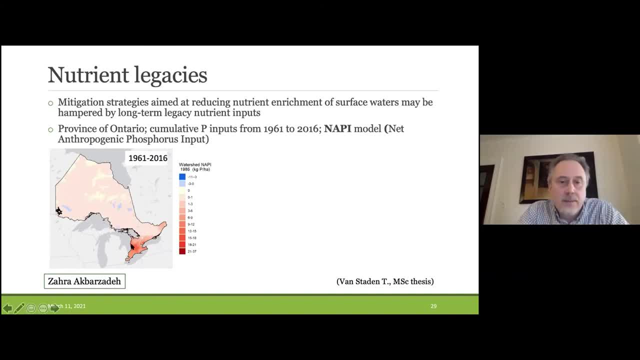 inputs in the Southern part of Ontario, because that's where all the agriculture is taking place And that's where all most of the people in Ontario are living. So the results of that, of course, is that these largest inputs of phosphorus to the landscape or in Southwest 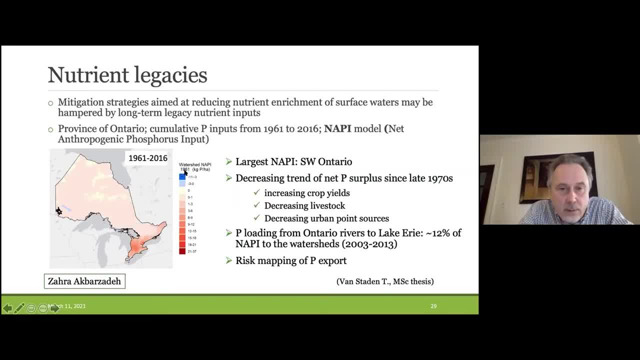 Ontario. we do see that, if you, if you would follow this how you started: 64,, 65, see the colors as you are getting redder and redder. So from the sixties to about the late 1970s. 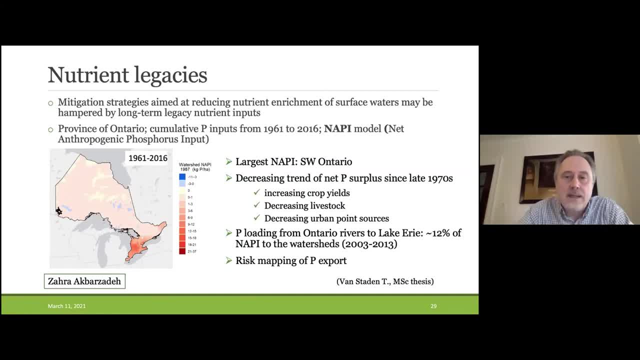 we have, year by year, increasing inputs of phosphorus to the landscape, But since the late 1970s it's actually decreasing because of increasing crop yields, decreasing livestock and decreasing point sources. But if we look now at the, the phosphorus loading from Ontario rivers to Lake area. 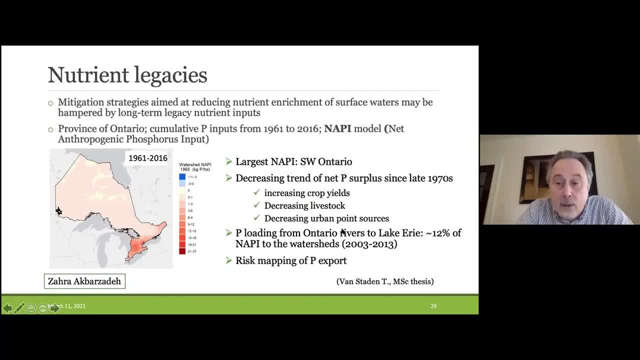 So what is carried by the rivers to the lake? it only represents about 12% of the inputs to the water sheds, So it means that about close to 90% of the phosphorus that is brought into the watersheds and applied as far as 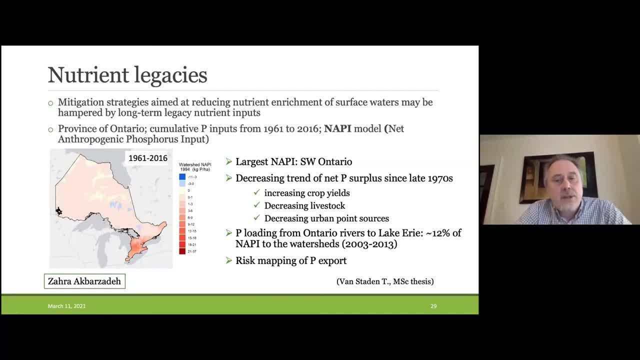 as fertilizers, as sewage, et cetera, actually stays, as is still staying in the watershed. So we're still building up the legacies, And so now we're coupling these spatial distributions of these phosphorus inputs, also to risk mapping of fossil export. 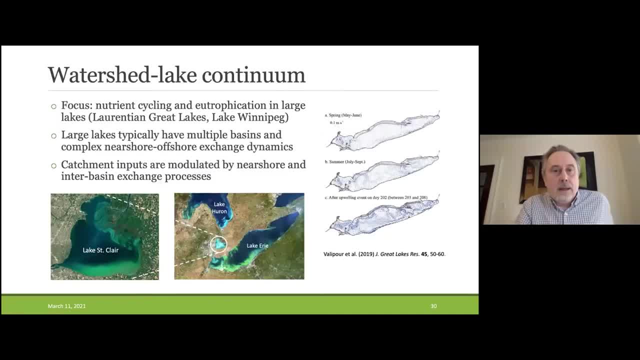 which, of course, also depends on the export pathways. Okay, Now let's look at- let's get closer to the lakes now and look at the watershed to lake continuum And the focus here is really on nutrient cycling and vacation large lakes, the Laurentian great lakes in particular. 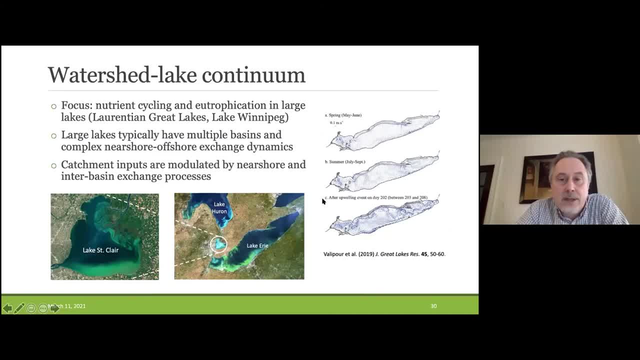 and also starting now in Lake Winnipeg. and large lakes of course have multiple basins. They have complex near shore offshore exchange dynamics and the, the, the river inputs don't directly go to the offshore lake but have to model it also by near shore in the base and exchange. 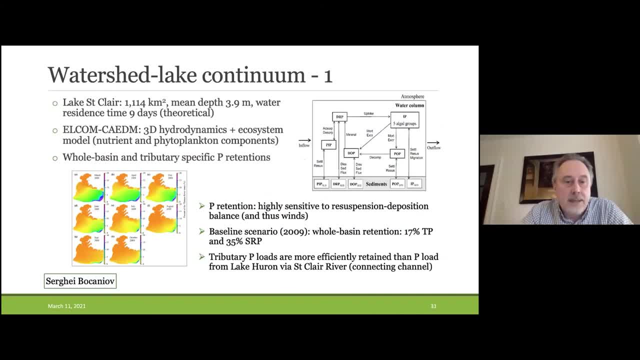 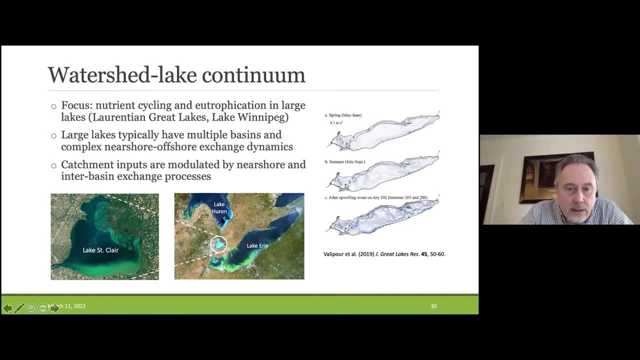 processes. So one project here by by Sergei was looking at Lake Sinclair. If I go back here, Lake Sinclair is over here, So it is actually the connection. It's your Lake Huron. It's connected then to Lake Sinclair, which then connects to the Detroit river, to Lake Erie. 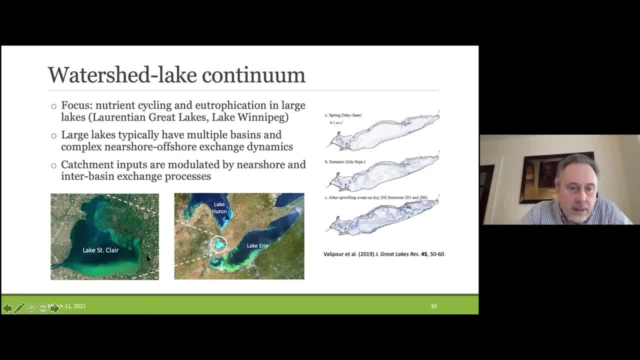 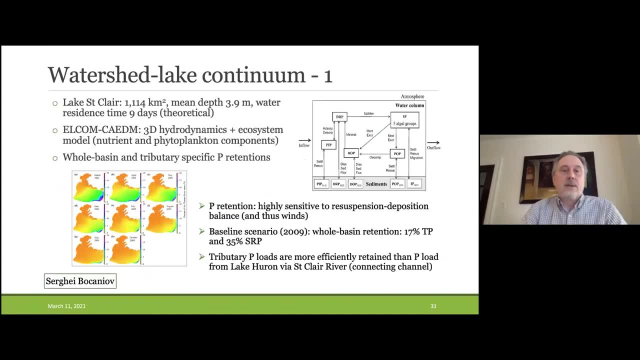 And so the Thames river, which is the largest Canadian tributary to the Lake Erie basin, first enters into lakes, Lake Sinclair. And so what Sergei did was to use the outcome KDM model. So the outcome model does the 3d hydrodynamics in the lake. 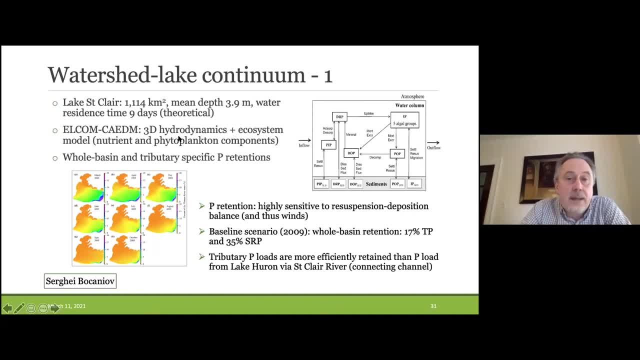 And then the KDM is an ecosystem model, And he particularly used the nutrient and phytoplankton components of that that model. Lake Sinclair itself is fairly shallow. It has a very short residence time, nine days- But what he was able to show and calculate was not only the whole basin, 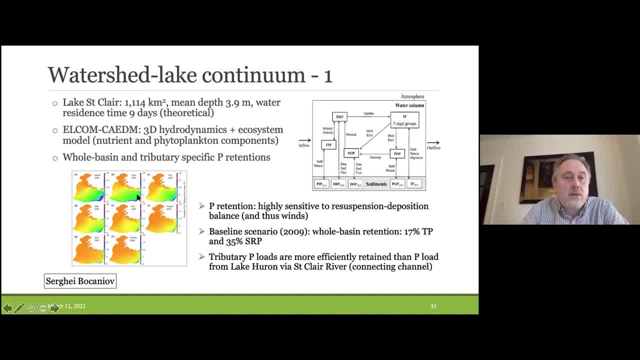 retention of phosphorus In Lake Sinclair. So looking at all the inputs of phosphorus to Lake Sinclair and then what is actually going out To Lake Erie, to the Detroit river, but also look at tributary specific fossil retention And some of his conclusions were that phosphorus attention 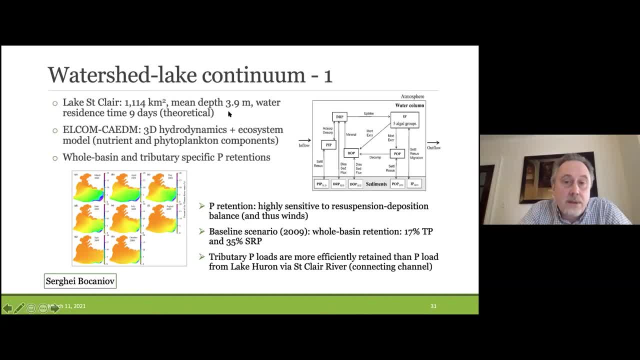 It's highly sensitive to risk, risk suspension, deposition, balance and so on, And so you know it's a very shallow lake, because it's a very shallow lake And just it depends a lot on the winds And that can vary. 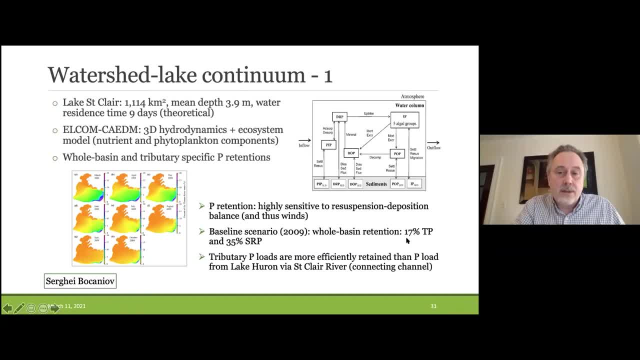 of course, from season to season and from year to year, And in his baseline scenario of 2009,. he found the whole basin retention of 17% of total phosphorus and 35% of Solvable reactive phosphorus, But the tributary loads 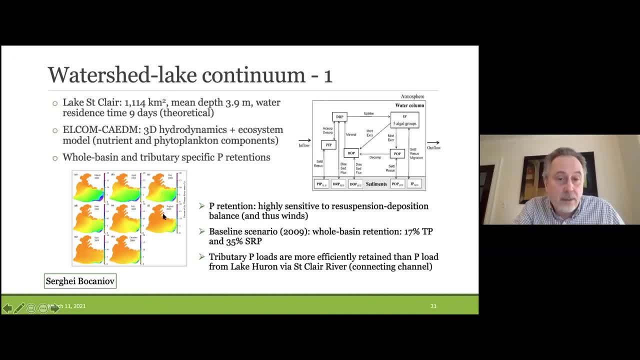 So the loads that are not coming from Lake urine, Those are actually more efficiently retained than the fossils load That is coming from from the curing. So in other words, in that you can see on this graph here, you see the, the color here. 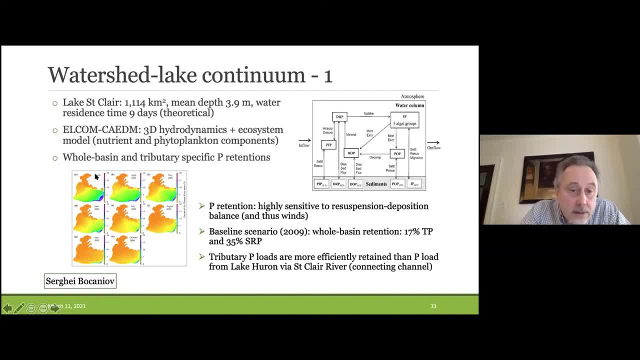 the blue color, the red color, the yellow color, the green color, the yellow color, the blue color, the blue color. These different colors Indicate different percentages of water That is actually delivered from the Thames river, So you can actually follow the phosphorus molecule. 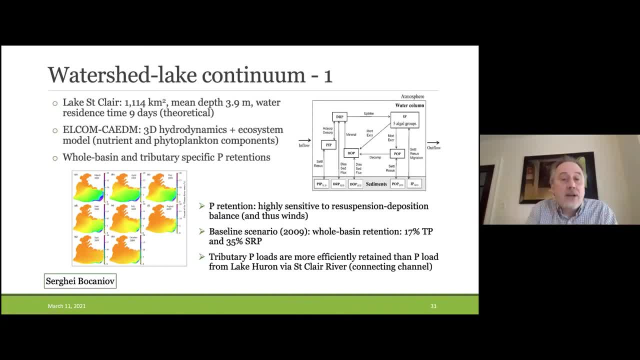 the phosphorus atoms that are coming from the, from the Thames river, from the other tributaries, from Lake urine, and essentially see how many of the fosters Atoms delivered by Actually make it out to Lake Gary. And so we can. 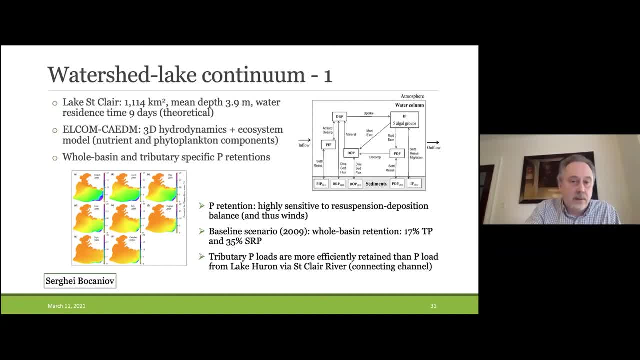 you can really do this, So this gives you a very, very detailed picture of what happens. And so you can, you can really do this, So this gives you a very, very detailed picture of what happens. So, so so. 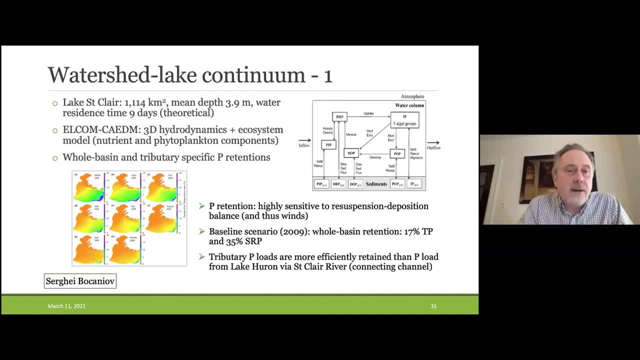 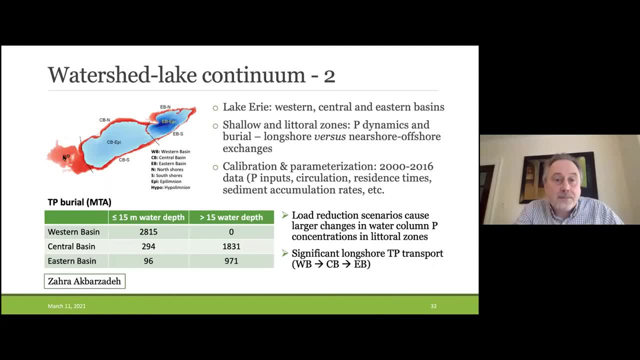 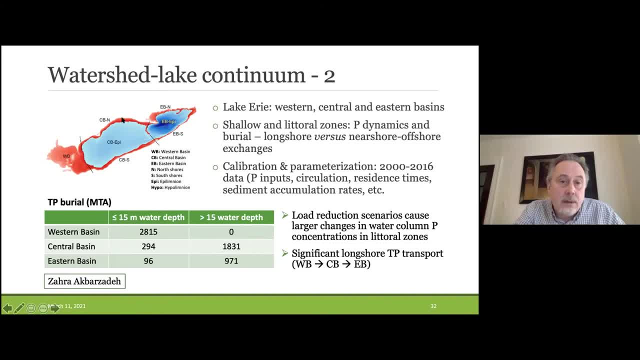 Now look at a role of the near shows zones, And so the zones that you see, or the red color here In a photo, Is the is the area that is up water depths- none shown- 15. Meters, And of course the whole Western basin, is a very shallow basis. 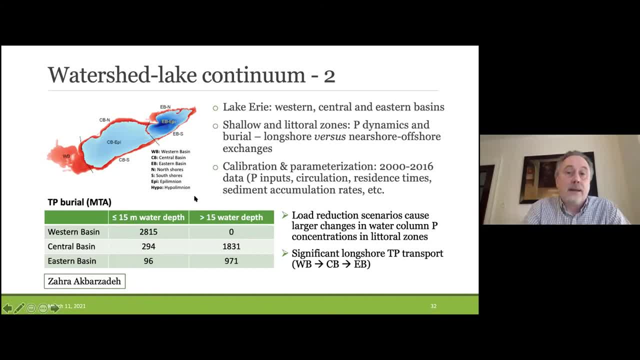 And so there's an 50 units. And then to try to estimate projetes, Then how these literal zones Can, how these literal zones is the retention of phosphorus in the literal zone, but also how do they serve as, uh, how are? 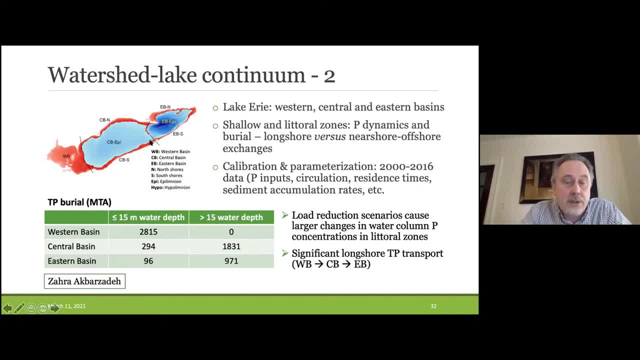 they involved in interchange, uh um interchange, uh interbasin exchanges. sorry and so for this is a much longer time scale than the, the previous uh project, so it takes data from 2000 to 2016 to calibrate and parameterize the model, and some of the big conclusions are the load reduction. 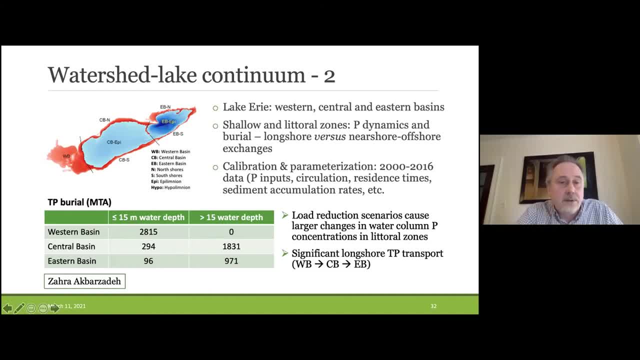 scenarios cause larger change in water column phosphorus concentration in literal zone. so if we reduce the riverine inputs of phosphorus to the lake, the, the biggest effect will actually be in these literal zones and in the western basin, less so in the large offshore zones of. 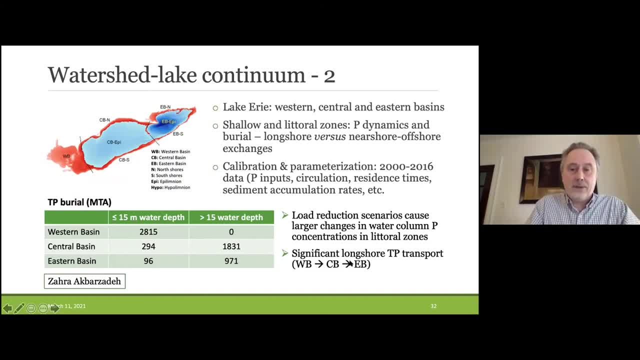 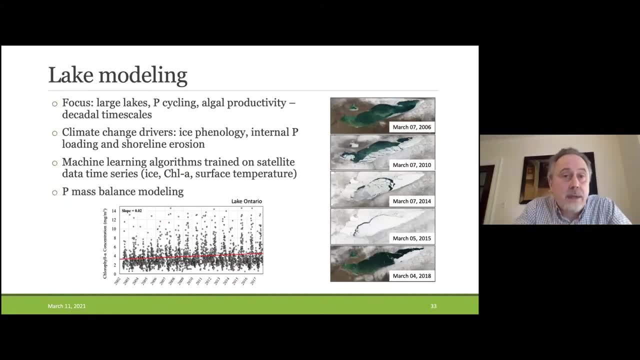 the central and western basin, but it also shows that there was very significant long short total phosphorus transport. now, if we go now to the lake modeling- and so i have a couple more slides here- so again the focus on large lakes and phosphorus cycle, on all the productivity. 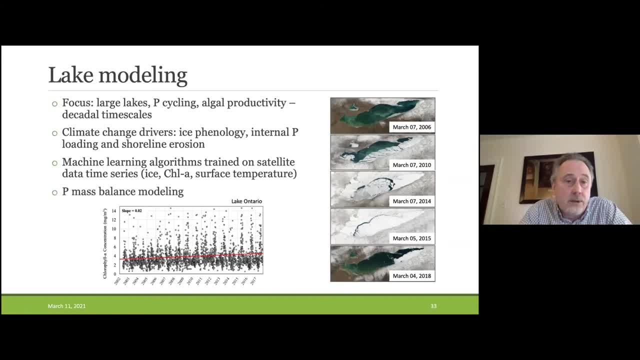 but also particularly on climate change drivers, ice phenology, internal phosphorus loading and shoreline erosion. We've been using also machine learning techniques to develop algorithms that are trained on satellite data time series like ice phenology, chlorophyll a and surface temperature. 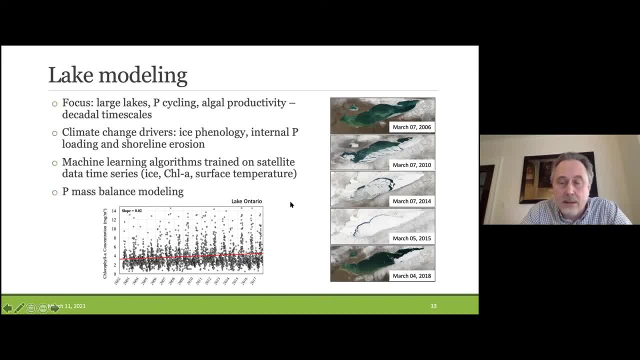 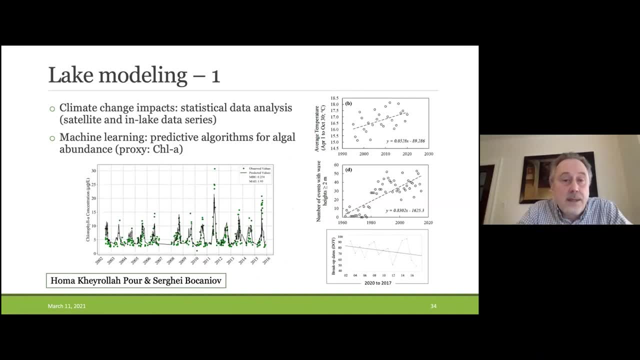 And then the last project I'll show is on phosphorus: mass balance modeling. So climate change, so a lot of statistical analysis of time series data which all showed that indeed we have these trends that are indicative of climate warming. So increase in surface water temperatures. 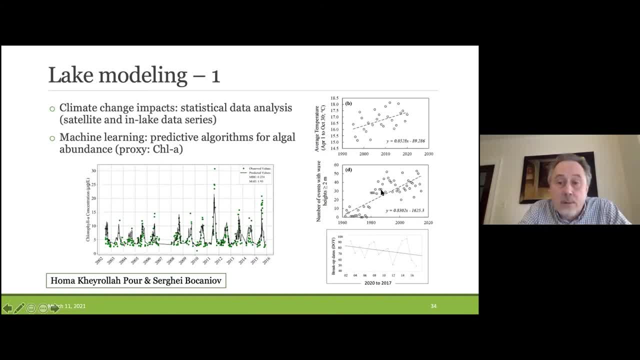 also increase in the number of large storm events and a decrease in ice coverage And so kind of. using this type of data, we can then train algorithms to machine learning techniques to essentially produce predictive relationships. in this particular case, you can see for chlorophyll a. 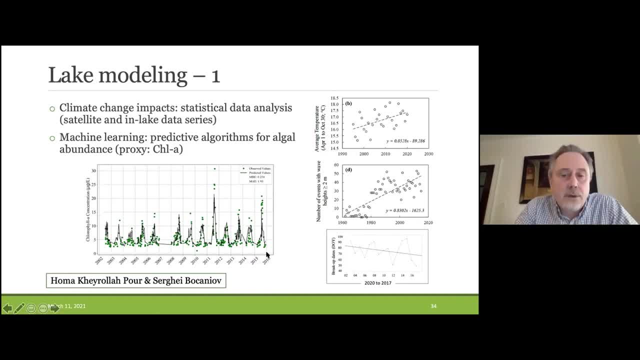 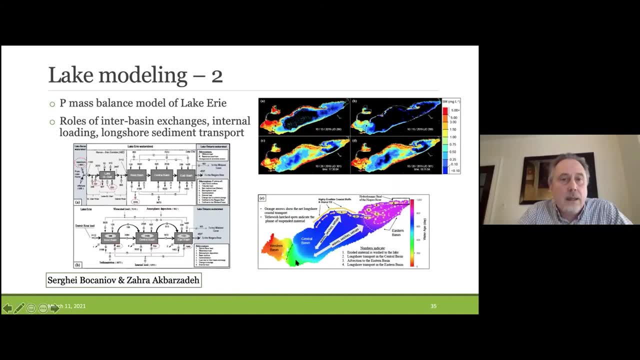 And so those type of predictions are then coming closer to the operational predictions of, for instance, all the blooms, like the ones that you see here in 2011.. Then, finally, the phosphorus mass balance modeling for Lake Erie. So this work- and again I'm sorry, this is very small- 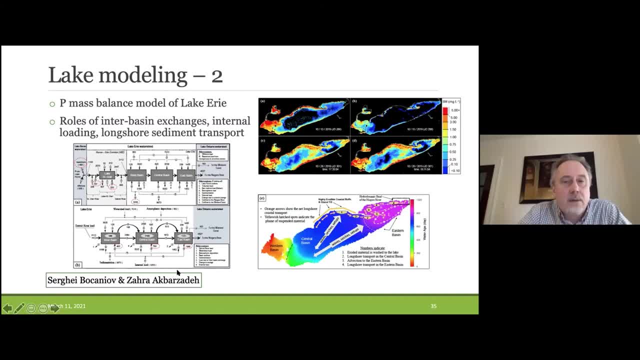 But it really shows- so this is a complete reanalysis of previous estimates- And it really emphasizes the role of interbasin exchanges in terms of understanding how phosphorus is being redistributed in Lake Erie. So, again, this is a complete reanalysis of previous estimates. 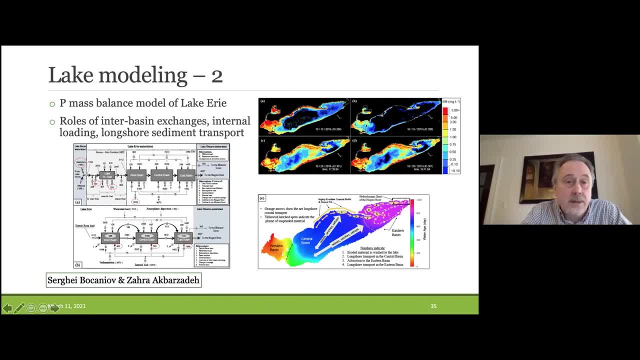 We have the Western Basin, the Central Basin and the Eastern Basin. It also is so very much long shore sediment transport, but also the importance of increasing shoreline erosion as a mechanism to remobilize phosphorus inside the lake. And in fact, if you look at the satellite pictures here, 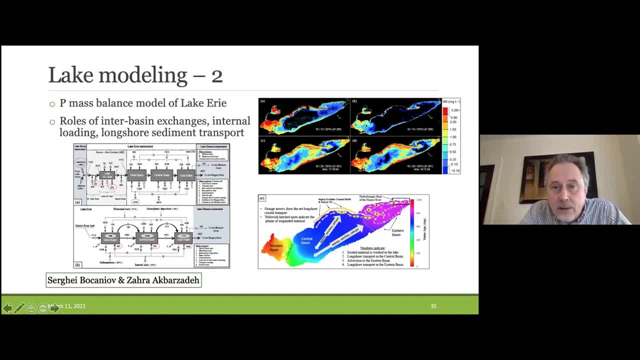 you see this suspended matter along the northern shore, for instance, of the central basin, And you see the extents down into the upper river, the eastern basin, and actually this is. we now propose a major mechanism of total phosphorus transport that is actually increasing because of climate warming induced increases in storm. 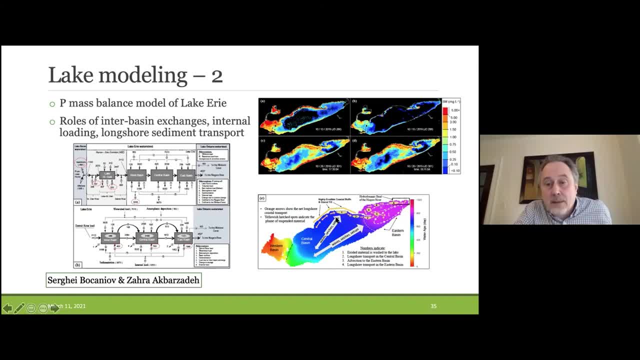 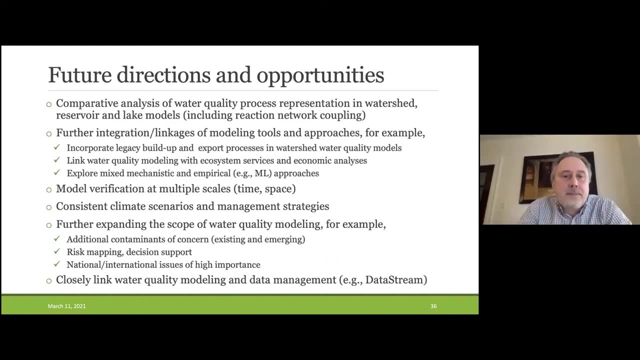 activity that remobilizes suspended matter to shoreline erosion and then pushes it into from one basin to the other basin. all right, so maybe to conclude, some some thoughts about future directions, opportunities. uh, i think that it's now a good time to look at the various models that we're using, uh, for instance, for nutrients, to do a comparative analysis of how. 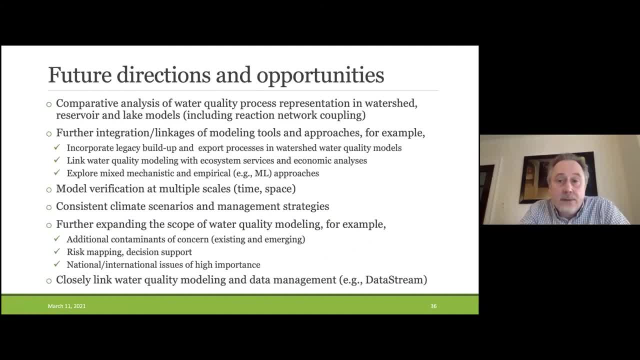 these water quality process process are represented in these different uh models, whether it's in watershed, reservoir or lake models. and also, looking particularly us, to what degree are some of these reaction networks accounting for the coupling between various water quality parameters? there's scope for further integration, linkages of modeling tools and approaches, for instance: 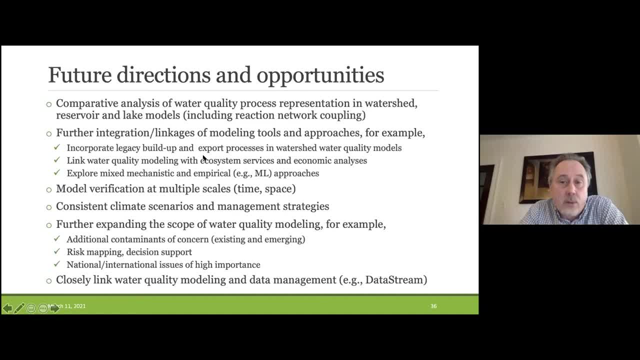 incorporate legacy build up and export processes in watershed water quality models, so explicitly taking into account that we had historical buildup of legacies that are now still influencing uh export from the landscape to river systems and ultimately to reservoirs and lakes. linking water quality modeling with ecosystem services or the provision of ecosystem services. 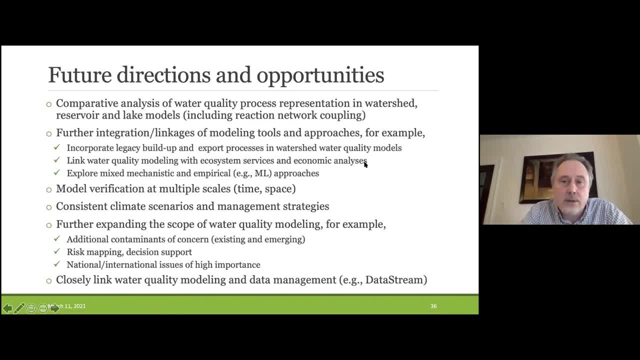 and economic analysis, such as ecosystem services valuation or cost benefit analysis, uh related to infrastructure. cinco um um ways to key will longer time scale if you go to decadal time scales, particularly if we start thinking about looking at climate scenarios or projected climate change, so maybe also develop within the group. but 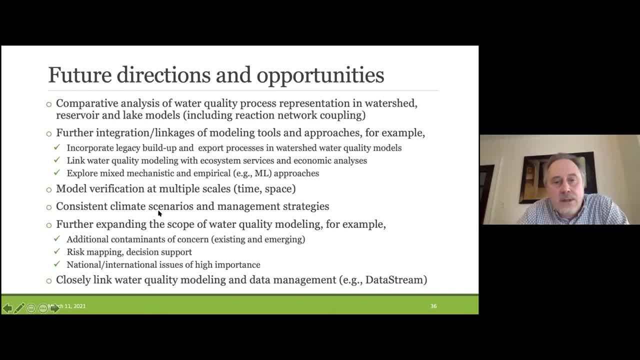 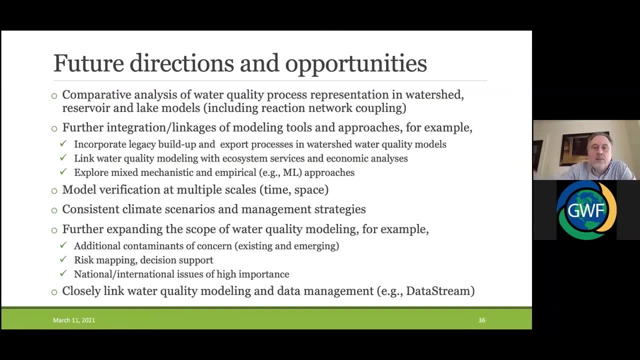 also in collaboration with other GWF researchers, consistent climate scenarios so that we're all kind of looking forward over the same type of time scales or important time points in the future, and then also in terms of management strategies, we can of course further expand the scope of water. 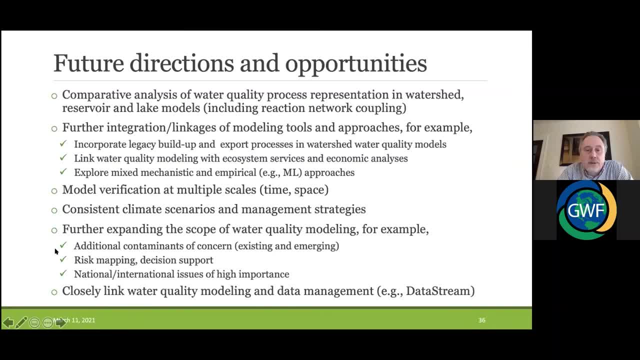 quality modeling by looking also at additional contaminants of concern, both existing and emerging, to go further into risk mapping and decision support and uncertainty analysis and then really start addressing also other national, international issues of high importance. of course, given the size of the water quality modeling group, we have to be, of course, strategic. 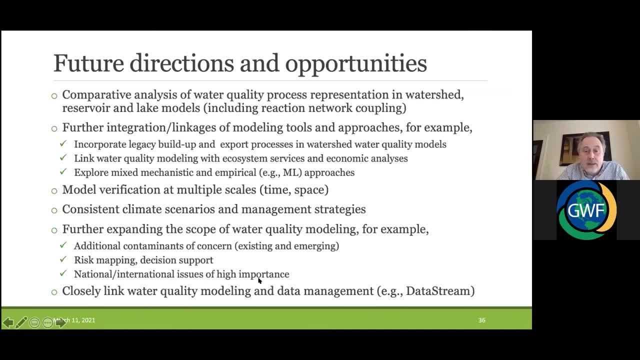 we can't do everything. so I think we really need to start thinking about how to highlight the importance of this work also to look at issues that are clearly of large interest or a broad interest, and then more closely link also water quality modeling and data management, for instance. we're 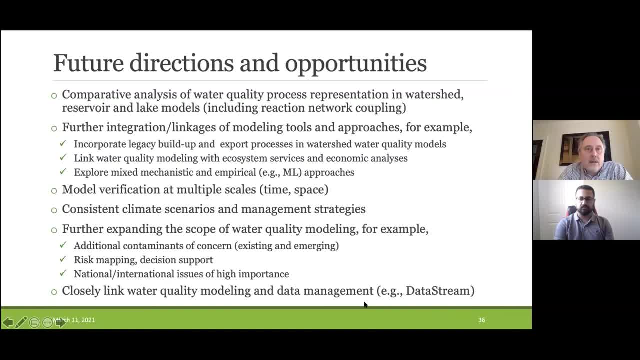 working now with data stream to see how we can better manage and curate and use water quality data, and with that I'd like to thank everybody who participated in the webinar and particularly many, many thanks to all our postdocs and research associates in the water quality. 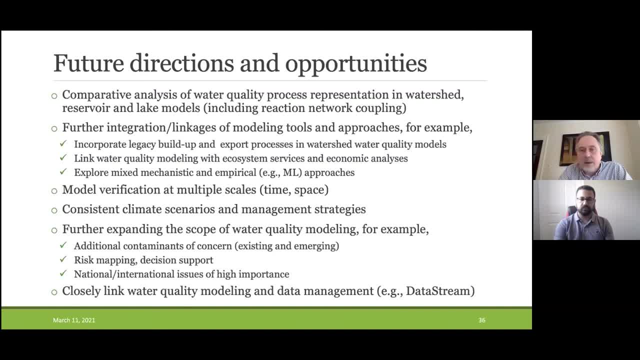 core modeling group who essentially did all the work. so thank you very much, and I'm open to questions also. some of the more technical questions probably will then be directed- or are better directed, to the, the actual core modelers themselves. thank you. thank you, Philip. it was a fantastic and very informative presentation. I will be now moving. 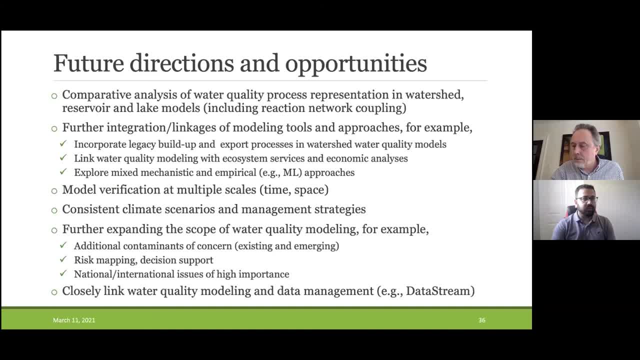 towards a Q&A session. we have one question. it's anonymous question, so the question is: all these research are very great research, but how is that research being applied to improve the water quality in this area that is being studied, so how you know how the research is. 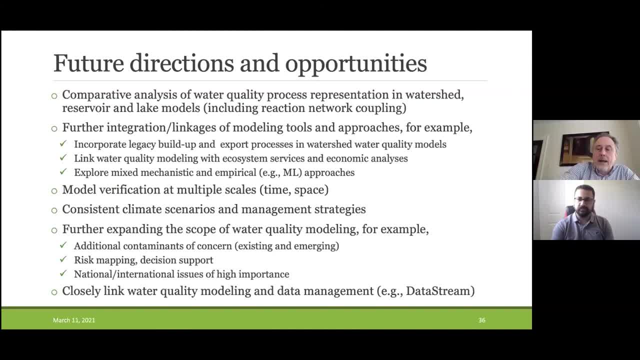 actually being translated into the practice. for instance, I showed the example of the work of Julie Terry in Buffalo Pound lake. that has very direct implications for which management options will be implemented in the future. at least, we hope that that will be in terms of of water quality improvements. for instance, the work that I showed on metal. 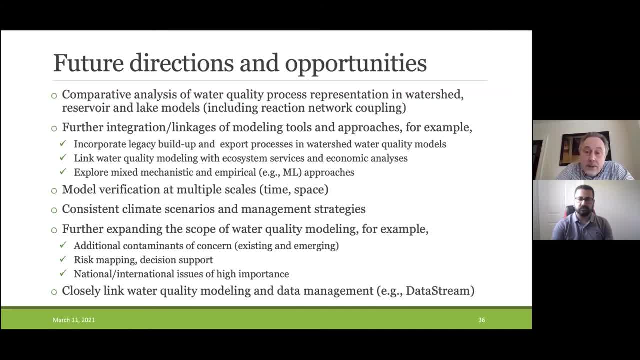 distributions in the Dunn valley is actually being considered or is actually helping directing some of the dredging work in the in the river, because we've been able to identify where the metals are accumulating. that's not that much important, so important for the Dunn river itself. it's more. 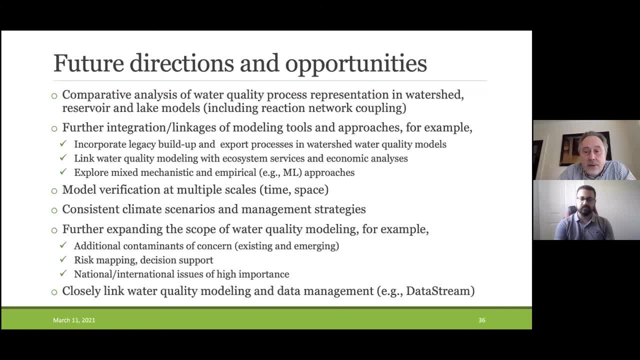 important for the Toronto harbour, which the international joint commission has identified as an area of concern with the water quality in the Dunn valley, and I think that's a very good point. I think that's a very good point, and I think that's a very good point, and I think that's a very good point. 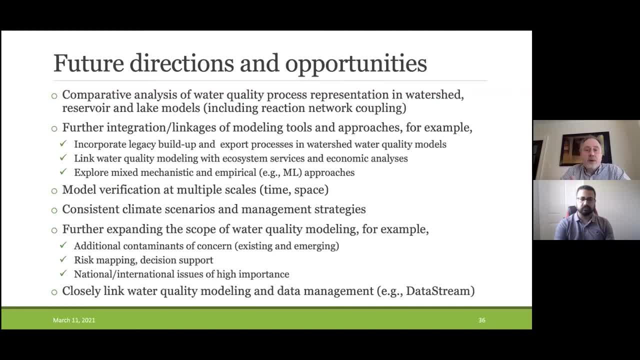 within the Great Lakes and so it's essentially preventing these metals from entering them, that environment. in terms of the lake work, we're, for instance, looking at assessing essentially the potential impact of the proposed reduction in phosphorus loading to Lake Erie by 40%, for instance. what we were able to show, for instance, is that, because if you reduce 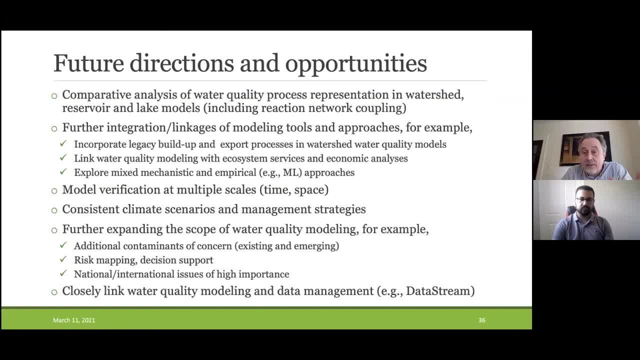 the input of phosphorus from the tributaries to Lake St Clair by 40%. it actually doesn't translate in a 40% reduction in the total phosphorus that is going from Lake St Clair to the western lake, western basin of Lake Erie, because most of the phosphorus load actually comes from Lake Huron. 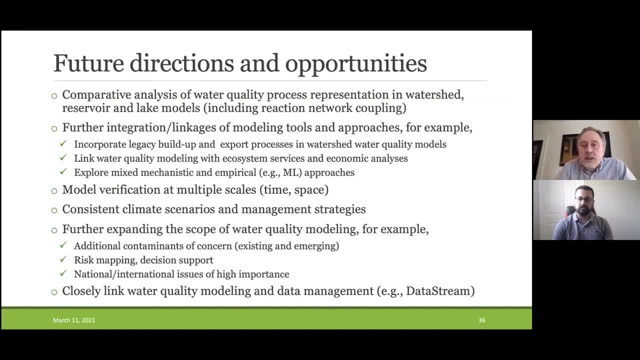 so I think we it's there's, there's different ways in which we can connect with, of course, practice and also with, with essentially informing policy decisions. so it's not that each project has necessarily the same kind of goal in terms of: hey, I want to improve water quality. 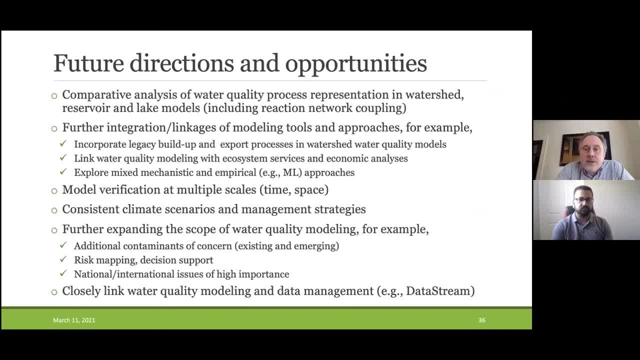 and it's also it depends on the, on the, on the stakeholders. for instance, the sediment transport work in in in the South Saskatchewan river basin is quite it's as important in terms of hydropower production or hydropower production potential also in other watersheds and what it. 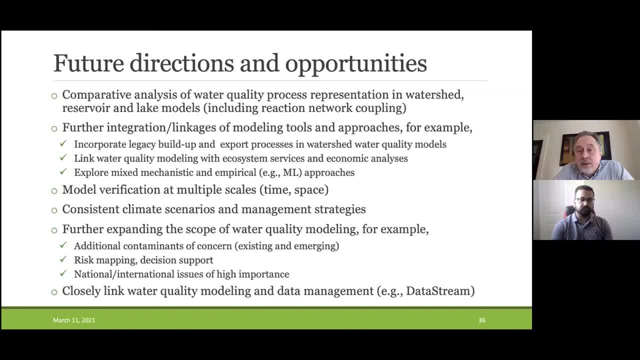 does in terms of starvation in the downstream delta areas. so i think what we're, what we're doing, is mainly connecting, connecting the dots and, as i say here in my last slide, of course we also, we have to also integrate the different parts of the modeling, but ultimately we also are a kind of a service. 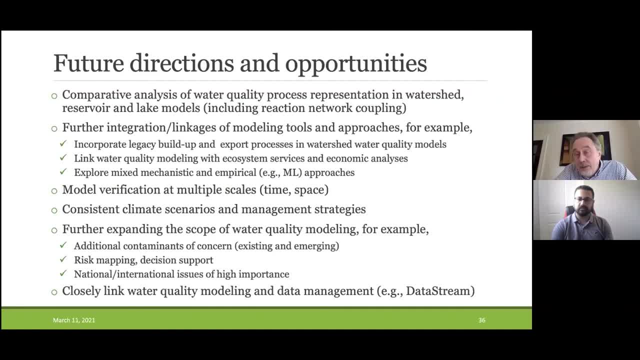 oriented group. so if other projects that have specific end users that want to basically contribute to water quality improvement, they can come to us with specific questions and we can help them develop or apply the necessary modeling tools to help them, even if they don't have that modeling. 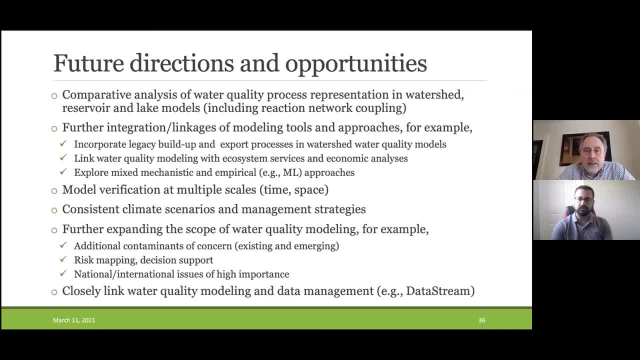 capability within their own, their own group. so so, essentially, that's that's my main message to anyone who says, hey, well, i have a water quality issue, but maybe i want to know which model to use. well, you've seen the comparative analysis of water quality models that already can direct you to the 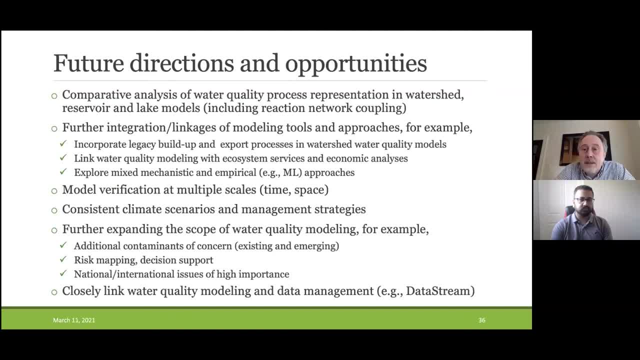 water quality models that already can direct you to the water quality models that already can direct you to the right model to use, and then we might have the expertise in-house to help you implement that particular model in your particular case study. i think we are already one minute past the hour mark, so there's two more questions i'll try to. 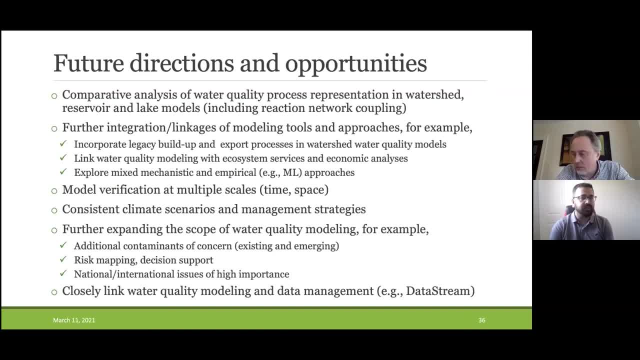 frame them in from them in one question and maybe you can quickly address that. so it's from muhammad riaz and he's wondering if there's any modeling video tutorials, you know, for the prospective uh learners to learn, and you know if, what, what types of programming skills are needed to require these models? 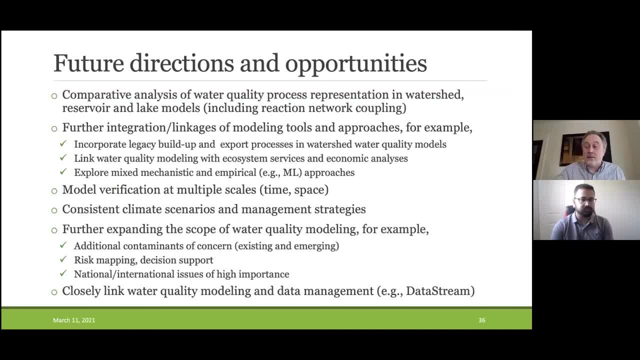 ah, well, it really depends on on which model, because we go from very simple models to very complex models. so, uh, we don't have tutorials as such. most of the existing models, like the, whether you have the, the wasp model or the, uh, the swim model, all those have actually 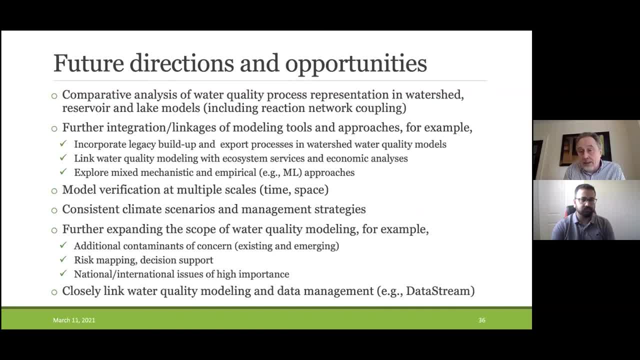 fairly well developed tutorials that you can access online or they also have manuals that go for it. so mostly what we can do is help you find the manuals. that would be necessary. a lot of these, these models of the shelf models. you don't need to have any programming coding experience. you can use them as a user because the coding has already. 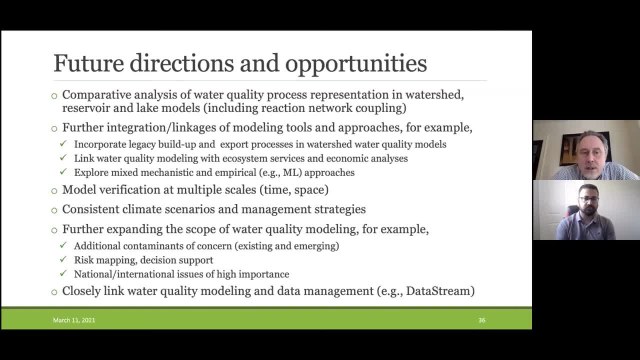 been done, but i would, i would strongly encourage, just to uh, to start a conversation with the modeling group, with a specific person or several persons, and just kind of see what the scope of your of the issue is, or the the system that you are interested in, what kind of, because it often depends on things like it's not just i want to model as i start in. 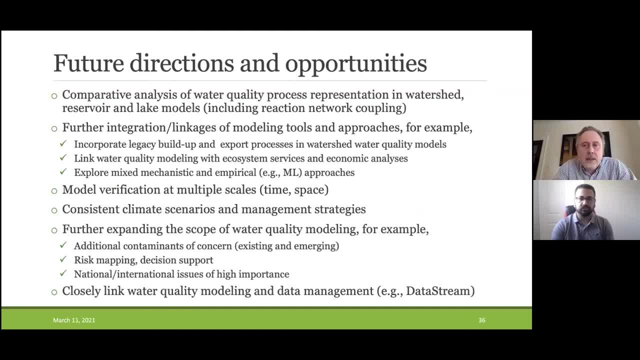 the beginning. water quality means different things to different people. uh, it also depends on what kind of time scales are you interested in. do you want to do something? do you want to understand things on the seasonal time scale, on the decayal time scale? all this will depend will, kind of. 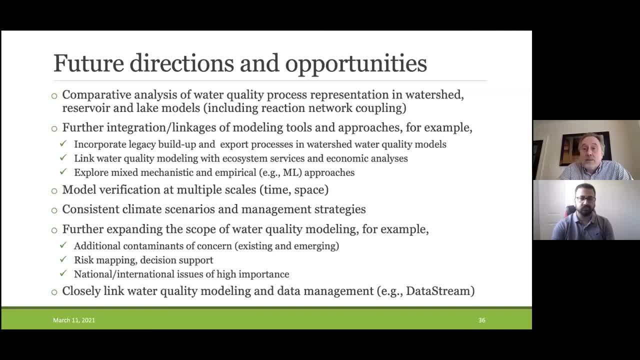 determine which kind of the best model to use is, but, as i said, there is not a single unique water quality model. that simply doesn't exist, and there's also no, no real reason for such a model to exist. um, but it really depends on the question. so you can contact me, you can contact prabin. so 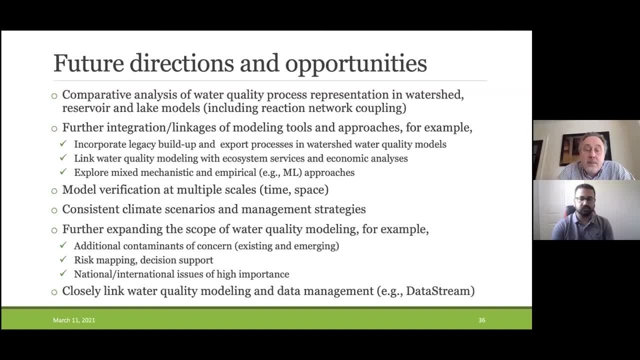 that he can start, uh, finding out who would be the best person to talk to. we can also help train students, for instance, in certain modeling capabilities. so i would say, yeah, let's be flexible, but the best is to to start talking. um, there's a few questions, but i would like to stop here and ask the attendees to email us with. 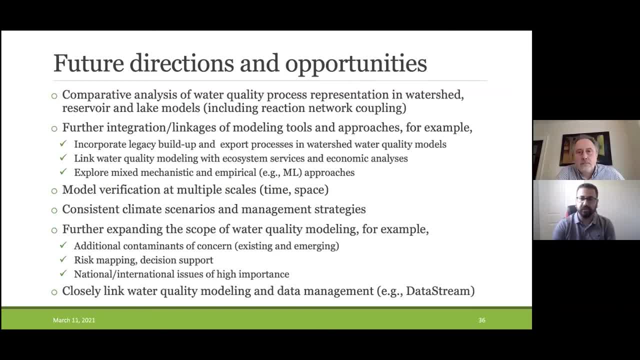 the question and if you can email directly to philip or to me, and then i will pass it to philip. uh, thank you again, philip. uh, i also want to thank everyone who attended this webinar and just a reminder that in next month, on first of all, phil will be having professor al petronero. 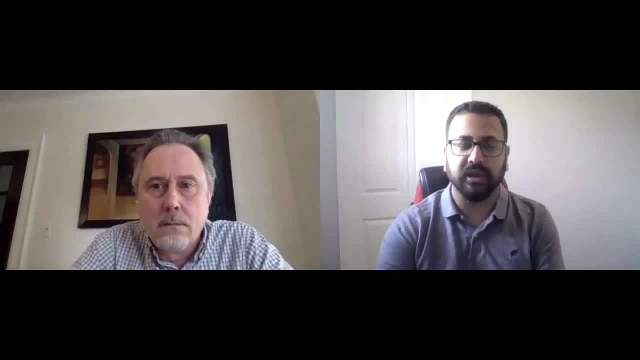 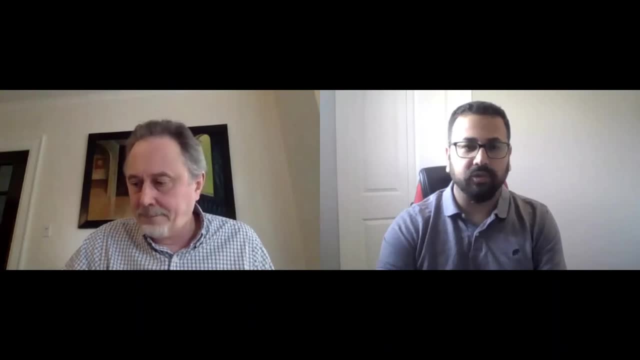 from the university of calgary, who will be presenting on advances in hydrological forecasting. so please stay tuned. uh, that will be all for today. uh, thank you everyone. uh, any last comment from you, philip? no, thank you, it was. um, it was a good experience for myself just to assemble all the, all the. 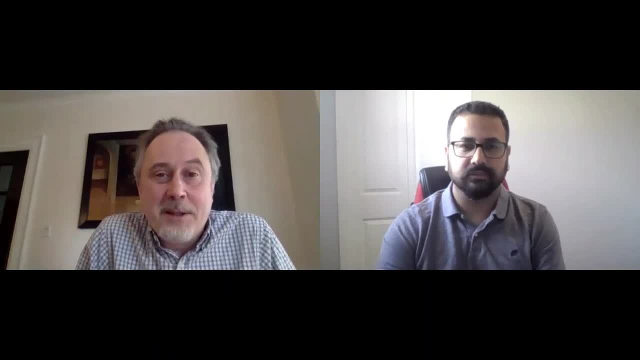 different projects and really very impressed by what our postdocs and our core modeling group has been able to achieve in a relatively short amount of time and with a small, relatively small small group. so i look forward to working- continue working with all of you all, right? yeah, thanks again everyone. i wish you a good day, bye, bye. 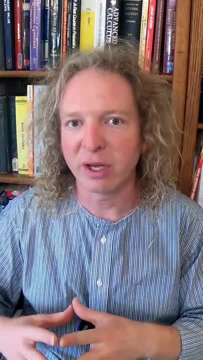 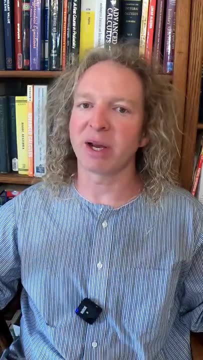 So there's this really really good book for writing proofs. It's called The Book of Proof, or Book of Proof, and it's written by Richard Hemmick And if you just go on the internet right now and you search for it, you can find it, And it's a good book because it has so 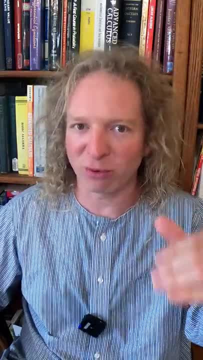 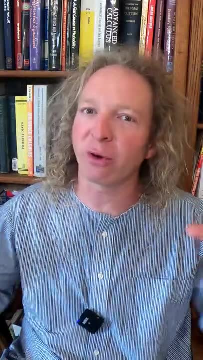 many different subjects in it and it shows you how to write the proofs in all of those various subjects. Now, some parts of the book are better than others. I've pretty much gone over the whole book. I haven't read it all, but I've looked through most of it And I 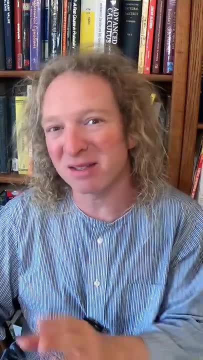 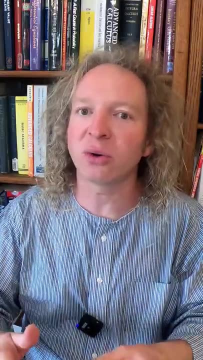 do think it is probably one of the better, if not the best, proof writing book out there. And the best part is it's free right. Anyone in the world can go online. you can go on Google and just type in Book of Proof And it's not perfect. but no math book is perfect.